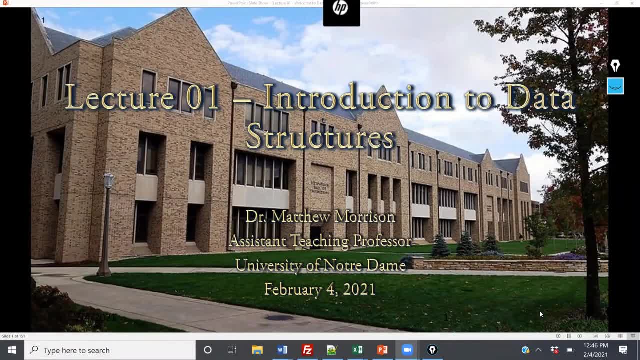 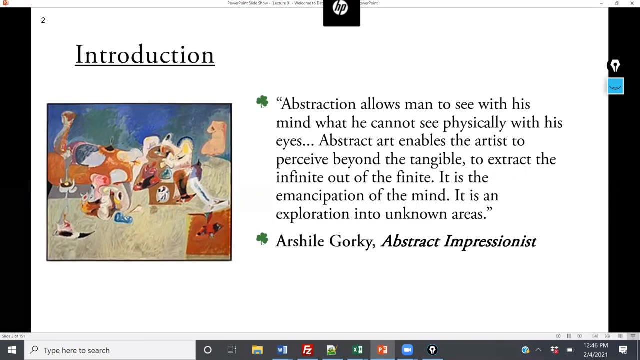 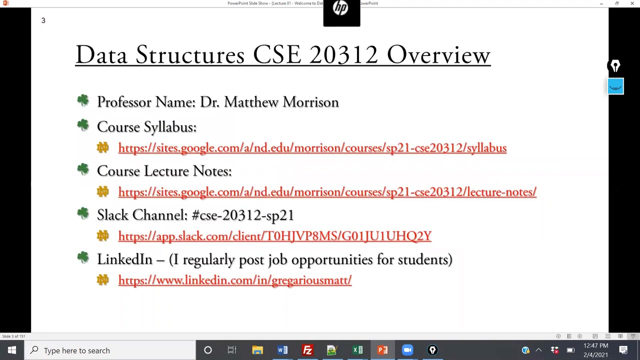 So the first thing I want to do to start the course is to go over fundamental things, things from the syllabus, expectations, tips about how to do well in this class, and make a couple announcements regarding the lab sections. So the first thing, let me do this all right there we go is i want to share a quote that's going to motivate the first of first couple of weeks of the semester and it's a quote from ashile orkey who's actually an abstract impressionist and he says that abstract allows man to see with his mind when he cannot physically see with his eyes abstract art enables the artist to perceive beyond the tangible to extract the infinite out of the finite it is the emancipation of the mind is an exploration into unknown areas the reason i share this is because in order to really master and understand data structures we're going to i'm going to hear me discuss this idea of levels of abstraction up to this point you talked to dr блualand's uh fundamentals computing course or my introduction to computing for c and c plus you learned a little bit about memory management and 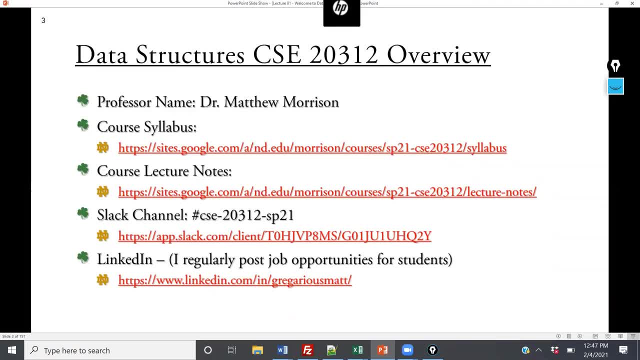 you learned a little bit about memory management and you learned a little bit about memory management about C. You may have worked with pointers, although it's not it's perfectly fine if some of you are frustrated and didn't understand what a pointer actually is. What we're going to spend the first couple of weeks of the semester doing is we're going to dig deep into what a pointer actually is because it's the fundamental to everything that you're coding in C and C++. 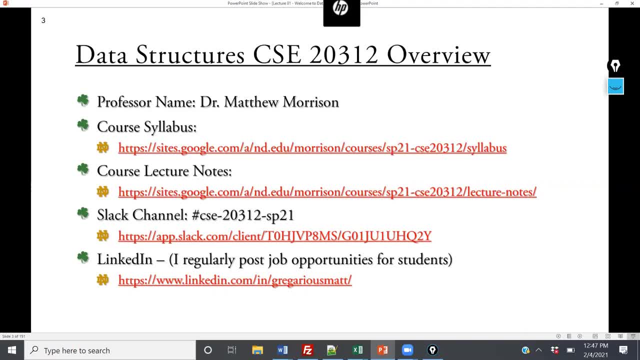 Everything builds from there and then what we're going to do is we're going to move from that which is imperative or procedural programming into this idea of object-oriented programming. How C plus plus uses libraries or you can build classes to be able to structure data in the way that you see fit in order to make your program work best. So it's the best way to understand this is to 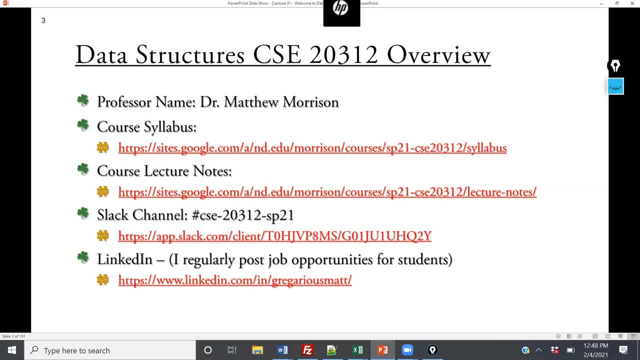 work from the ground up and to be able to see how your program works at different levels of abstraction. So here this information that I have, I have the links for the course syllabus, the links for the course syllabus, the links for the course syllabus, the links for the course 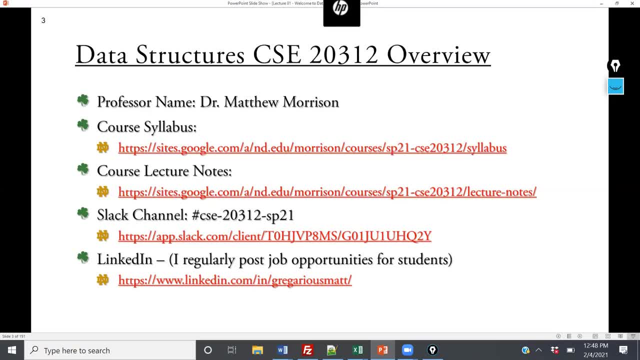 Lecture notes. I also have a Slack channel. I sent out an email a couple days ago. If you can't get into the Slack channel, shoot me an email and I will add you. And also a few of you have already found me on there. I have a LinkedIn page. I'm happy to connect. I regularly post job 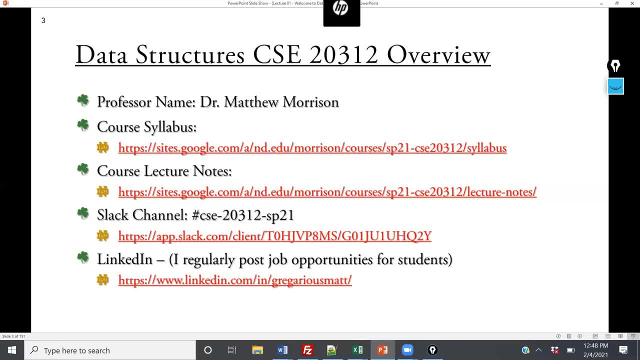 opportunities and internship opportunities to try to give you an opportunity to expand your job 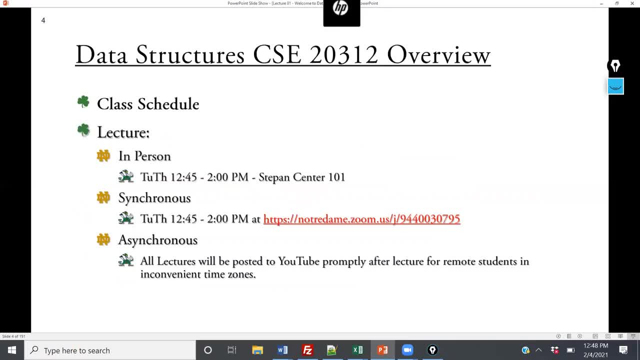 prospects. Lecture will be here at 1245 to 2 p.m. every Tuesday and Thursday. I will, and I'm broadcasting it right now on the Zoom. If for some reason you feel ill or you don't feel comfortable going outside, you are welcome to attend via Zoom. The only thing we got to work on is making sure that there's a property, I think, for the midterm and final exams. Otherwise, you do not have to ask my permission. You just watch on the Zoom. Furthermore, I record all the lectures on YouTube, posting them to YouTube. For those of you who've already seen the lecture schedule, you'll see I have everything for every lecture YouTube link available after class. And you have the ability, if for some reason you can't attend at the particular time, to go back and watch as well. And in the event that we have some sort of disruption 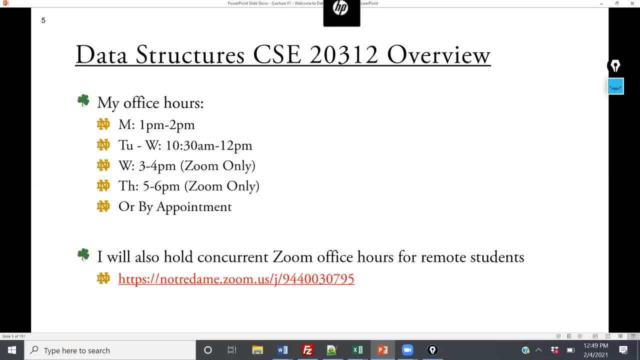 like we did last semester, we will continue to hold lecture on Zoom. Okay, so these are my office hours. Monday, 1 p.m. to 2 p.m. Monday, 1 p.m. to 2 p.m. Monday, 1 p.m. Monday, 1 p.m. Monday, 1 p.m. 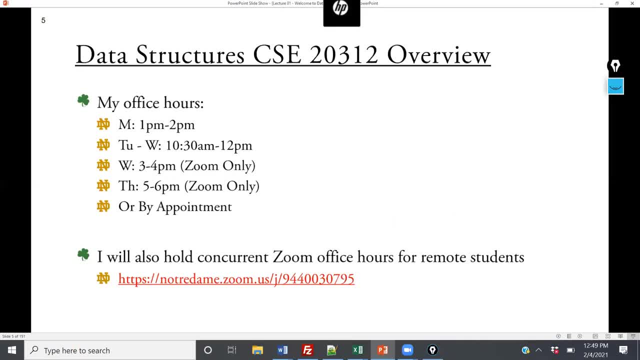 to 2 p.m. Tuesday and Wednesday, 10 p.m. to 12 p.m. I hold Zoom-only office hours on Wednesday and Thursday afternoons. And the reason I do that is because the coding challenges will be due every Thursday at midnight. And therefore, I want students to have the opportunity to be able to ask me questions. As you'll see when you get to the office hours for the teaching assistants, there are huge blocks of office hours on Wednesdays and Thursday nights. So that way, you have a good opportunity to be able to ask questions. And be able to progress on those and do well on those assignments. 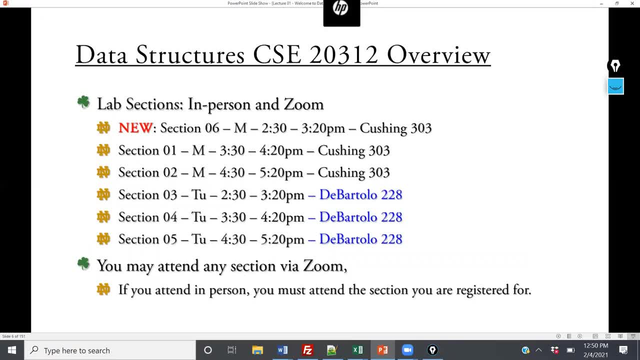 All right, so quick announcement regarding the labs. So we just created, so there was a little bit of scheduling drama. And what we're trying to do to work with it is that there is a new Section 6 that's a Monday from 2.30 to 3.30. And the Sections 1 and 2 are still at the same time and pushing 3.03. We have to move Sections 3, 4, and 5. 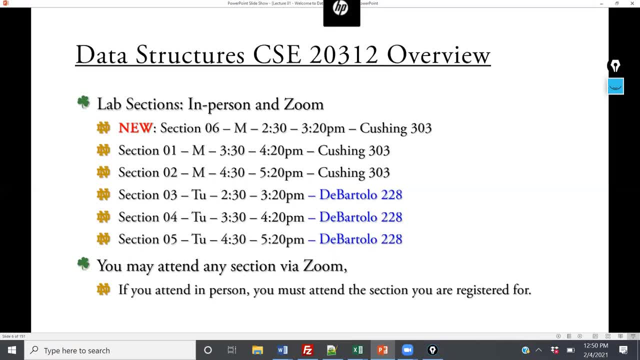 So we're going to move those sections back to the Bartolo 228. That's something that was just worked out this morning. Ramsey sent out a couple emails, but I want to make sure that I announced it here as well. You are, so if you want to move over, in order to meet the spacing requirements, we actually need four students from Section 3 and one student from Section 4 to move. 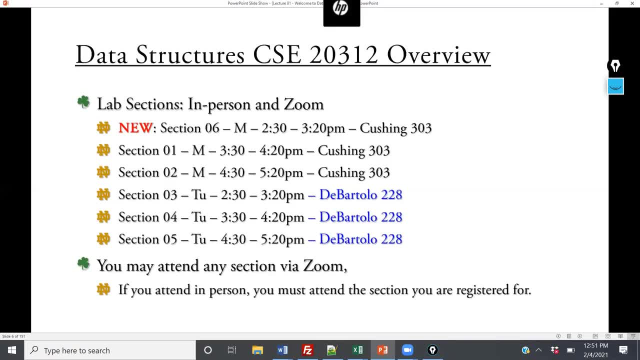 But my understanding is that the Monday sections are more coveted. So therefore, if you want to try to register for those, that first come first serve basis. Furthermore, we'll be having a Zoom room. You are welcome to attend any lab section you like via Zoom. 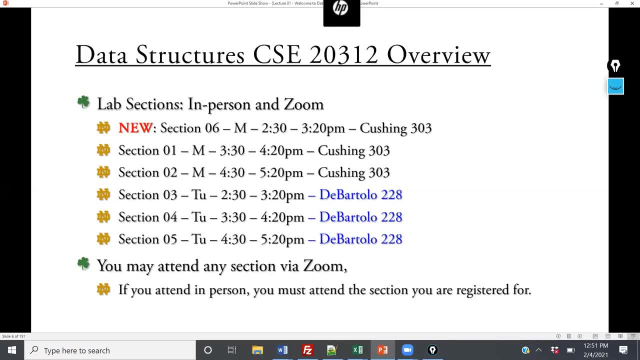 TAs will be attending via Zoom, and you'll make a breakout room to present your lab work. And therefore, you can attend. But if you want to attend in person, you have to attend in the lab section that you're registered for. Does anybody have any questions about 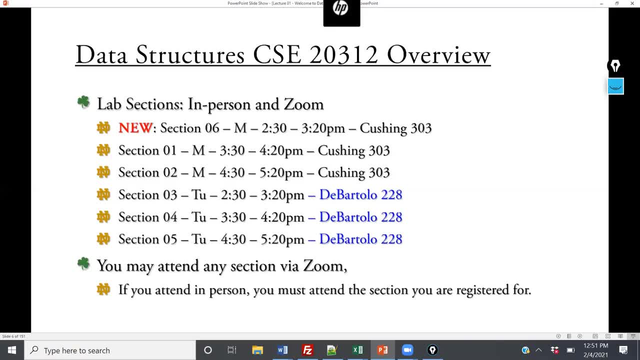 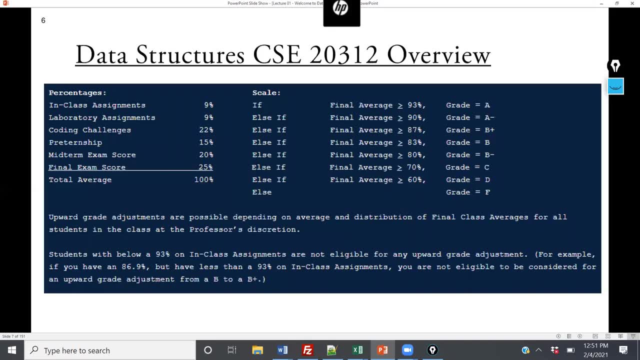 this before I go on? All right. So this is the grading breakdown. My grading breakdown is breaking down into five parts. There are in-class assignments, which I'll describe in a moment. There are laboratory assignments. And both of those are building up to the coding challenges. 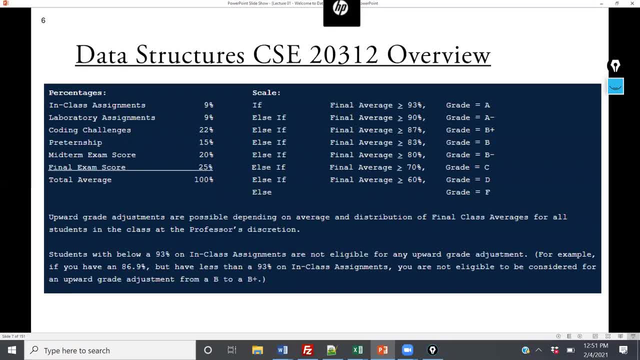 There'll be eight of those throughout the first part of the semester. And then the last third of the semester, we're working on the pre-turnship project. And the pre-turnship project is a final group project where you'll actually be working with an industry mentor to build a large project. 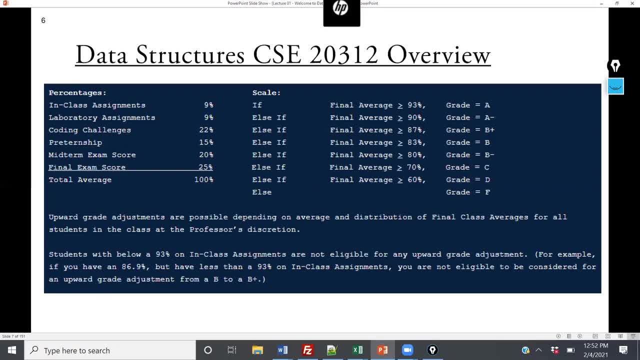 Then there's the midterm and the final exam. And what I have here at the bottom is this idea of upward grade adjustment. So what I can do is in the event that you're really close, like you're borderline A, A minus, A minus, B plus, something like that, by saying that, I reserve the right to be able to move your grade up if I feel that's appropriate. I have one rule, though. The rule is I will only provide that for students who have a 90% or higher on the in-class assignment. 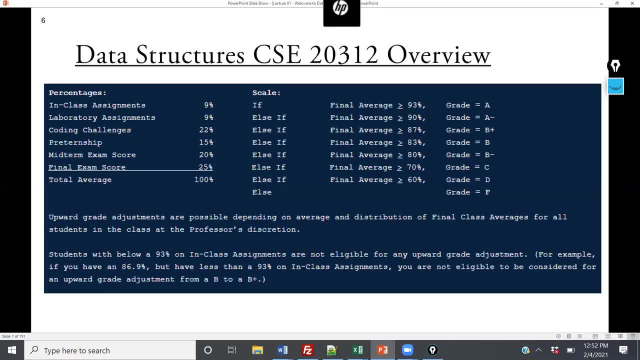 The thing is, for the in-class assignments, you'll work on a problem, and then I'm going to present the solution, and we'll discuss the process. So if you attend lecture and submit them on time, you should have no problem getting 100%. 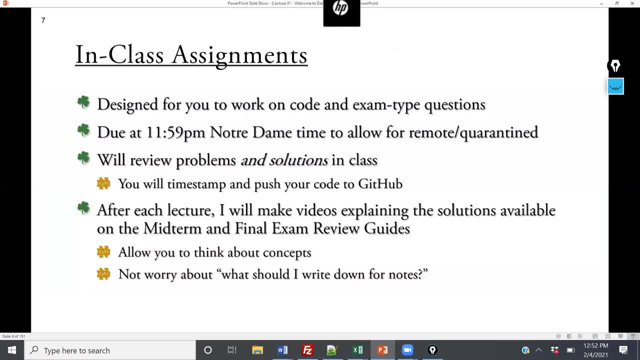 Okay, so the in-class assignments. Basically, what I'm going to do is I'm going to discuss a concept and then allow you to work on one or two problems. Each lecture should have about six or seven total where you're actually going to get the opportunity to see if you understand what the concept is. You'll actually work on a problem. It'll be very similar 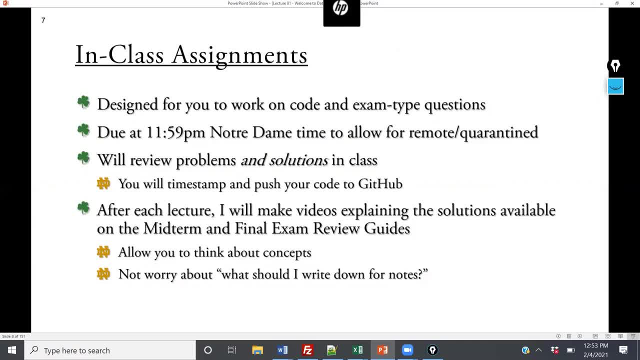 to the type of problem that I will ask on an exam. You'll demonstrate that you understand it. You'll learn if you make a mistake in a low-risk environment, and you'll understand how I ask 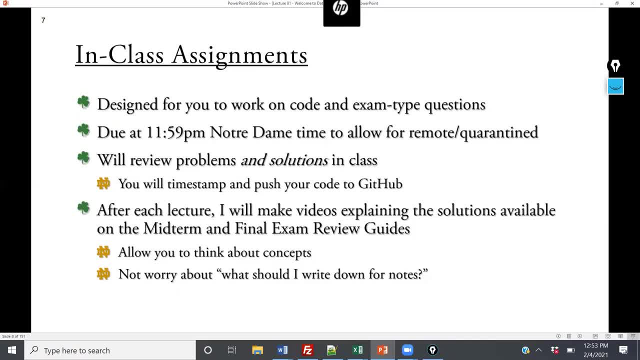 questions on the exam, so that way it ensures fairness. And furthermore, one of the benefits is I believe that the best way to learn data structures materials should be trying to 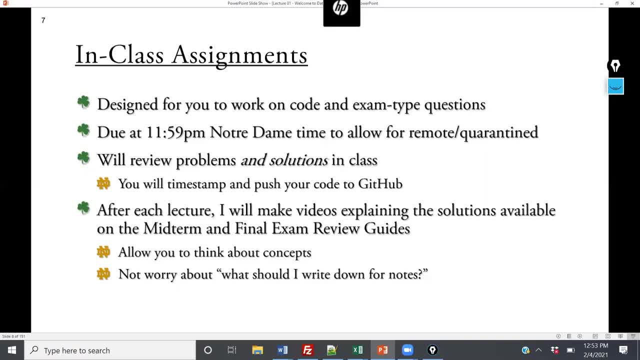 think through it. I don't want you to feel like you have to constantly guess, in my lecture, about what notes to write down. And so to emphasize that, not only will I go over the answer in class, but I'm also going to have a link, which is a midterm review, and we'll have the problem, and I'll have a short video where I describe the solution as well. And that will 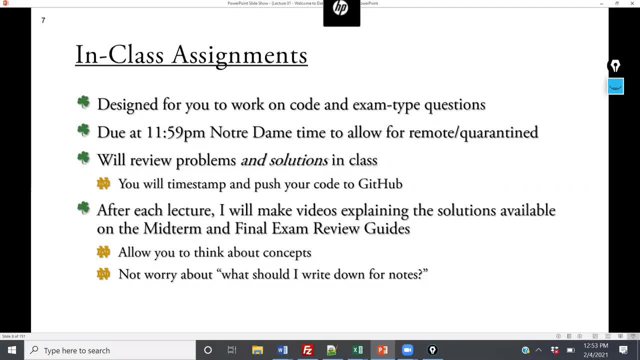 actually be building up the midterm and final reviews for you. So what I want you to do is kind 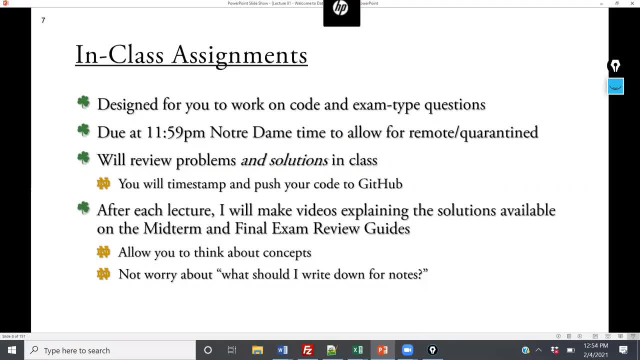 of more thinking through the process, trying to visualize the data structure, how it's operating, and then apply that understanding. So that's why that's my advice. 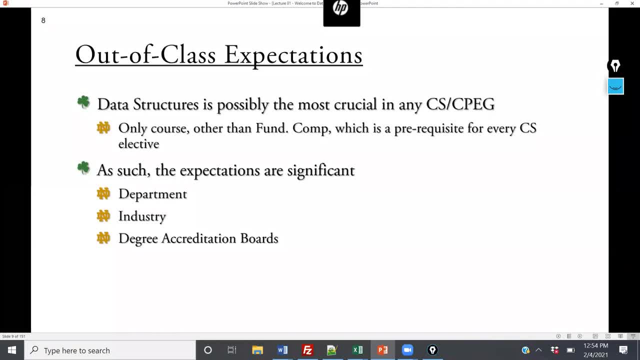 So out-of-class expectations. So with data structures, this course is unique in that, with the exception of fundamentals of computing, it's a prerequisite for every single required and elective course in the curriculum. Furthermore, and I'm sure many of you know this already, this is the course that industry really starts to expect you to understand when you start applying for jobs. 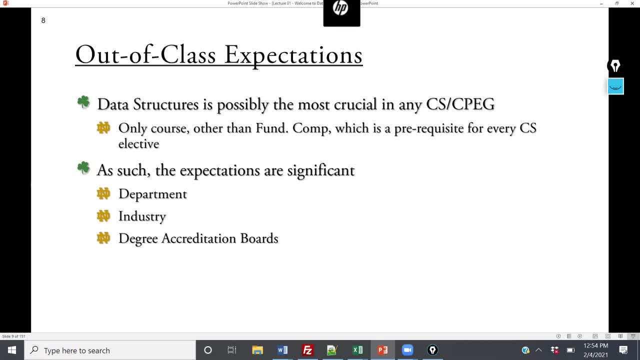 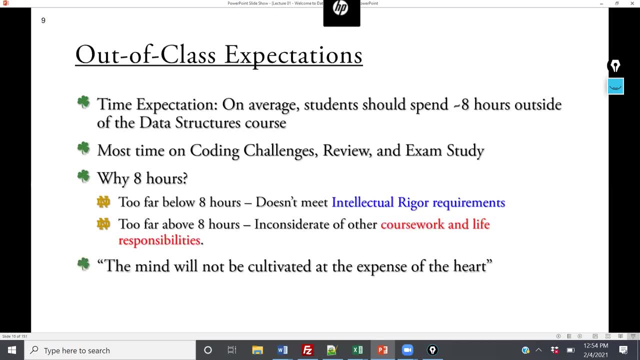 As a result, the expectations can be a little higher than your normal class that you might have had up to this point. So the rule that I have come up with is that a good amount of work outside of class per week is on average eight hours. If you go too far below eight hours, you don't meet the intellectual rigor that is expected from industry or degree accreditation boards to make your degree valuable. If I go too far above eight hours, then that starts eating into your time for other classes, your time to actually be able to relax and do other activities. So that's kind of the goal that I have there to make sure that I'm working that balance. I've included this quote from the Holy Cross that is also mentioned to Notre Dame students that the mind will not be cultivated at the expense of the heart. So I know that I have to provide an intellectually rigorous course but I want you to make sure that you understand that I'm going to work with you and the TAs are going to work with you to make sure that you're going to be able to achieve those goals. And I do think it's an 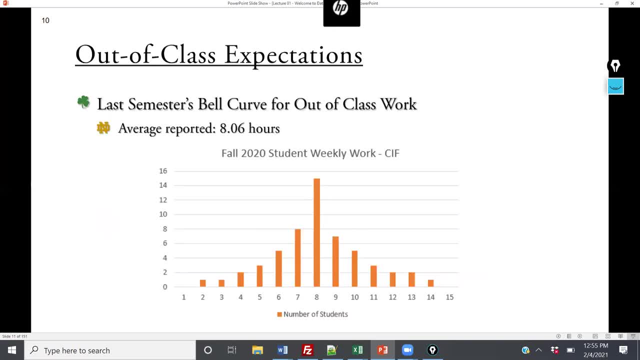 that you all succeed. So on that point, this is the bell curve from the SIF from last semester students, and it came out almost exactly at 8. It's 8.06. So the million dollar question that some of you might be thinking, right, is what happens if I'm on the wrong side of the bell 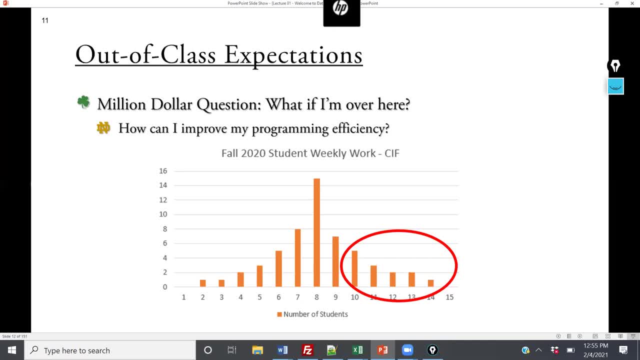 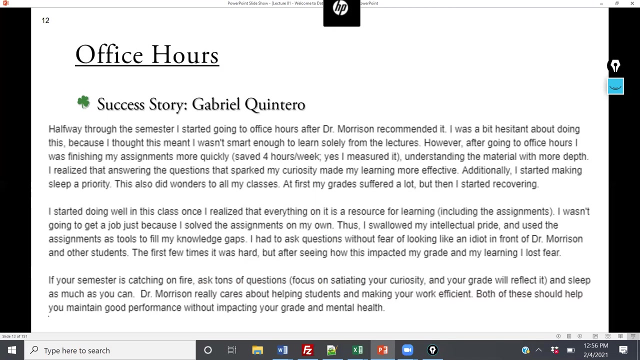 curve? What happens if you're really struggling, you're taking 14, 15 hours a week, you're pulling your hair out, you're really frustrated? First and foremost, I want to say that does not mean you're a bad programmer and you should drop out of computer science or computer engineering, but it's an opportunity for us to be able to intervene and work with you. I want to give you an example of a student from last semester, Gabriel Contero, who about at the, I want to say with a 40% mark of the course, was actually failing, and he was taking an incredible amount of time on the assignment, and he came in and he was telling me this, and I was going through his process, and the recommendation I made to him is come to office. Ask questions. Do these kind of things and identify when the moment you get stuck, find me, find a teaching assistant, and from then on, I could count on every single time I opened the door to start office hours, he'd be waiting outside, waiting for me, and so I've included this note because I consider it a success story because he actually thought it's great up to a B plus. It's really impressive. So I want to root through this note that he said because I asked him to make this kind of thing for you to kind of motivate you as you're working through this. He says, 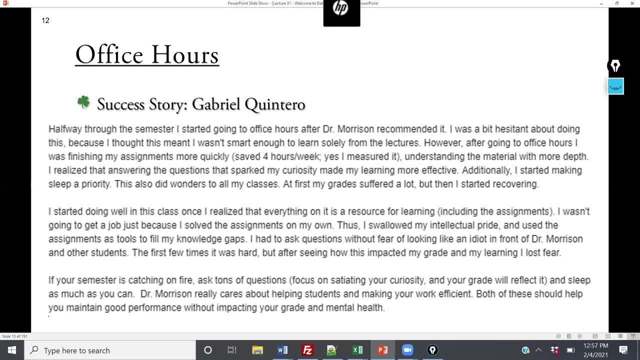 halfway through this, I started going to office hours after Dr. Morrison recommended. I was a bit hesitant about doing this because I thought this meant I wasn't smart enough to solely learn from the lectures. However, after going to office hours, I was finishing my assignments more quickly. Saved four hours per week. Yes, I measured it. 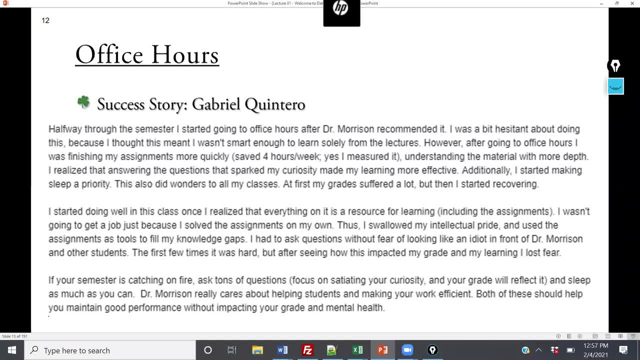 Understanding the material with more depth, I was realizing that answering the questions that sparked my curiosity made my learning more effective. Additionally, I started making sleep a priority. 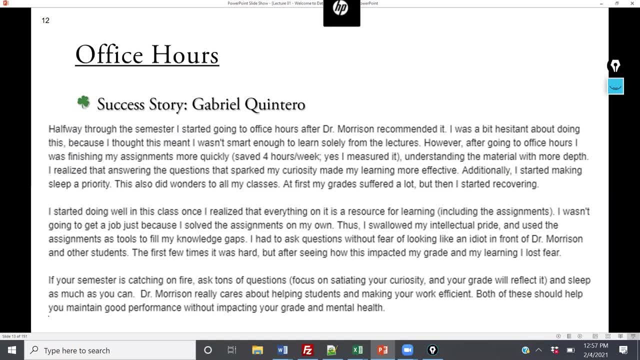 This also did wonders for all my classes. At first, my grades suffered a lot, but then I started recovering. I started doing well in this class once I realized that everything on its own is a resource for learning, including the assignments. I wasn't going to get a job just because I solved the assignments on my own. It's not like you're about to get your job offer at your dream company, and I'm just going to hop out from behind nowhere and go, oh, you didn't do coding challenge three the first time without help. You can't get hired. I'm not going to do anything like that. 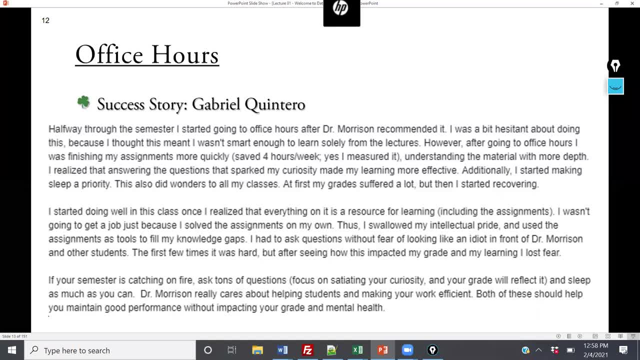 I wasn't just going to tell you. Thus, I swallowed my intellectual pride and used the assignments as tools to fill my knowledge gaps. I had to ask questions without fear of looking like an idiot in front of Dr. Morrison and the other students. Trust me, we're all not judging. We all want to be here to help. 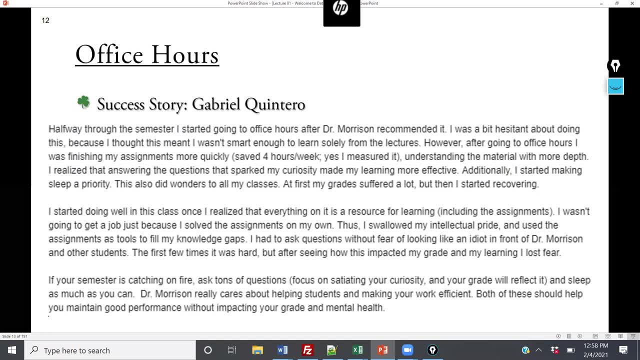 The first few times it was hard, but after seeing how much this impacted my learning, I lost fear. So I want to take this last thing. This is great advice, especially if the semester starts getting a little more stressful. If your semester is catching on fire, ask tons of questions. Focus on satiating your curiosity. 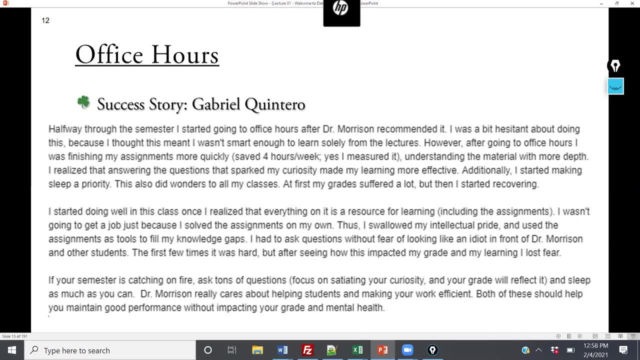 Your curiosity and your grade will reflect it. And sleep as much as you can. 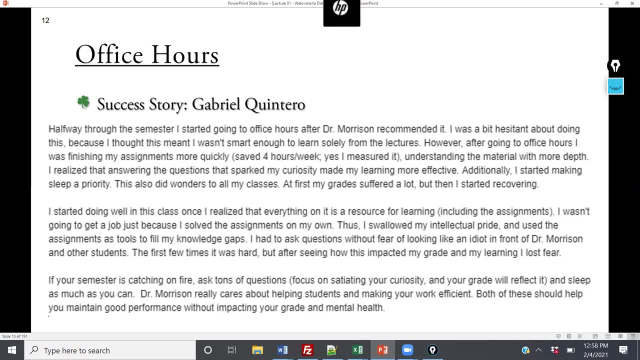 He's true when he says this, that I really care about helping the students and making your work efficient. Both of these things should help you manage performance without impacting your grade and mental health. 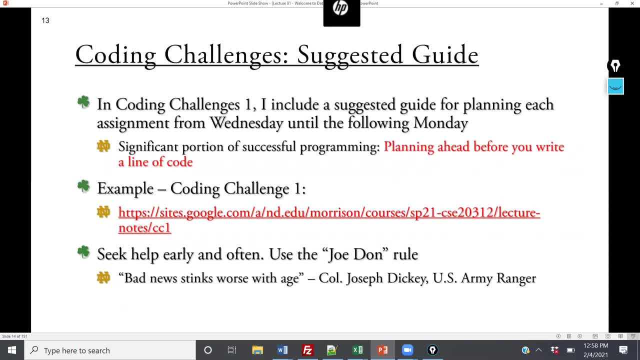 So, for example, on coding challenge one, they are officially assigned on a Wednesday, and then they're due the following Thursday. So there's eight days. And for an example, I have 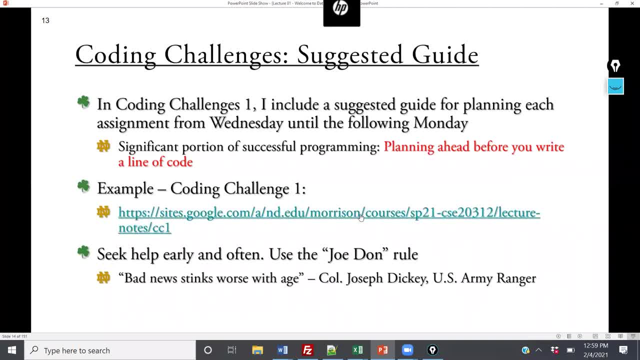 Click on this link here to show you. And what I've included, Once it comes up, I'll show you. I'll click on it. 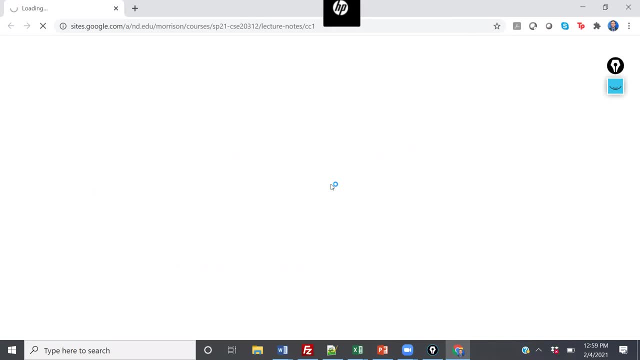 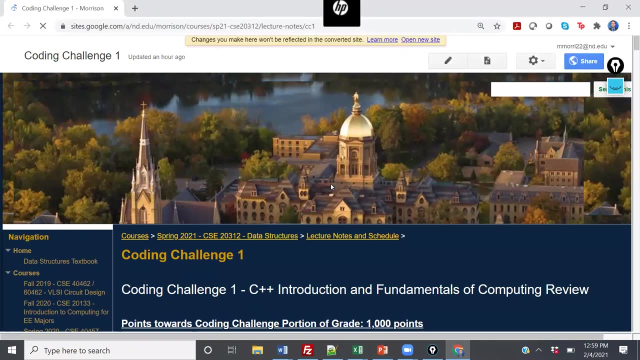 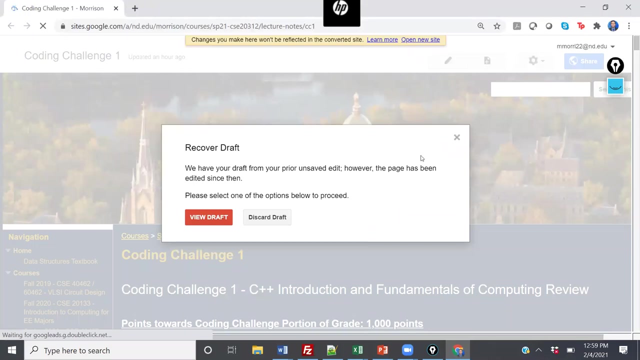 Is I've included a sample link on how to plan out working on a coding project. As you get further into your coding career, what you're going to see is that You become a much more effective programmer and you're doing most of the work before you write a single line of code. And so, no, I do not want to recover draft. 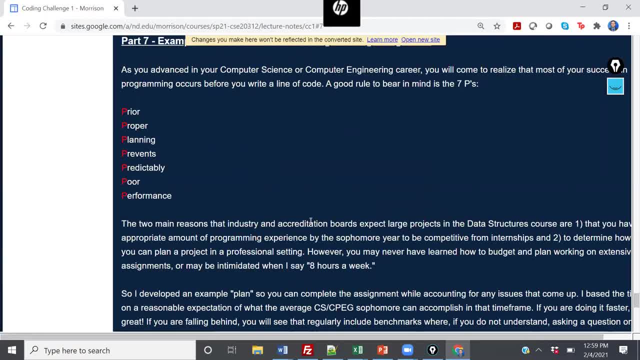 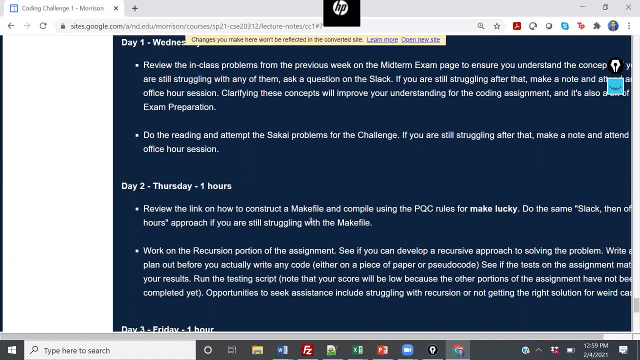 And so here I have example schedule and plan for and I have Written out like a certain amount of time. And more importantly, I have benchmarks, where if you don't understand it, don't find us in the office and ask Did you have your hand up in the back there. 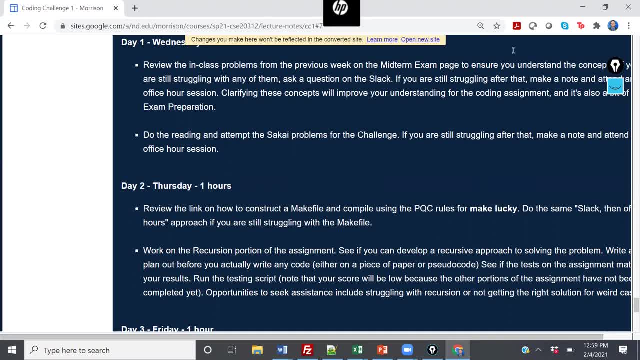 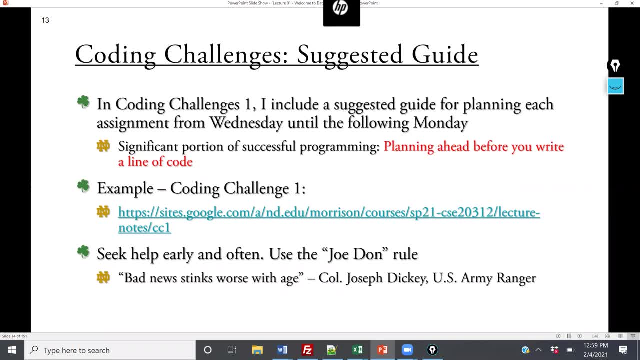 So I just want to show you this But I also have what I call the Joe Don rule Joe Don and say the army ranger friend of mine back in Mississippi. He said bad news things work with age. 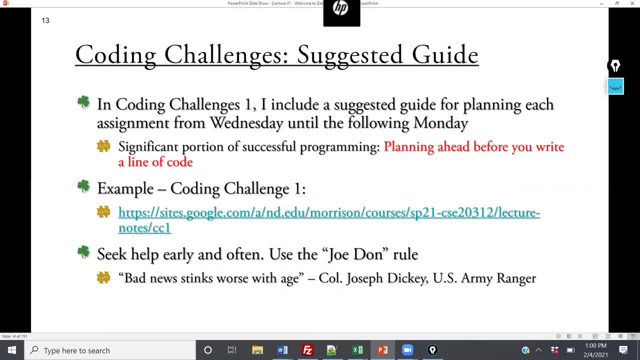 If you are proactive about getting help. I promise you'll I'm going to cut down the amount of time that you need to do. 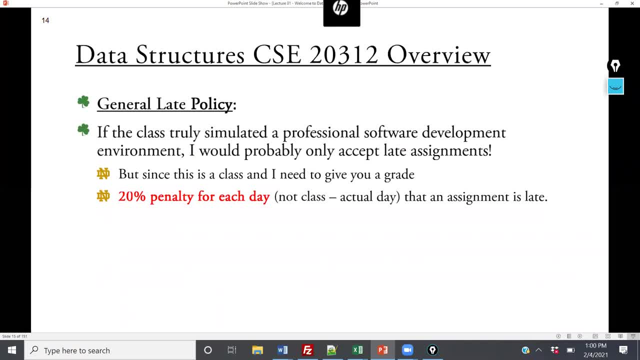 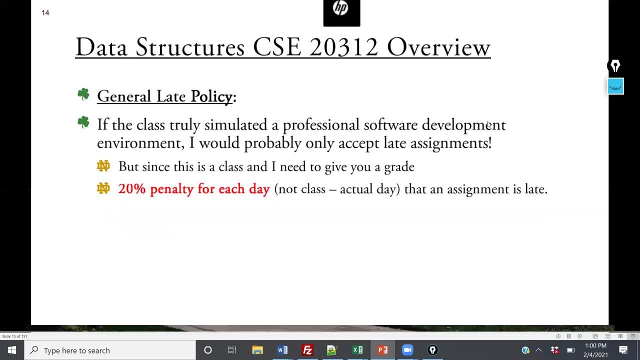 Does anybody have any questions about the out of class and comments, anything like that before I can The other thing I'm going to do is I'll occasionally check the chat, just to make sure. Okay. 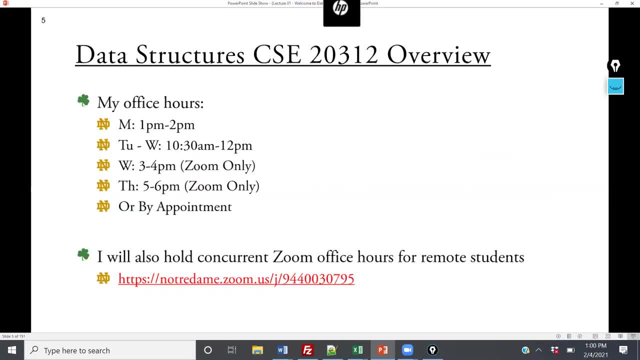 So a couple quick things on Submission and late policies. 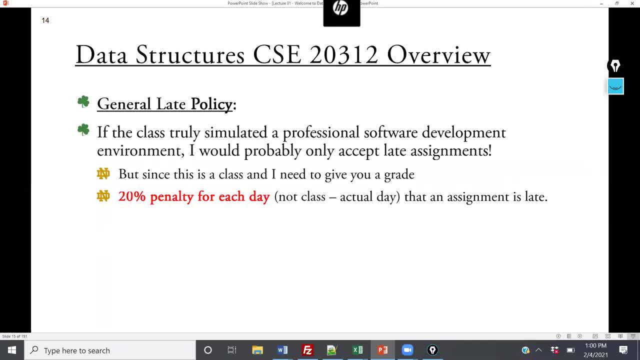 But so Generally, for the coding assignments or the labs. 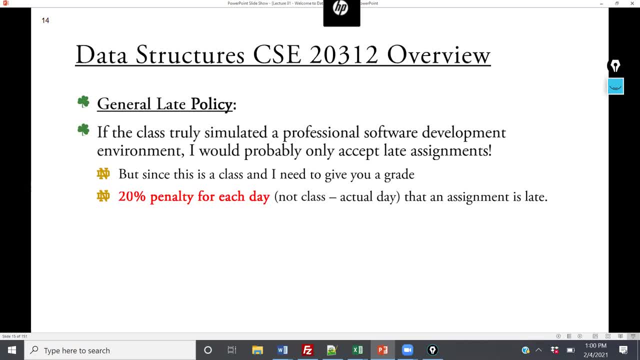 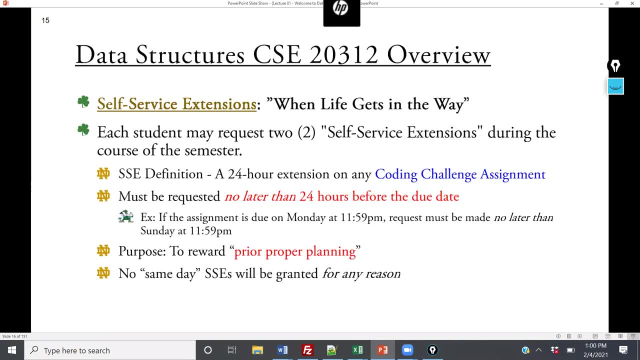 It's a 20% deduction for each day that is late. However, I have what are called self service extensions and you get two of them for it for out of the eight coding challenges. And what it is, is that you can request a one day extension on assignment with no penalty. 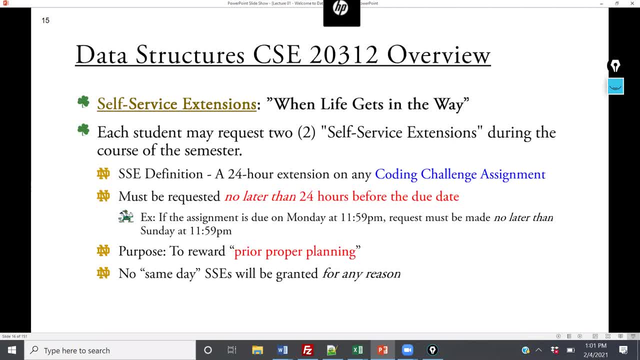 My only rules that you have to ask With With no later than With no later than 24 hours before the lab. 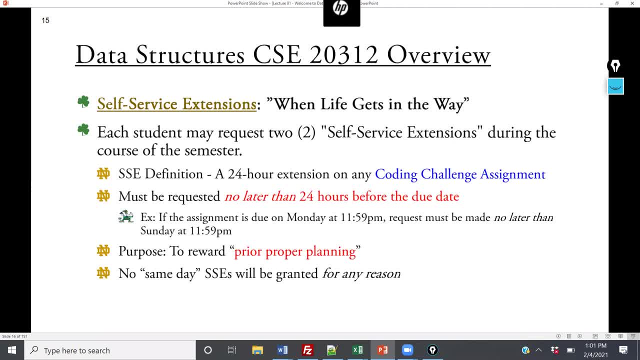 With no later than 24 hours before the lab. With no later than 24 hours before the lab. the assignment is due. So the objective here is to reward prior proper planning on an assignment. 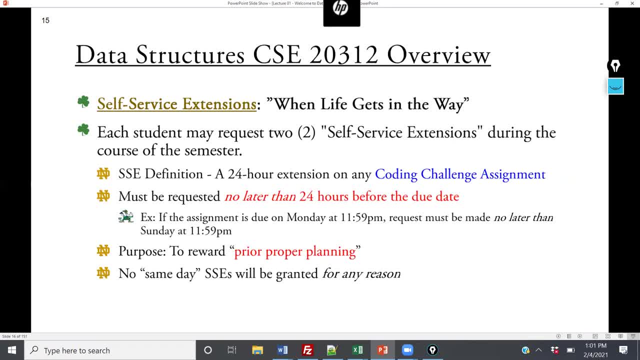 If you do that, and I have the times for each assignment about when a self-service extension would be due, if you do that, you can get a full 24 hours. And the objective is to consider when life gets in the way, another assignment took longer than you expected, you have a big exam, I want to make sure that we're accounting for this appropriately. Furthermore, if you are sick 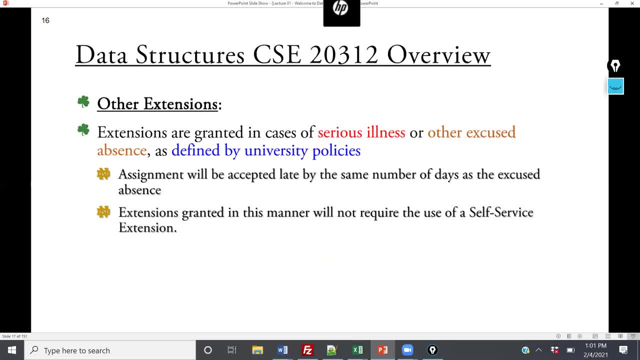 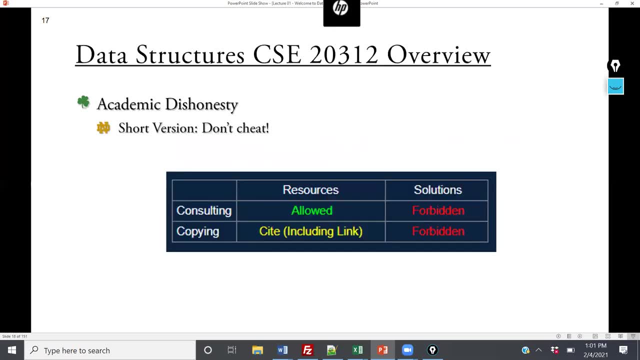 or something comes up, life happens, you contact with me, I'm happy to work with you and you won't have to use a self-service extension on there. A quick academic dishonesty spiel. So short version, 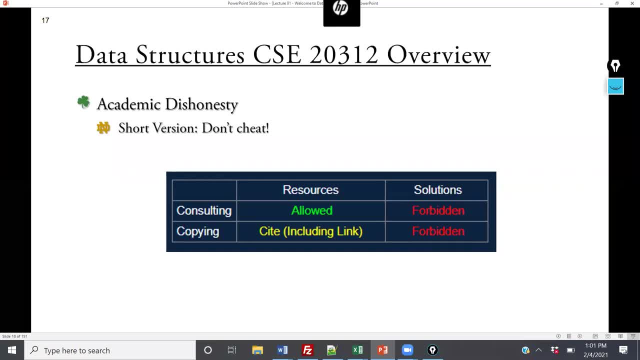 don't cheat. So the question is, what actually is cheating in computer science? This can be a tough, it can be hard to understand the first time you're going through, so I want to give you a quick spiel on it. There's a difference between resources and solutions. So if you see something that describes an algorithm on Wikipedia, that's fine if you cite it, but if you actually go on Geeks for Geeks and copy code, even if it's only part of it, that's generally a bad idea. 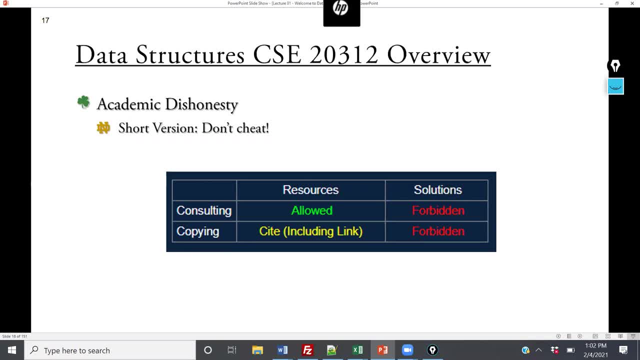 The whole goal is you should have what you submit should be what came out of your mind. So if you're talking to one of your classmates, it shouldn't be like, okay, well, here's my exact code. But if I talk to my classmates, and now I understand something better because of it, and I'm able to now solve this problem, because I understand it better, that's perfectly fine. 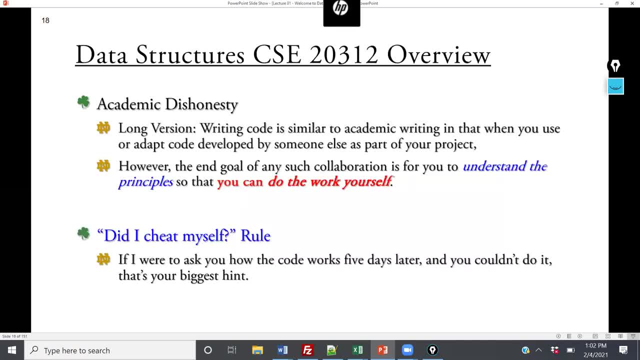 So here's a good rule that I like to follow. I call it the did I cheat myself rule. The whole goal of any of these assignments and these concepts is so that you understand the principles and can implement them after graduation. I like to think that my class is important, but in the grand scheme of things, it's not. But if you can take those skills and build upon them on your own, that's what truly makes this worthwhile. So the did I cheat myself rule is if you look back, in your code, where if I were to look at a code you submitted, I said, can you tell me what this code does, and you can't do it, then you cheated yourself. And the crucial thing is that when you 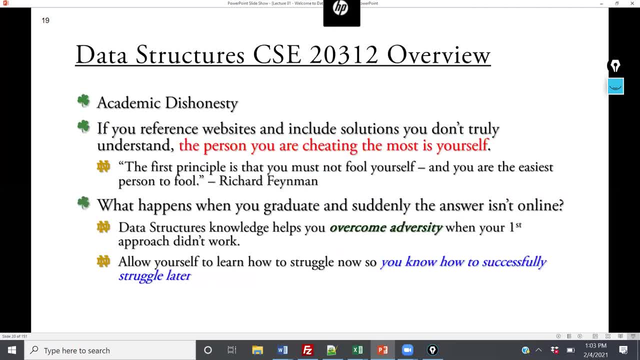 cheat and do something like that, the person you're hurting the most, the cheating the most, is yourself. Because you don't want to put yourself in those positions where you think you understand something, and then you hit a real-world situation and you don't. I like to cite Richard Feynman, a Nobel Prize-winning physicist, who said, the first principle is that you must not fool 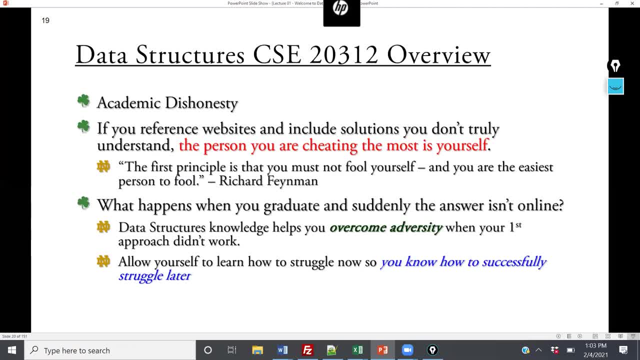 yourself, and you must not cheat yourself. And the second principle is that you must not fool yourself, and you are the easiest person to fool. So what happens when you graduate and some of the answer is online? 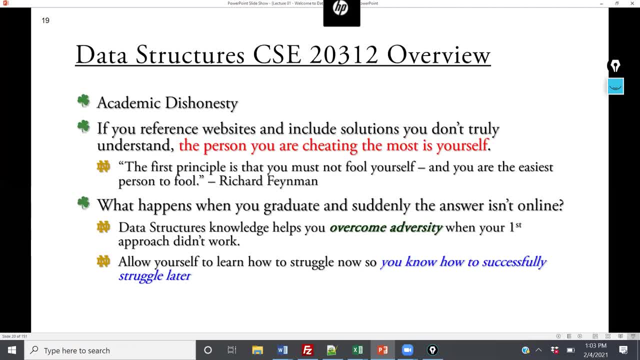 The one thing I want you to take away from this first lecture is that the idea of data structures is that you're learning how to apply different structuring principles to learn how to overcome adversity. What happens when your first approach doesn't work? Should I use a hash table? Should I use a tree? You know, should I use a graph? What kind of concepts, speed, memory, all these things contribute. And if something doesn't work the first time or doesn't meet appropriate benchmarks, you can use your knowledge of data structures to think, okay, instead of panicking, I can think this through. Oh, that's right. Maybe I should use a hash map. That'll improve speed. Or, oh, I'm using way too much memory. The hash maps take up too much memory. I can significantly reduce memory and get good enough access with a red-black tree, for example. So if you're taking that kind of stuff and you're approaching the course that way, it will really only help you once you graduate. 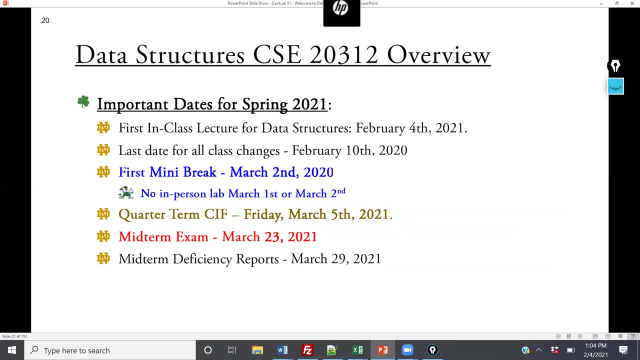 All right, so quick overview of the important dates for the semester. 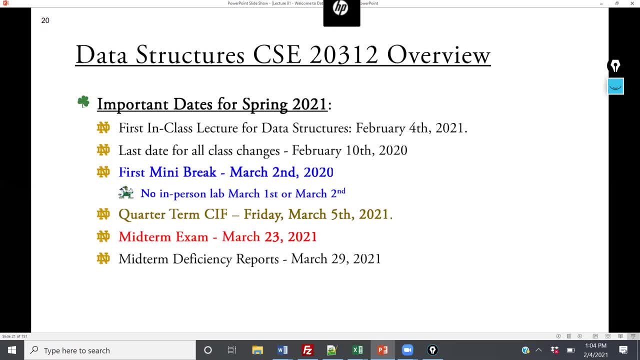 The first mini break is March 2nd, so the university is imposing two mini breaks. One is going to be March 2nd is a Tuesday, and so there's no classes, and we are directed. We cannot assign anything. We can't hold office hours. That is your day to relax. 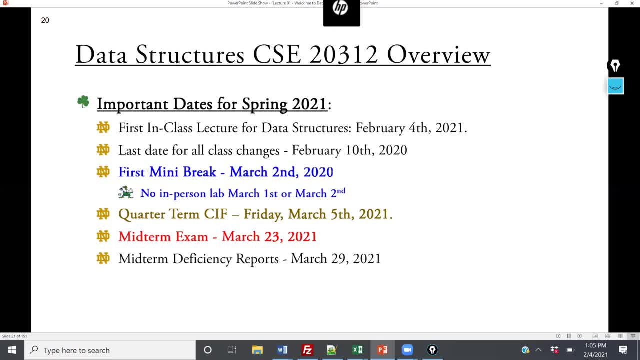 Because of this, the labs on Monday and Tuesday have also canceled the Monday lab as well. So those two labs are canceled for the mini break. I also do a quarter-term SIP. 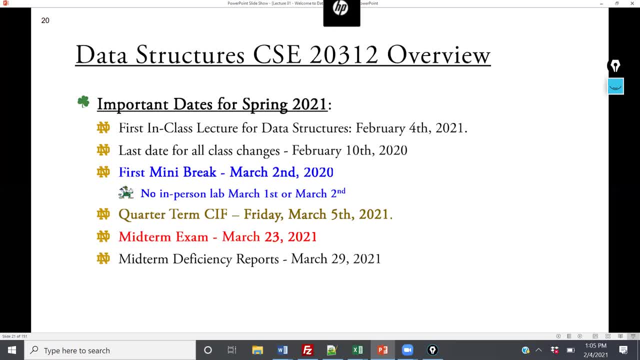 I'm going to be doing that on Friday, March 5th, and it gives me a good idea of how the class is coming along, how you're feeling, and I can make appropriate tweaks to the class if there's something prescriptive that I can do to improve the student experience. Then the midterm exam is 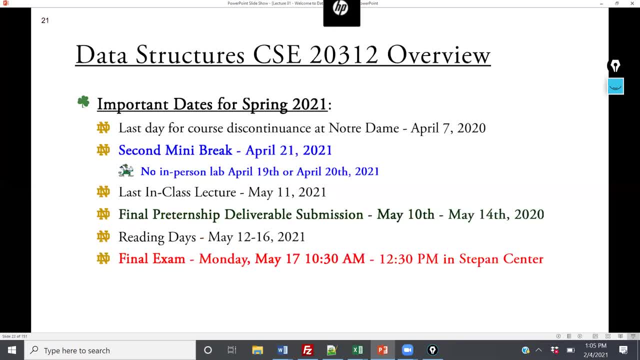 on Tuesday, March 23rd. The second mini break is April 21st, so I'm also canceling that. I'm going to be doing the labs for that week as well. Then last in-class lecture is May 11th on the Tuesday. 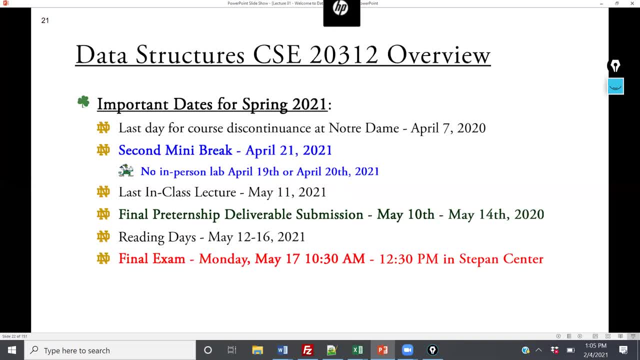 The final preternship deliverables, you'll understand a lot more about what I mean by that later, are that final week. Then the final exam tentatively is Monday at 10 30 a.m. on May 17th. 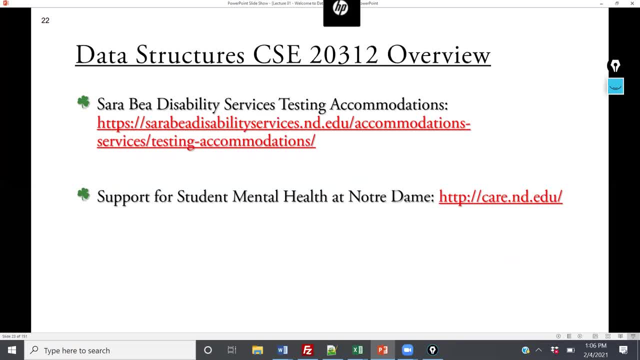 You'll be able to take care of all that. The other crucial thing, and I know I've been emphasizing this idea that we're trying to make the course efficient, is that no assignment that I have is worth compromising your mental health. So if you're struggling with something, please do not hesitate. I won't shame you. There have been times when the students have been really struggling, where I've actually just called the Sarah B. Center and said, can you give me permission to give the student an extension or get them to help me? I'm happy to help you. 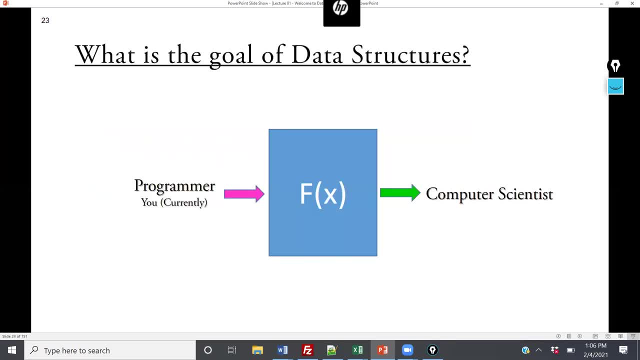 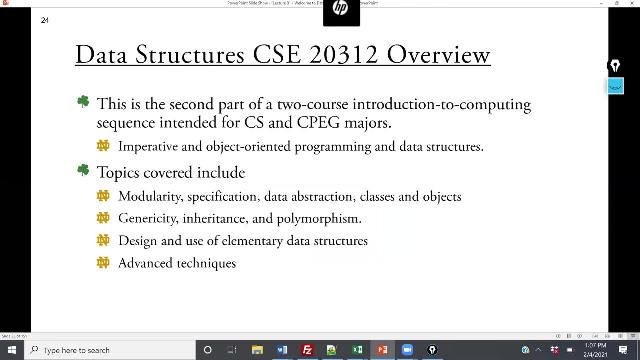 All right. So what is one of the goals of this data structures course? So up to this point, you've done a lot of programming. In previous courses, you've coded in C. Maybe you have a little experience with C++, and you've learned, okay, I write something, and the code does something else. And basically, think of data structures as a function, where before you are just a programmer, and when I say just a programmer, I mean you're not implementing mathematical and physical understanding of certain principles. And by the time you're done, you're a computer scientist. So my goal is that by the end of this course, I will look at you as a peer. And that's an awesome thing, especially at the sophomore level. I think that's one of the best things about our field. So the whole goal, and this is more from the course description, is that you're going to be learning about imperative and object-oriented programming and data structures. So you're going to be learning about imperative and object-oriented programming and data structures. 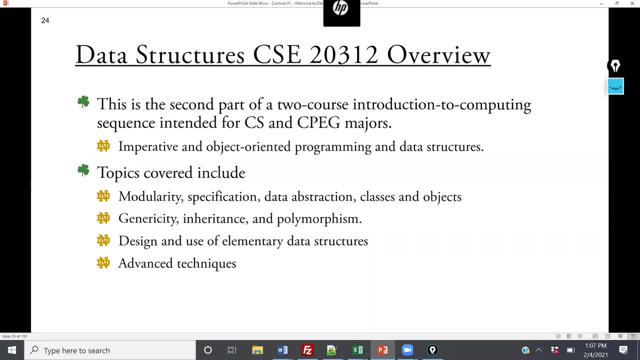 So you learned a lot about procedural programming in fundamentals. Memory management, pointers, being able to make functions and kind of run them through the computer. So you will learn this, but you'll see this, and how it contributes to putting memory on the instruction memory and the data stack. You're going to learn a lot about that in this course, and how to make that efficient and reliable. And then we're going to learn about object-oriented programming, which is actually a different kind of philosophy as opposed to C. So C++, we build classes, we build them as objects, and the goal is to treat these objects interacting as you would do in the real world. So for example, human sits in chair, you know, dog wants pets. There's certain kinds of things that objects do that we might not necessarily be able to represent in a normal procedural language. And from there, we're going to learn about the design and use of elementary data structures and how to have them be implemented effectively. 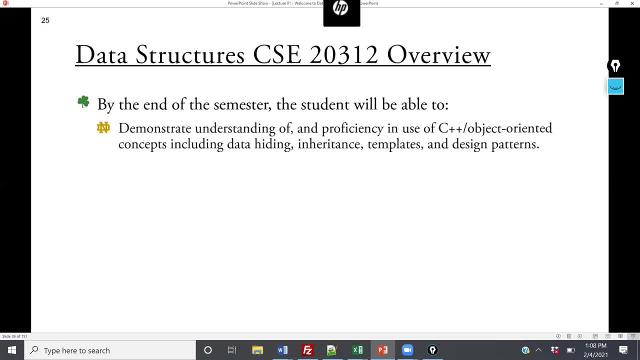 So by the end of the semester, here is what we expect you to be able to do. So to be able to 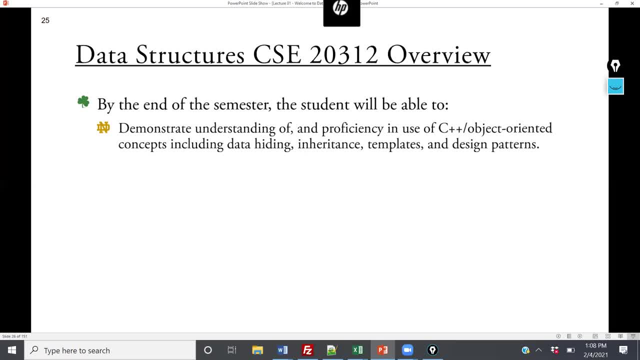 demonstrate understanding of and proficiency in use of C++ and object-oriented concepts, including data hiding, which is going to be really important to protect security and reliability of data. Inheritance, so very briefly on inheritance, you know, everybody in here is a person except for 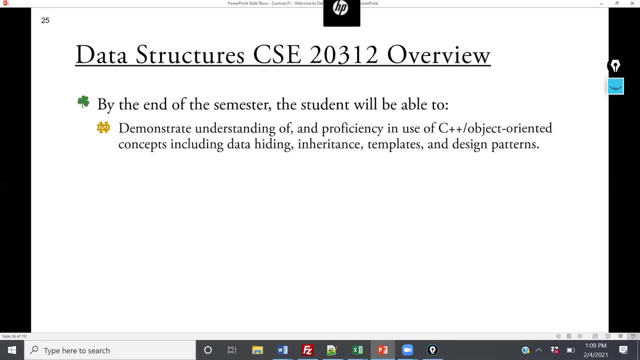 one, only one dog, but then there's categories. We have Irish, everybody's a member of the Notre Dame community, but then you are Notre Dame students, I am a Notre Dame faculty. And then based on these inheritance, we can do different things in many forms, that's called polymorphism. So learn about these concepts in this course. Next, you learn about analyzing performance. So we're going to 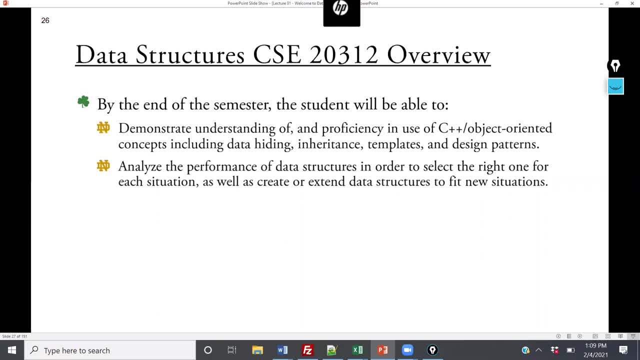 talk about things such as amortized analysis, Big O notation, something, the Big O notation is something you'll hit in a lot more for those of you taking discrete math this semester. 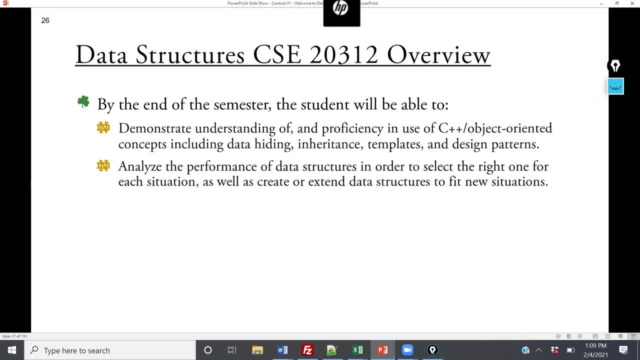 But the idea is, how can I measure with reasonable accuracy, the worst-case scenario for this particular program. And we're going to use that to be able to select the right fit for any situation. What does the customer want? How do we use this to be able to meet that requirement? And then finally, applying these data structures in real-world application, employing abstractions to make them work together cleanly and safely. 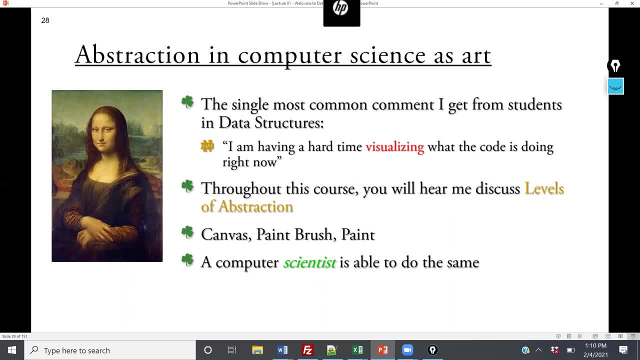 Okay, so when I say that computer science is also an art form, and when I say it's a type of abstraction, one thing I want you to think about is that they work on different levels, just like in a painting. So here we have the Mona Lisa. And the Mona Lisa at the surface, we just have a picture. But there's all kinds of things that go into a painting. You have different colors of paint, you have different thicknesses, you have different brushes, you have different types of canvases. And somebody who is really good at painting can take advantage of that in a way that's really helpful. 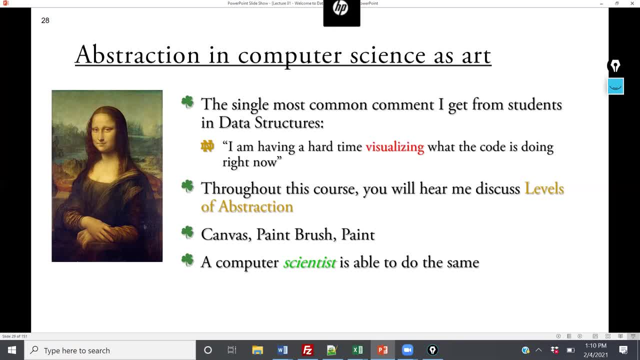 So I'm going to show you an example of a computer scientist who is able to do the same with hardware and software together. And that's the big thing about data structures is, okay, I'm writing a piece of code. How does this impact it when I put it in the hardware? And how can I take advantage of that knowledge to make the program run well? So this is Donald Knuth. I was 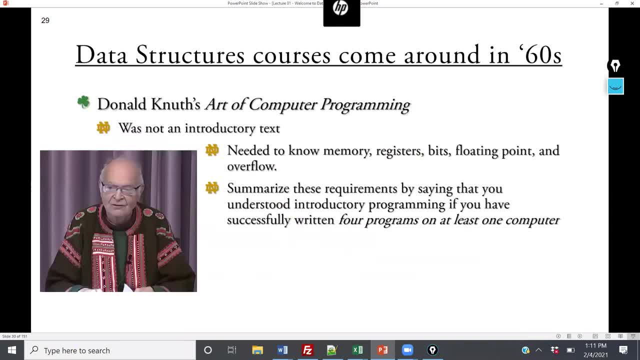 about to ask him a question. And he said, how do you make the program run well? And I said, well, I don't know. How do you make the program run well? And he said, how do you make the program run well? So this is Donald Knuth. I was about to ask him a question. And he said, how do you make the program run well? 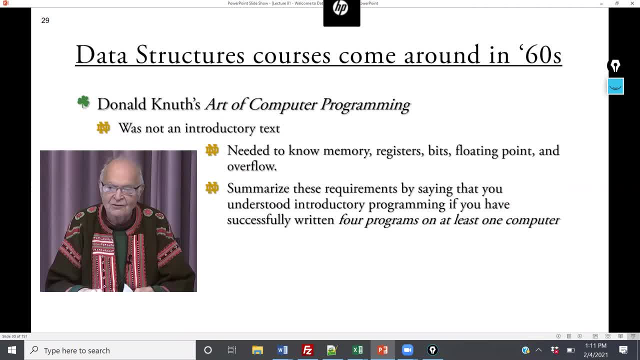 And I asked if anybody could tell me who that is, but his name is in big letters up there. So Donald Knuth is often called the Yoda of compute programming. And he wrote this book called the art of computer programming that started out in the 1950s and 60s. And he is a professor emeritus at Stanford now. And when he wrote this book, he actually stated, it's not an introductory text. 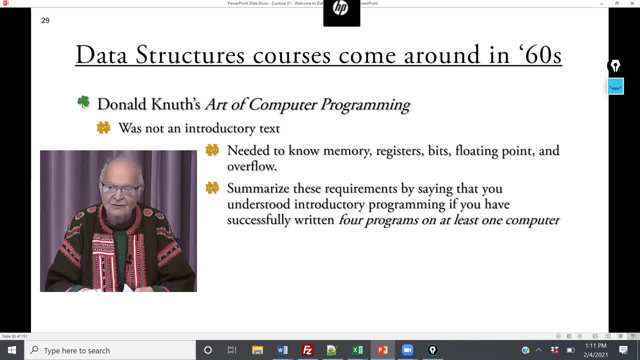 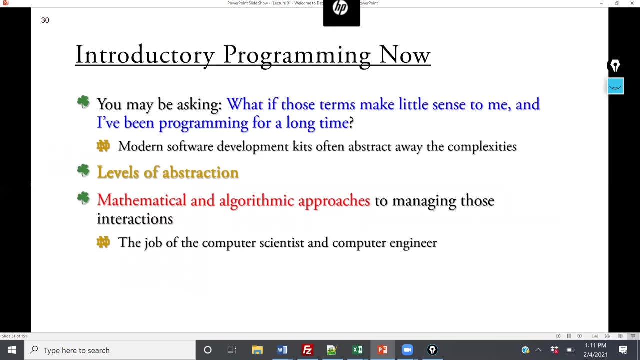 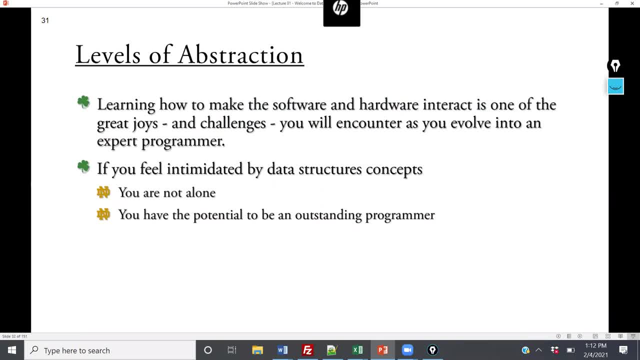 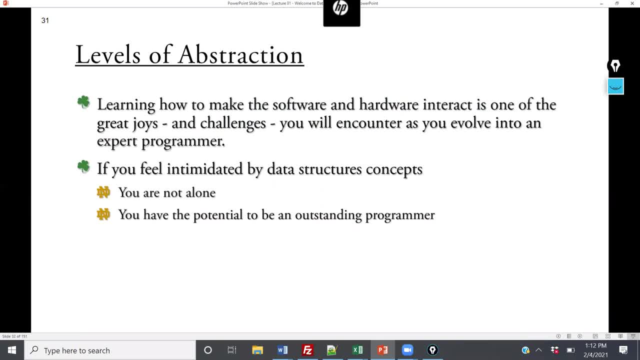 is one of the great joys but also one of the great challenges which is one of the reasons why 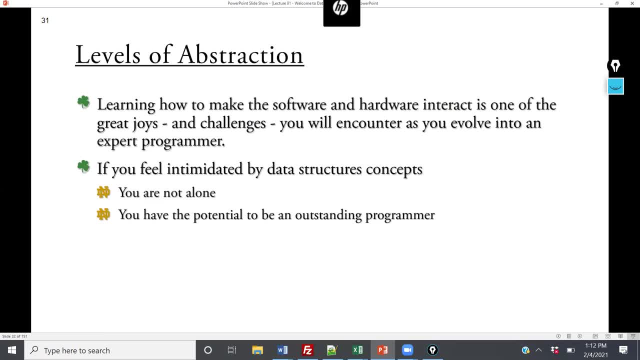 this particular course is considered so to be so important you know in competing for 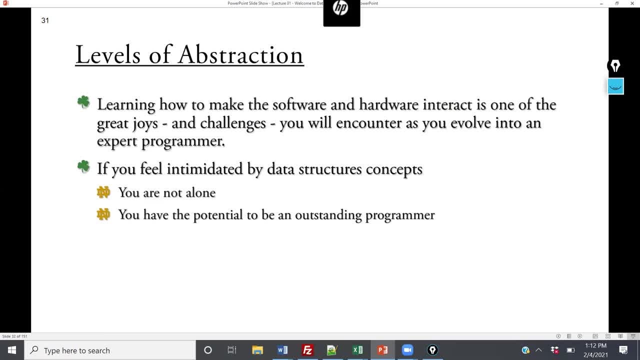 industry positions so i have this quick note if you're intimidated by this don't worry we're going to work with you we all want you to 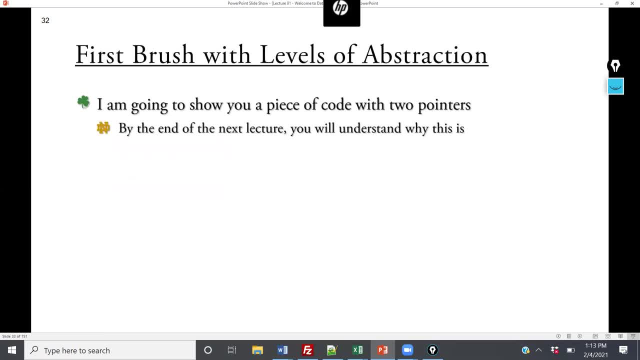 outstanding program. Okay, so before I go into levels of abstraction, does anybody have any questions? All right, so first, let me go through the list of the levels of abstraction that you'll need to understand to do well in this class and how a computer actually works. So the first one is this idea of pointers, and this, oh, I went too fast, sorry. 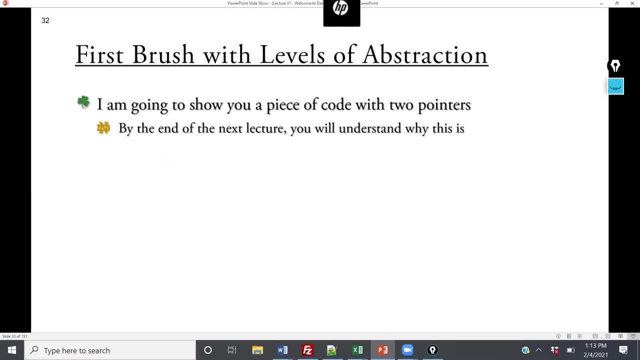 Okay, so what I'm going to do is I'm going to show you a piece of code that many of you, if you've coded in C++, you're going to be familiar with, and I'm going to make a claim that this code contains two pointers, and it might not look that way. So this is actually just hello world in C++. 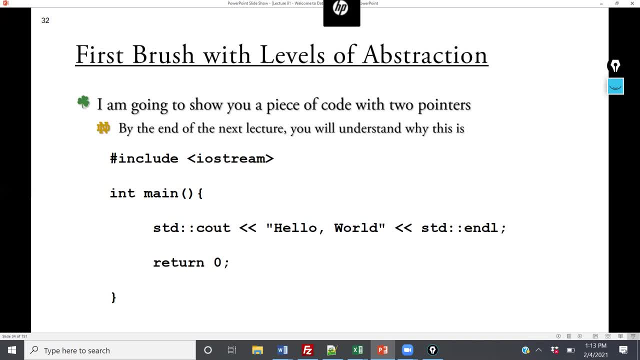 You have what's known as standard CL. For those of you who are not familiar with standard CL, it's an object-oriented version of printf or fprintf, and then I have a hello world and then standard nline. That is just puts a backslash n in the line of code. 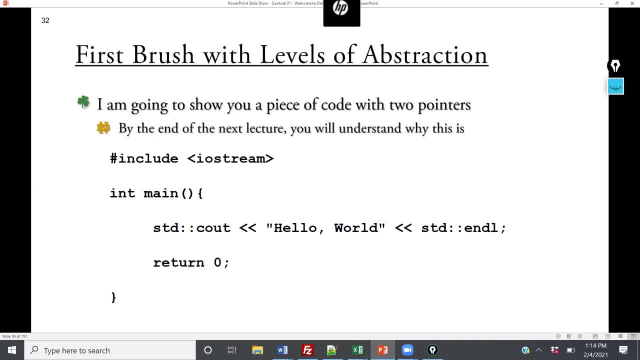 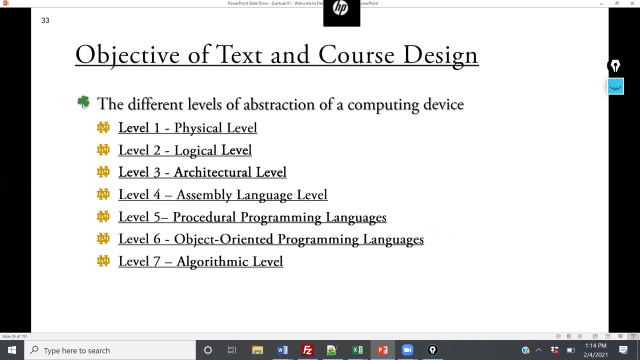 So by the end of this lecture, I'm going to give you an example of why this is actually contains two pointers, and when you start to be able to see code like that at different levels of abstraction, you'll be able to implement and master C++ in a better way. So the first level is a physical level, and we're not going to go into that at all in this course. That's transistors, that's silicon, that type of level. 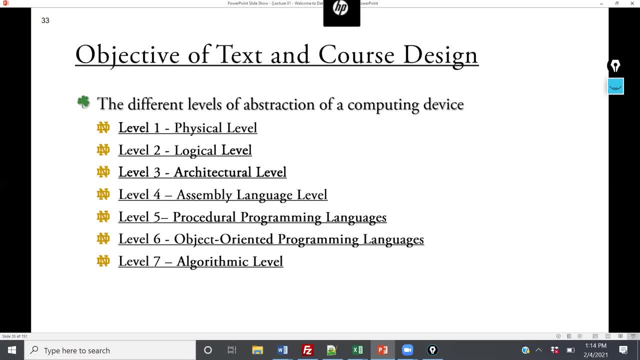 So that's something if you want to take a CMOS course to understand how to fabricate computer 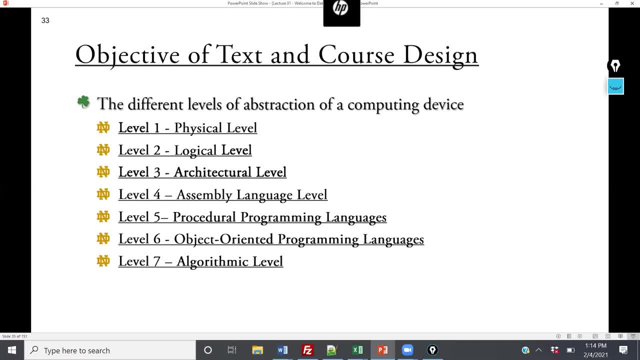 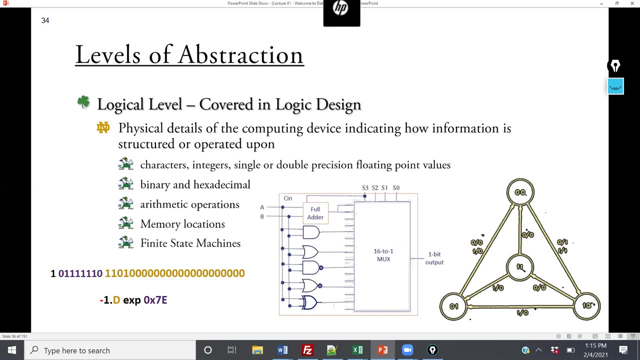 chips, that's what's really going on at that level. Level two is logical level, and you're going to learn a lot about that level in logic design if you haven't taken that class already. If you're taking it this semester or you're taking the labs this semester, you're going to learn a lot about the implementation of the logical level. So let me go to the next slide and show you the logic level. So logical level is things like creating arithmetic logic units, being able to take that physical level and turn it into things like AND gates and OR gates, which will be able to make decisions. And what I have here, this is a one-bit arithmetic logic unit where I have two inputs, and what are known as select inputs. And what those select inputs do is they say, all right, I'm going to calculate AND, OR, addition, subtraction. And based on these selections, you're going to select which one goes on the input of a multiplexer. 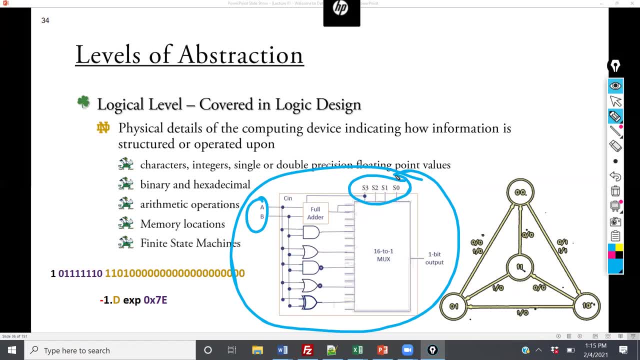 Now, that's really deep down, but what that's going to help you do is help you understand this idea of a finite state machine. Finite state machine is you start a specific state, and then the user gives you a specific input, and then based on that input, you move to another input. And then you keep doing that, and that's a way of simplifying a program and being able to make it more effective. And so that's kind of one of these ideas of the logic level. So let's go to the next slide. 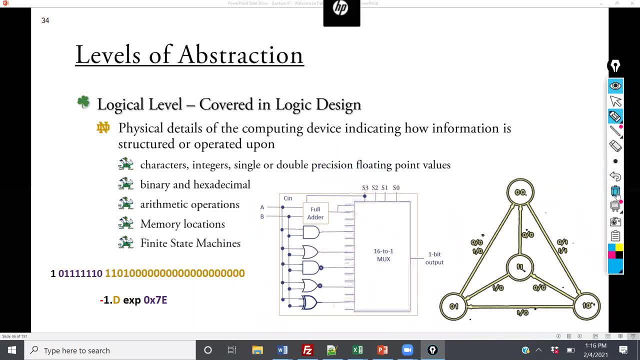 So this is the logic level. Another thing that I have over here at the logical level is this glut of zeros and ones. I've broken them down into three pieces, and this is what's known as a floating point value. So if you've ever coded a float, what's actually going on there is that it's representing a level of precision. So for example, I know from the IEEE 754 standard that that one at the front means it's a negative number. And then I can plug this into a particular equation, and I can actually get a specific decimal point and a specific exponent. And having the computing device structure the data in a specific way, you can come up with a level of accuracy. So integers are accurate because one is always going to be equal to one. 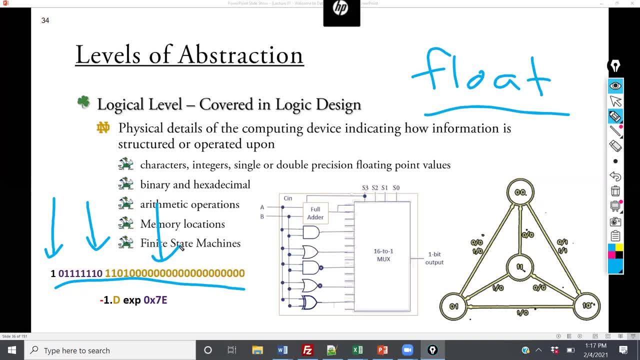 But if you plug in a number, you can actually get a specific decimal point and a specific exponent. So if you plug in 2.2 and subtract minus .1, in our heads, we know that's 2.1. But in a computing device, it's only a certain level of precise, and that makes it hard to be able to make certain decisions, like loops. That's why I typically want to use integer values in a loop, because that can give you an exact value. So understanding how even something like a float is structured becomes really important to be able to implement algorithms. And I'm actually going to show you an 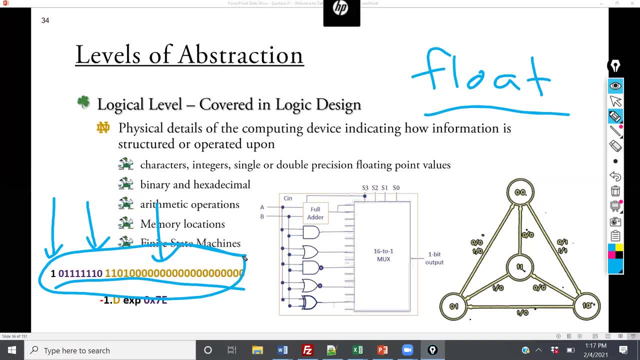 example later this semester of the Ariane 5 space rocket, where improper structuring of floating led to a catastrophe. So this is the idea of the second level of abstraction at the logical level. 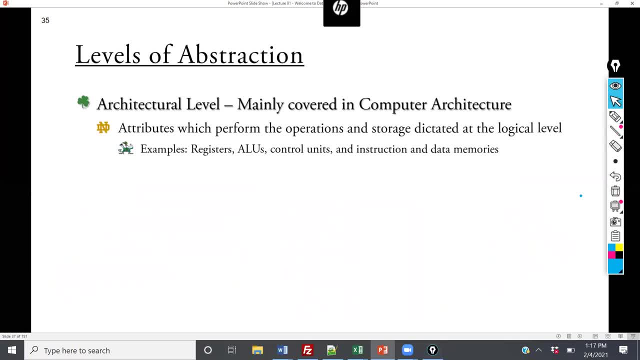 There we go. So the next level, we come up a little more, and we go through this idea of the architectural level. Now, in the computer architecture course, you'll go into a lot more detail about the design and implementation of computer architecture. 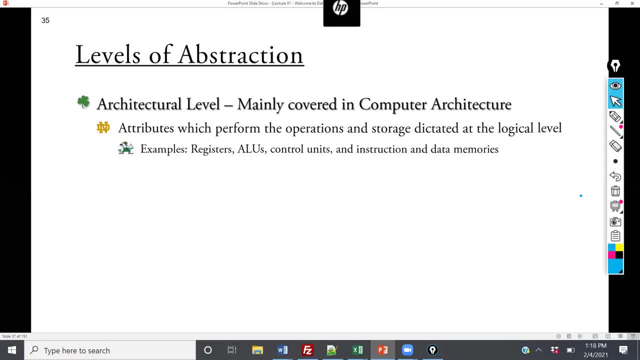 But what I want you to take from this class is just enough to understand what a pointer is, how it works with the instruction memory, and how it works with the data heap. Because a pointer pointing to the data heap is going to be a huge portion of how data structures work in the memory. 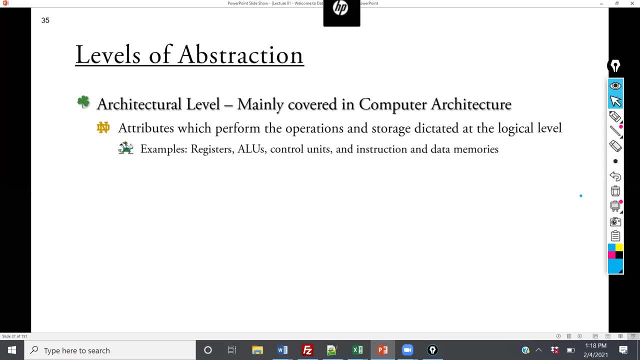 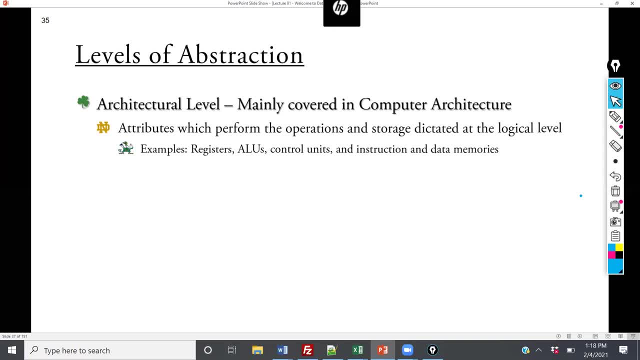 what's going on with the input and output devices. Which is, you will have an occasional operation, which takes a long time. But by doing that long-term operation, it'll actually significantly reduce the time of all of the other operations at that particular data structure. 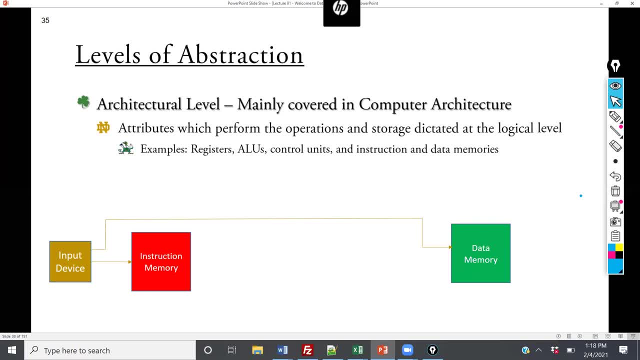 So the general idea behind a computer architecture is that you have some sort of input device, or you have input code. So for those of you who have coded in C, int arg C char star star arg V. That tells me what I need to put in the input, and I know how many command values I have on the input, and I also know how to attain all of them. 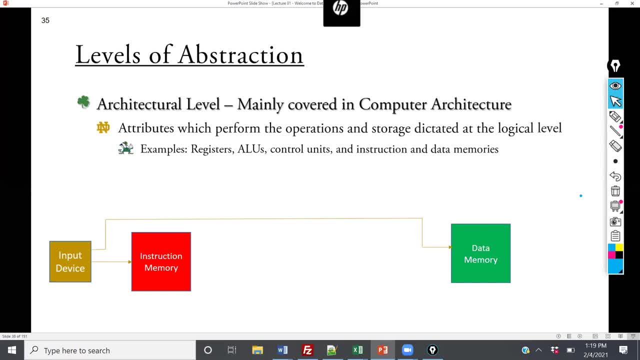 What we're going to learn is this char star star is actually just pointers to different locations in the data memory. And that's what's going on here. 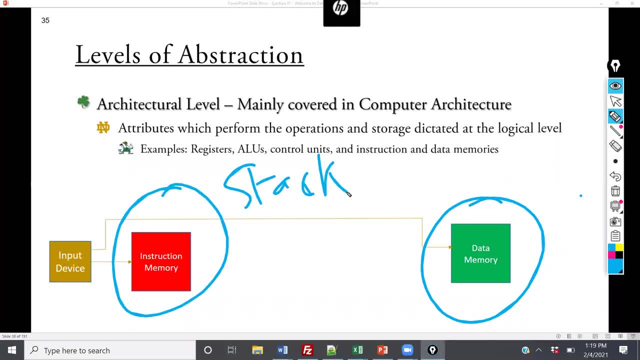 So we'll learn how this contains what's known as the stack, and we'll learn about how this contains the heap. From there, we have registers, fast, efficient, and reliable. The difference is when you turn the computer off, they're volatile, which means that the power goes off, they don't save the information. And also the control memory. 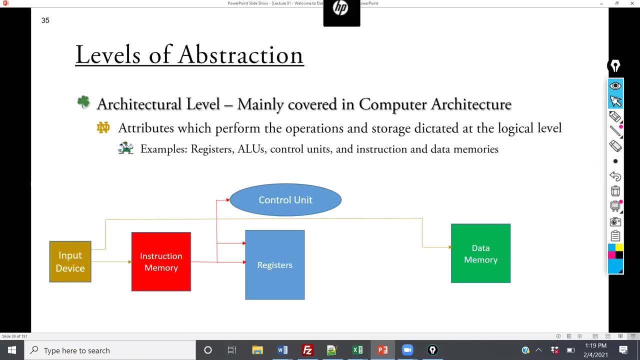 So the control unit sends information to all of the other elements in the computer architecture. So, for example, I'm going to, if I want to do something called a load, and then add, and then a store, that's the fundamental of what a pointer actually is. 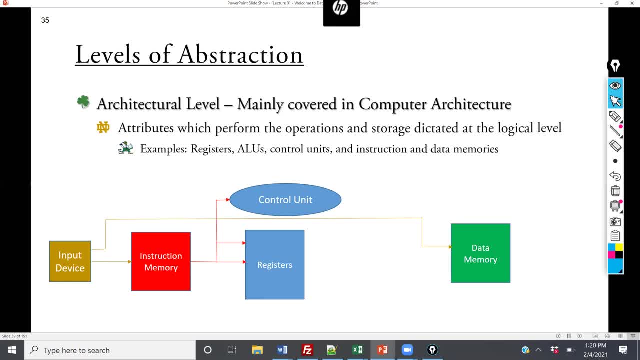 And the control unit helps me be able to dictate what all that is. So in a control unit, if you understand that, that's actually going to be helpful when you take your theory of computing course later and you start learning about Turing issues. 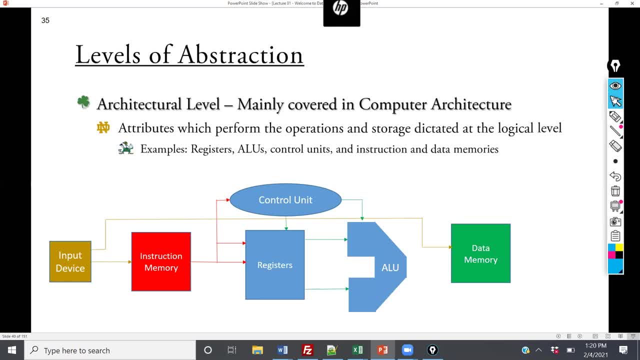 The arithmetic logic unit, I was just describing that in the logical level of abstraction. A pointer is actually an addition. We're going to look at that later. 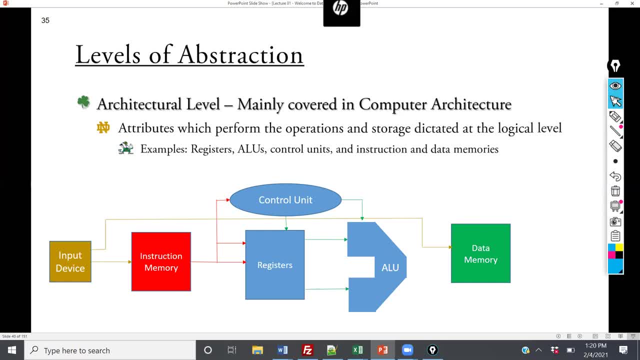 We're going to look at that later. We're going to look at that later. We're going to learn about how the additions contribute to actually putting things into that data memory, or accessing them, and then putting them into the register for fast things. Good thing we got all that brand new duct tape. I don't know what's going on out there. 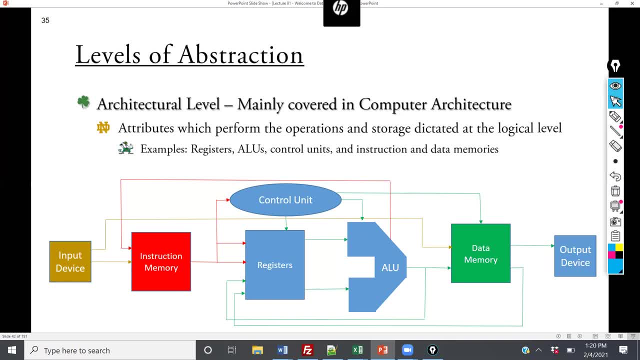 And then at the end, you eventually want to have something on an output device. So a very simple version of a Turing machine, the Turing slot experiment, you had somebody put in a bunch of zeros and ones. There's a person in a box that does a set of operations, and then puts them out on the output. And the person on the output can interpret what the computer actually does. 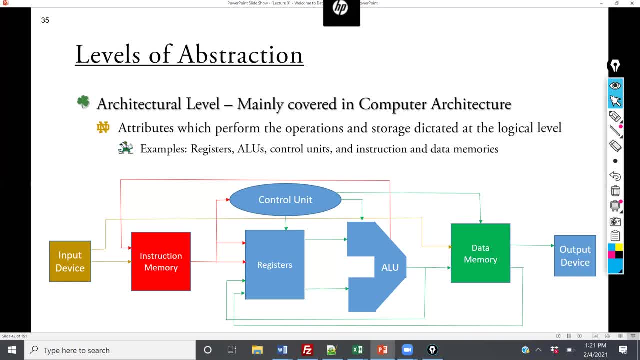 And so that's what's actually going on when you run a program and you execute it. 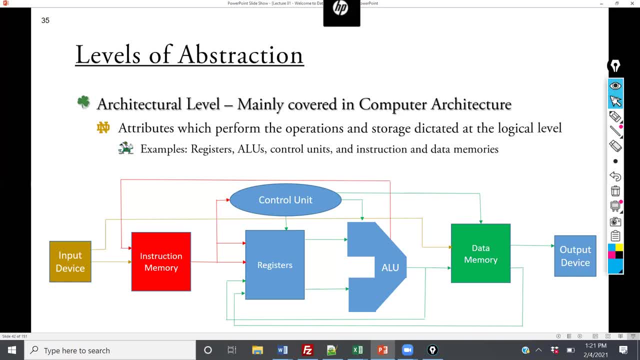 Eventually, you need to have the computing device output the result in a way in which we can interpret. So that becomes really important when you start learning about representation of characters when you ask about it. Does anybody have any questions about this before I continue? All right. 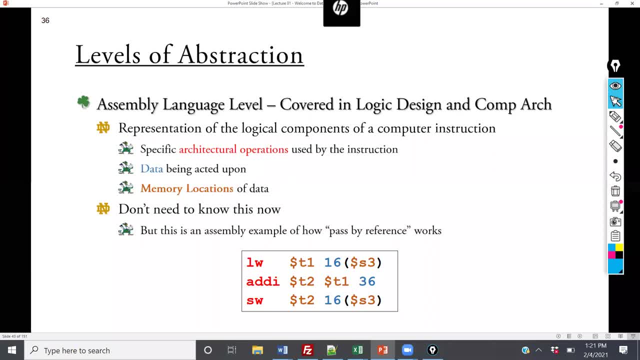 So building up from there, there are several different levels to programming language. The first level is known as assembly language. And assembly language is actually mapping to the computer architecture. So I don't expect you to actually replicate this on an exam for now. But you can do it. You'll see something like this in computer architecture. 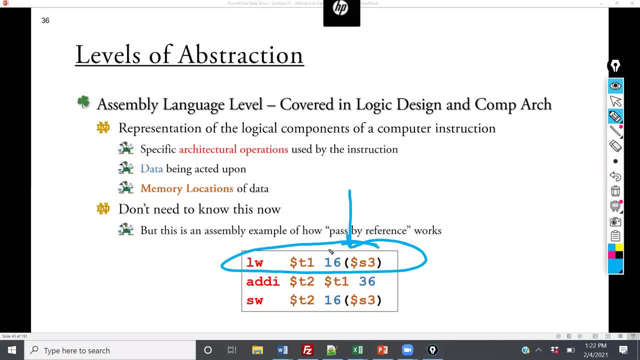 What this line of code means is that I'm going to take something from the data memory and put it in a local register. Next, I want to add the value to that register. In this case, I'm adding 36. 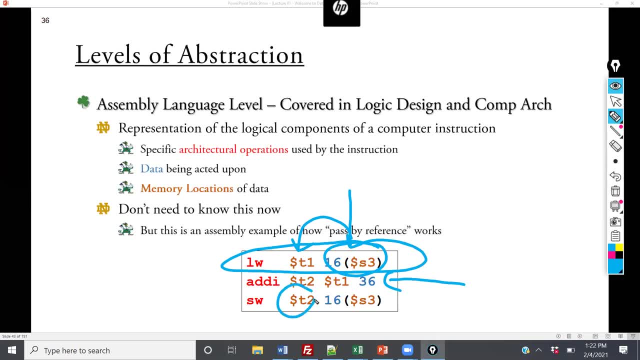 And then SW means I'm going to take that final result and put it in data memory. 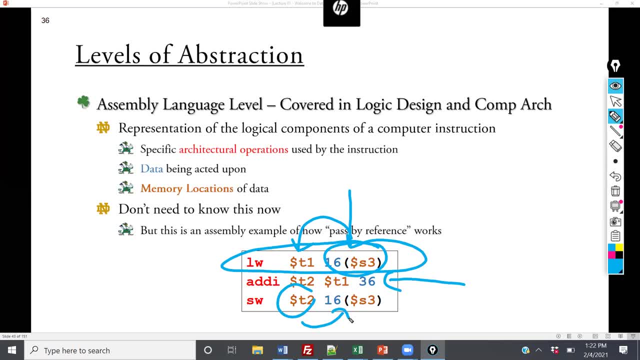 Now, I don't expect you to be able to do that. But that is the fundamental of what has by representation. You have a pointer. 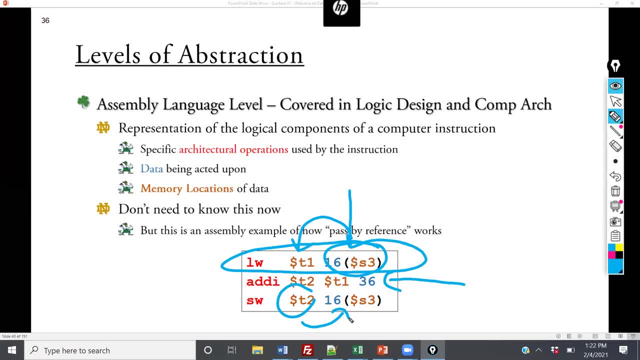 You dereference the pointer. Sorry about that. You take it out of the memory. You perform some sort of fast operation on it. And then you take it back. And that's how dereferencing a pointer works. 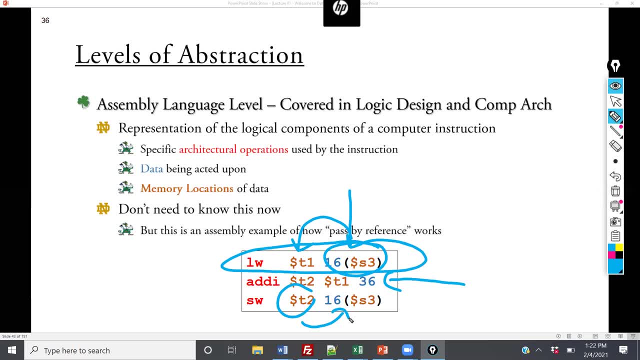 And so we'll understand that. And we'll implement this by learning about void pointers. So you don't need to know this now. 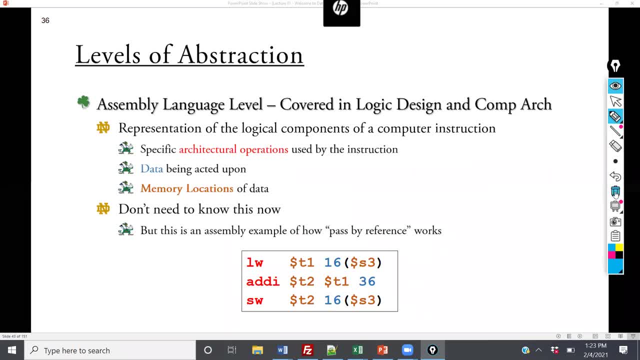 But the crucial thing is that. There's something going on underneath. When you write that code, it sends information. And it's all interpreted by this physical computer architecture. So if you understand how a pointer works and what's actually going on, it'll make your code more efficient. All right. 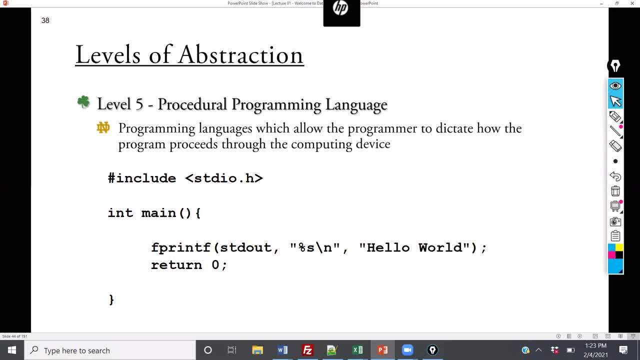 So now we get to procedural programming. Procedural programming is. It's at a higher level. 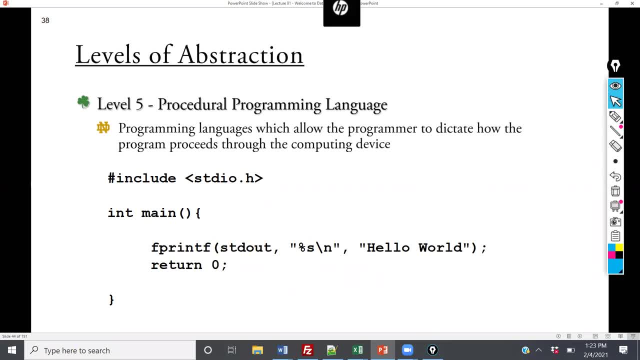 Than assembly language. But the whole idea is that you are telling the computer precisely what to do. 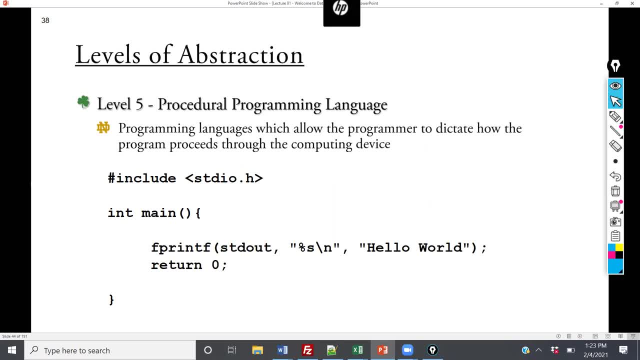 So, for example, this is a hello world program in C. And the difference here is you have some standard output. So that's the terminal. 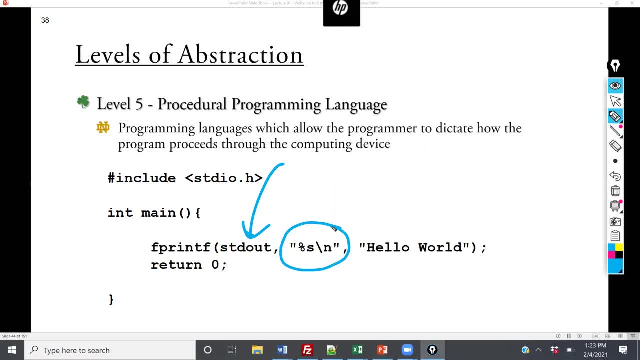 And then what you're actually doing here is you're allocating memory on the data. And you're saying, I need to allocate some memory. And it has to contain characters that represent hello world. 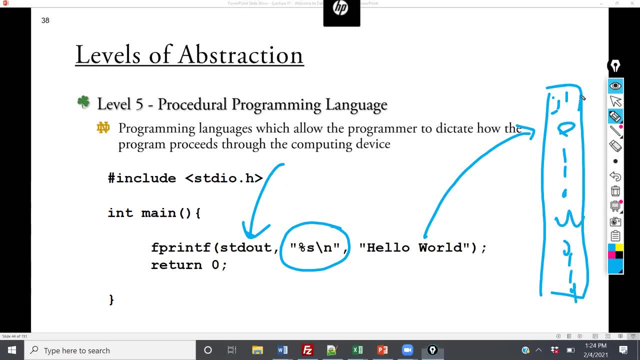 And then you will print these to that output. 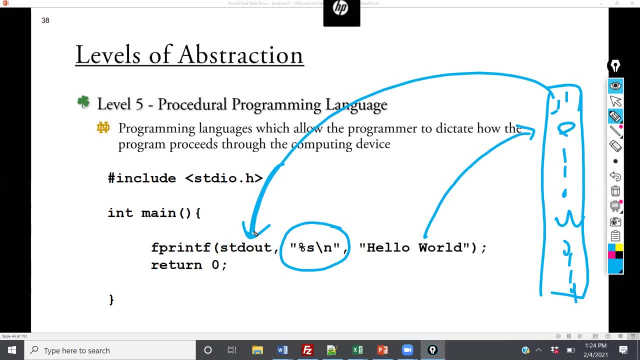 So we tell the computer, create a register that is pointing to a location in the data memory. The data memory contains binary representation of characters that represent hello world. And then we have to somehow access them and print them to the output. 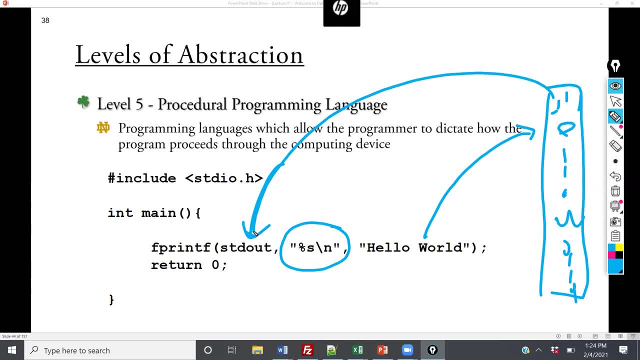 So you can see this idea of procedure. It's working through. And you're thinking about it. And you're telling the computer exactly what to do. 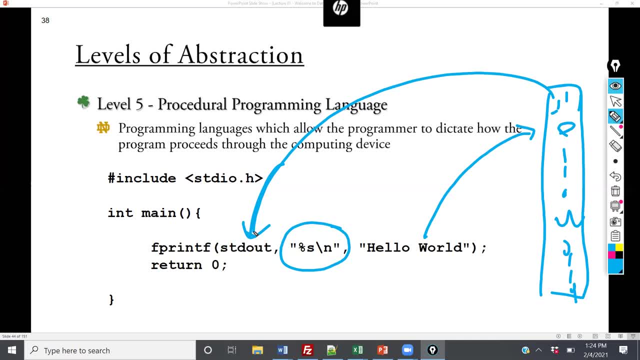 And so some people, particularly, you know, I'm a computer engineer by trade. A lot of people are computer engineers who really like to deal with the lower level programming. 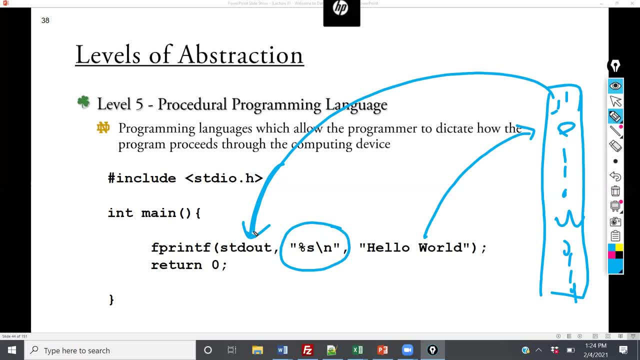 They really enjoy coding at the C level. And C++ or object-oriented programming is a little different. I see some people scribbling down notes. Does anybody? I'll wait for a split second. 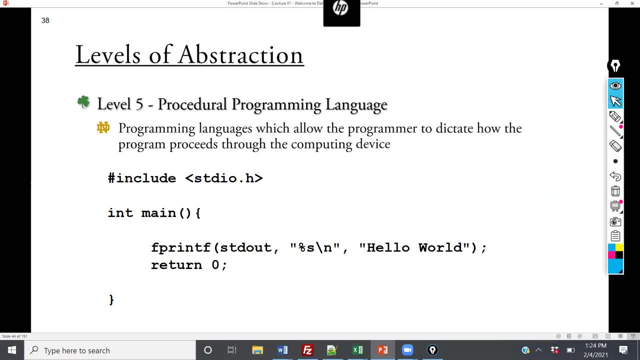 Oh, you don't have to stop on my behalf. Does anybody have any questions before I hop on? 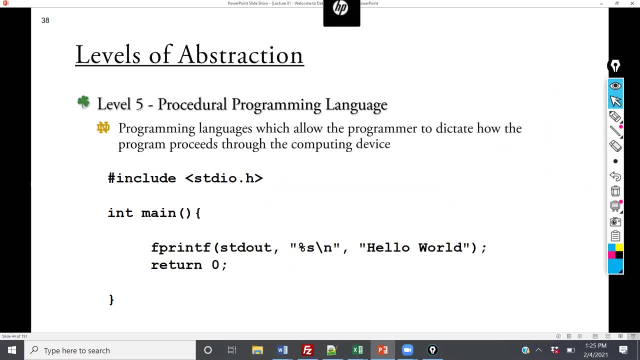 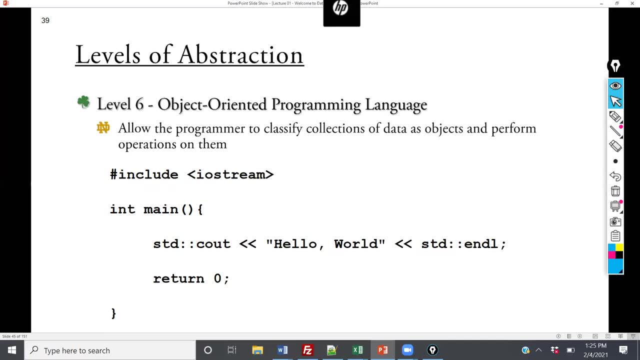 Do I do that? If I see people still scribbling down, I'll hesitate for a moment to let everybody catch up. 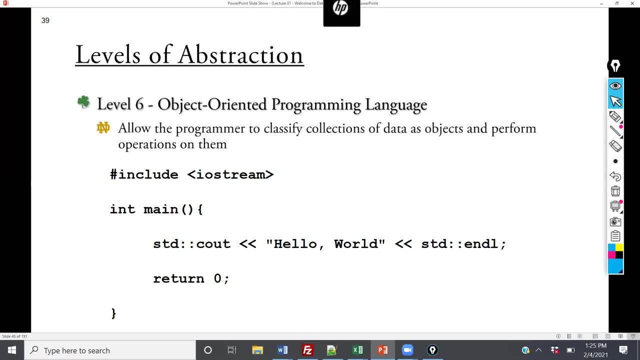 This code that I showed you before that I claimed has two pointers is object-oriented. 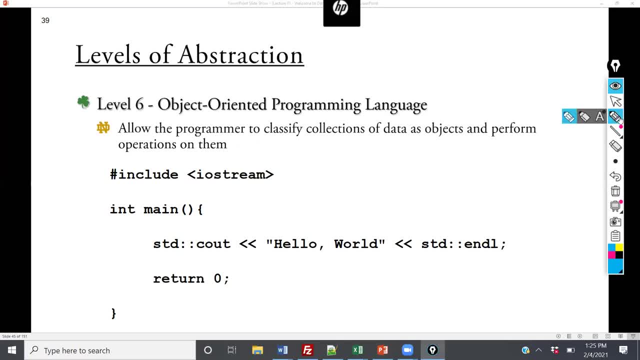 Standard C out tells me where the output is. 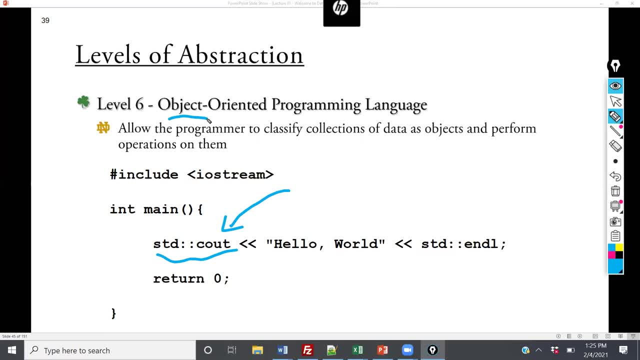 But it's also what's known as an object. It treats hello world. World is some sort of object. 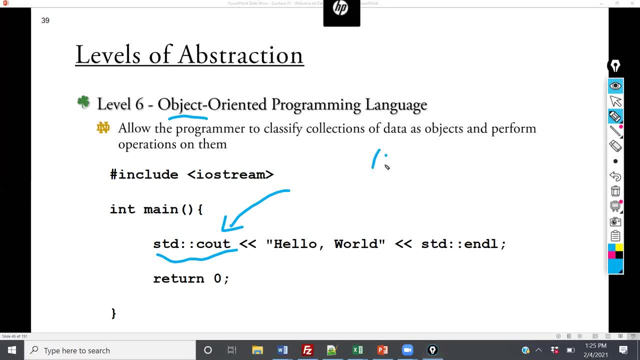 In the C version, I had to indicate with an output specifier. This percent S means it was a string. 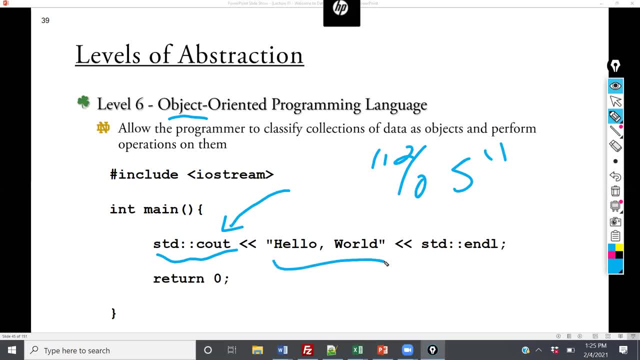 What we're going to be able to do in C++ is I could put an integer here. I could put a float there. 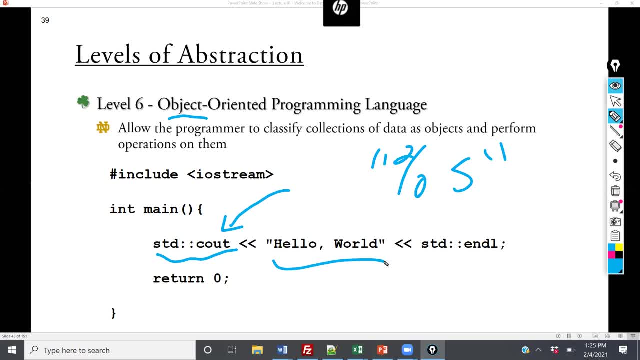 I could put a string there. And C++ will treat it as an object and will take in anything, any type of object. 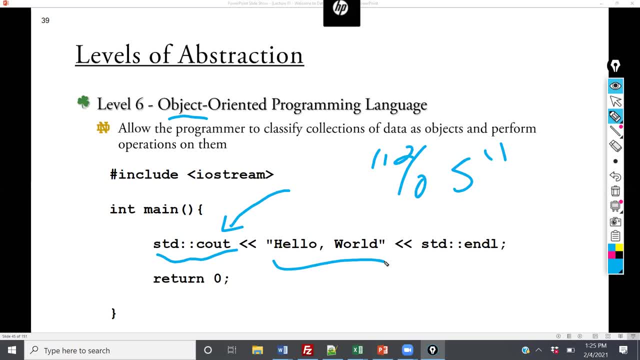 And that process is known as generosity. Where you can do something generically. 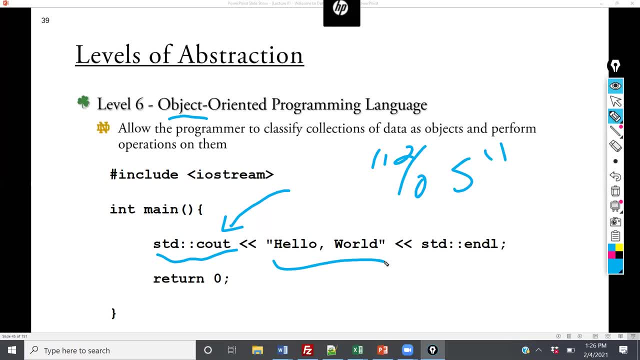 And so here, we put in a string. And the object says, okay, it's a string. I'll do the work for you. 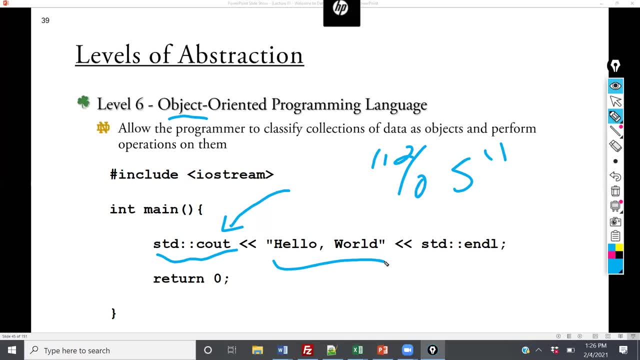 So it's a higher level than procedural programming. And the objective of object-oriented programming, I mentioned this a little earlier, is to have things work as though they're real-world type objects. 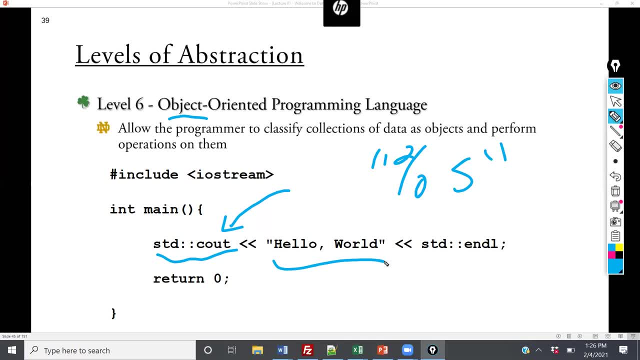 And to abstract some of the complexity away from the program. So one of the important things about data structures, of course, is making this transition from procedural programming. In C, to object-oriented programming. 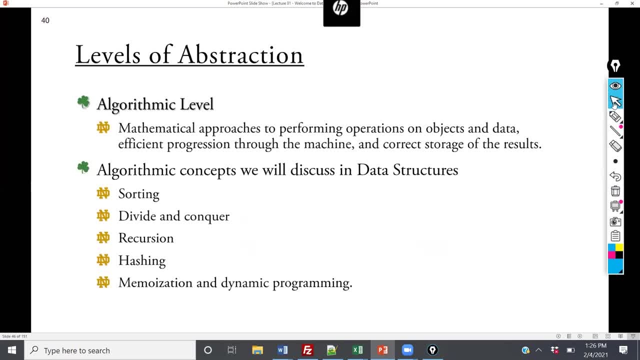 So now at the algorithmic level, we're going to go into a few types of algorithms in this course. We're going to go into things like divide and conquer. We'll learn some sorting algorithms. We're going to go into a lot more detail about recursion and something specifically called memoization, which allows us to be able to do recursion a lot faster. 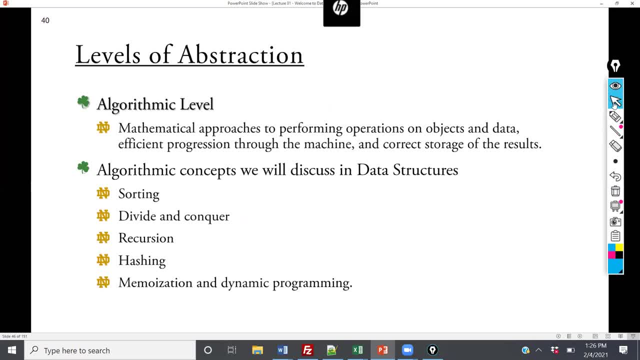 We'll learn about hashing in order to be able to do speed. And then dynamic programming, which is a way of taking previously calculated solutions to be able to develop a new solution. 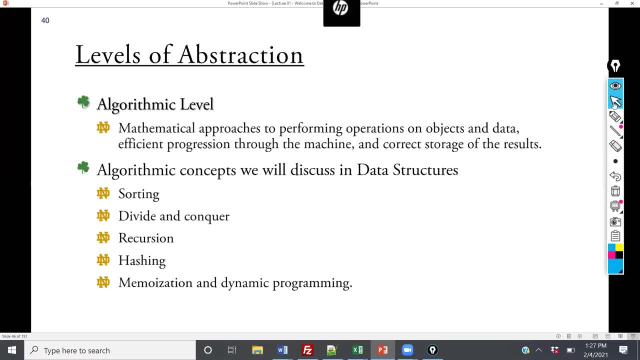 So, for example, the Fibonacci sequence. Fibonacci sequence, we have the first two numbers are one and one. And then you just add the last two numbers. So one and one becomes two. Then it's two and one becomes three. Three and two becomes five. 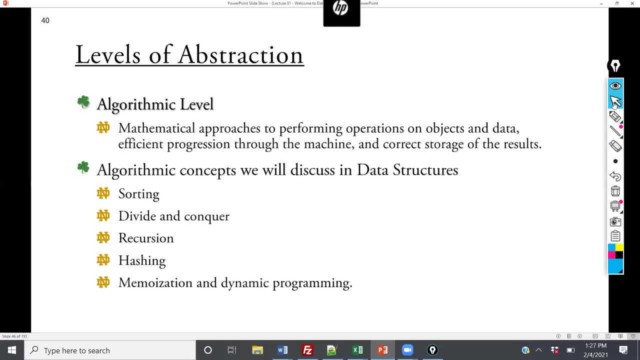 Five and three becomes eight and so on. So what you're just doing is taking recently calculated results to develop a new result. 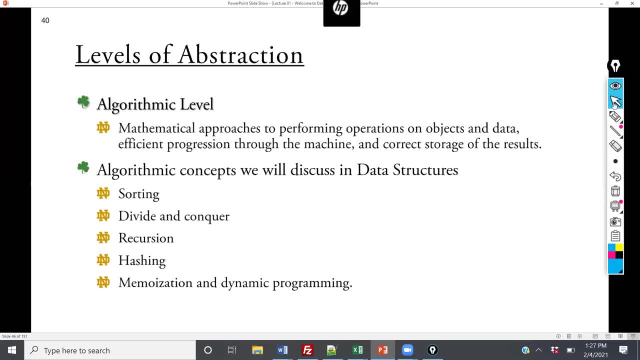 What you don't have to do is you don't have to go in every single time and recalculate everything. 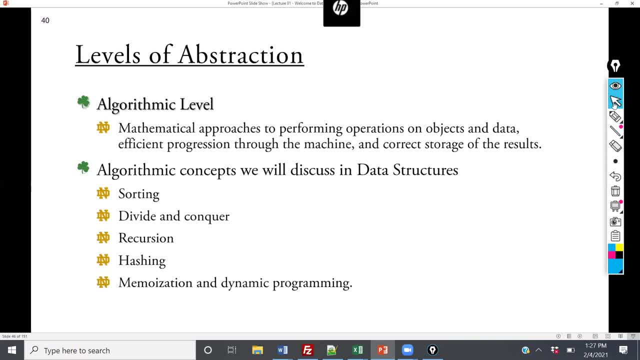 So taking advantage of data structures in this kind of algorithmic approach will make your code run more efficiently. 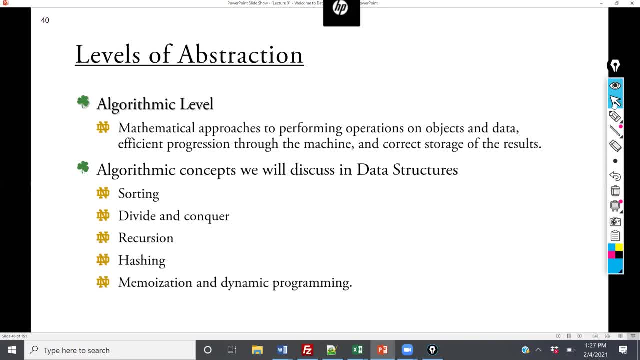 And so there are tradeoffs. So hash tables, you can access them in what's known as bagel of one time. 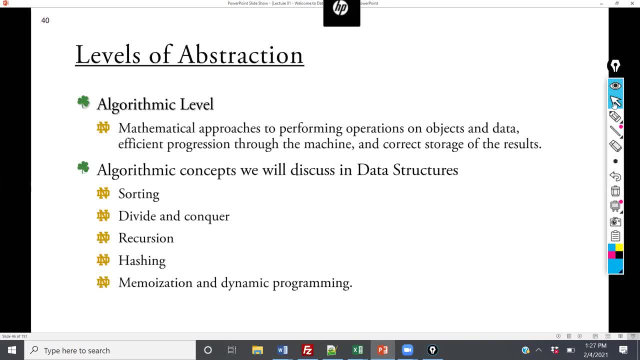 So this is constant. Every single time we do that, it's constant. 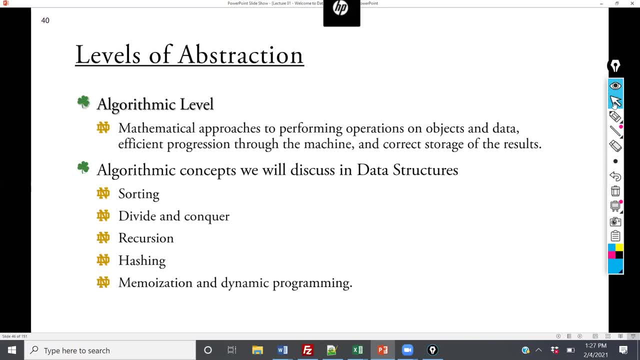 However, in order to do that, we have to implement a lot more memory, which means we have to implement more memory on the data stack. 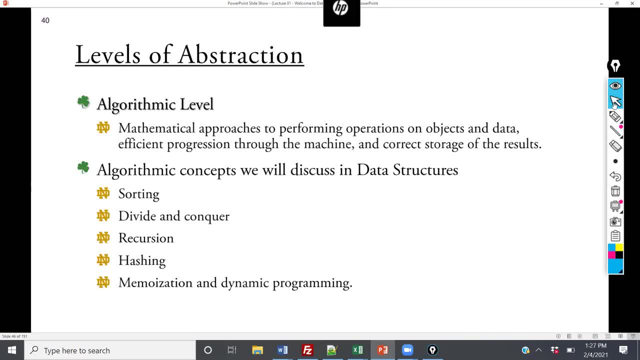 So there's tradeoffs to these different approaches and understanding all of that all the way from the logical level all the way up to this algorithmic level will really strengthen your approach as you become a programmer, computer scientist, computer engineer, or whatever it is that you plan on doing with what you learn in this class. I'm sorry, did you have a question in the back? No? All right. 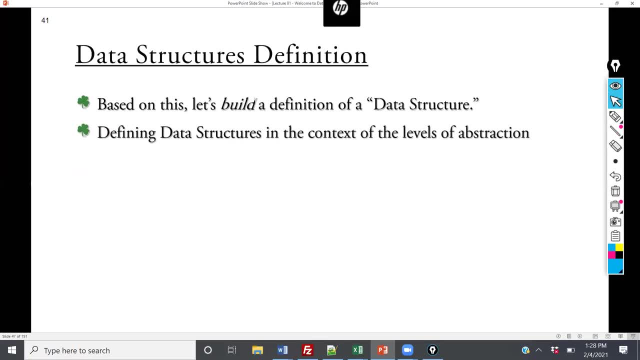 So based on this discussion, what I want to do is I want to do a little bit of a study. I want to build a definition of data structure. I will not ask you to replicate this on the exam, but I want to kind of work through it and see if what I've been talking about so far makes sense to you. And if it doesn't, please do not hesitate to ask any questions. 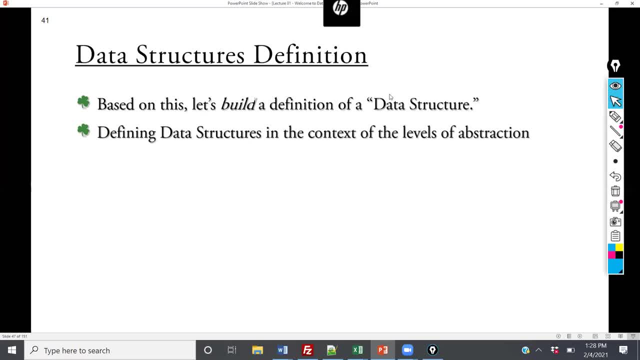 So defining data structures in the context of levels of abstraction. 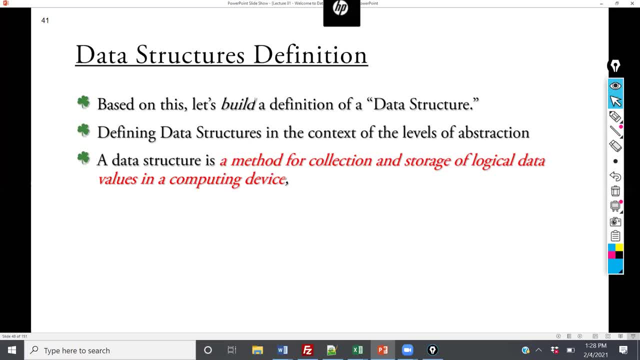 First, I want to say that a data structure is a method for collection and storage of logical data values in a computing device. So we saw one such example with Hello World. The data is characters. I have a certain amount of characters. And I need to collect them and store them somehow. And I also need to be eventually able to access it. So I need to be able to know how to do it efficiently. I know how to be able to do it reliably. 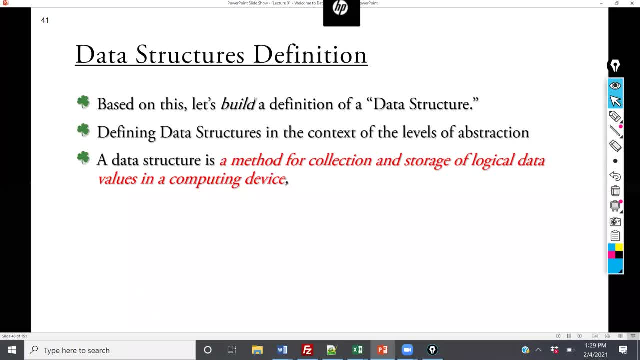 And then I need to somehow go through and be able to get that. Because in Hello World, that eventually goes to printing the output. To the terminal. 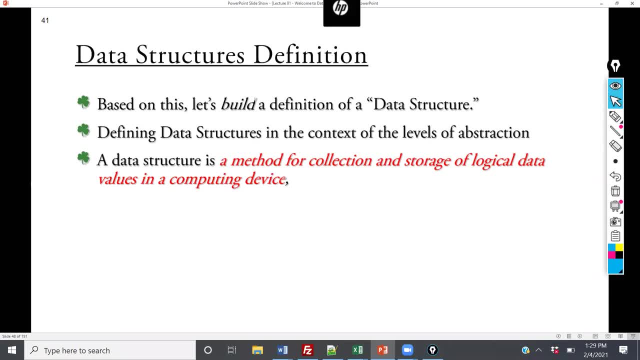 Does that make sense so far? I'm going to give everybody a moment to jot that down. 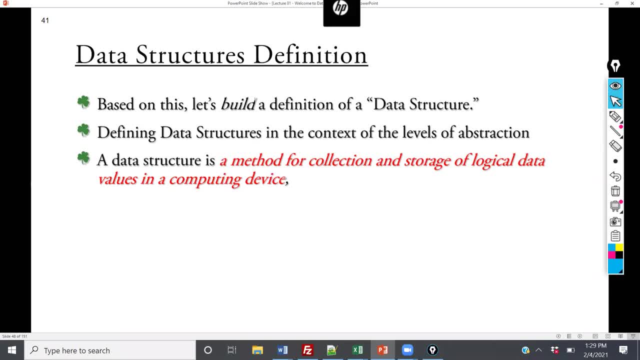 So let me repeat that for you. The first part is a data structure is a method for collection and storage of logical data values in a computing device. 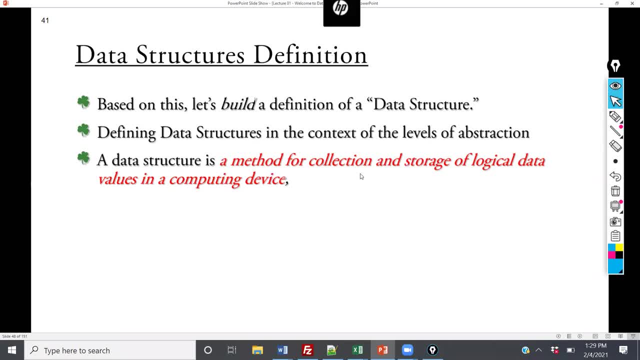 While you're all writing that down, I'll check to see if there are any questions in the chat. So for those of you who are online, I will regularly check the chat. 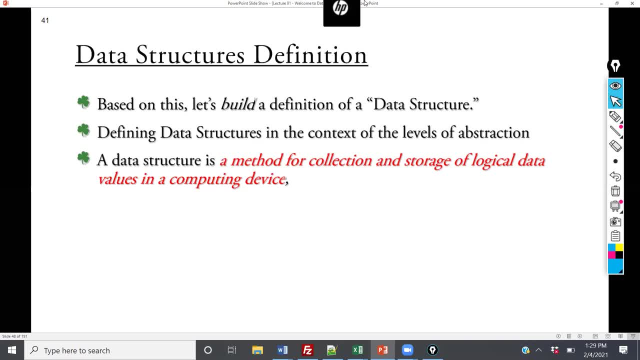 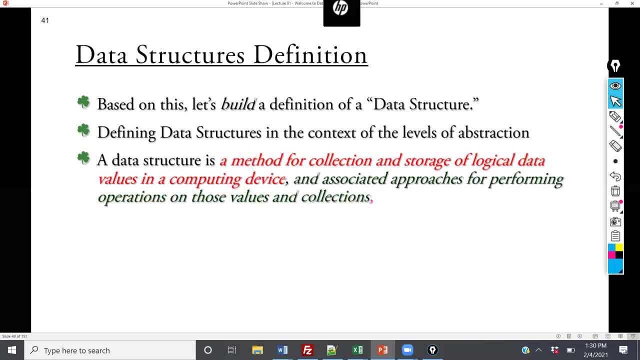 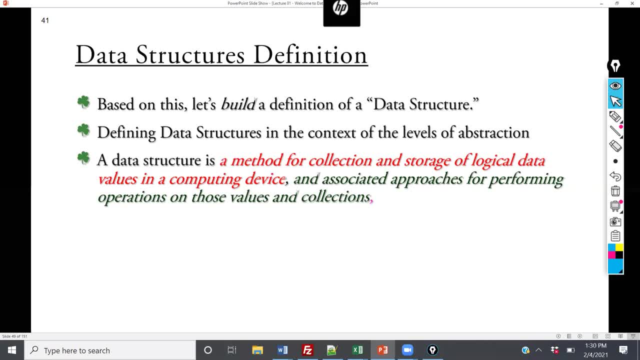 Okay. Okay. Okay. Okay. Okay. Okay. Bye-bye. Bye-bye. 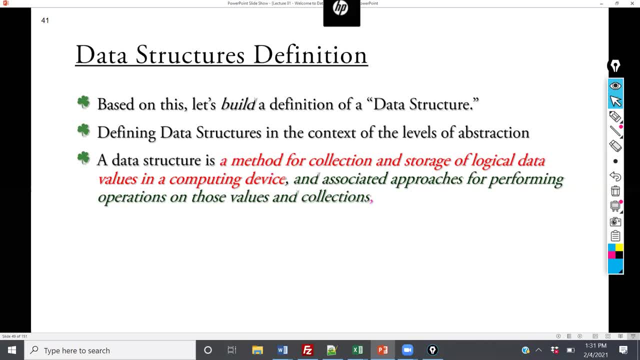 But in general, we have to say, okay, well, if I actually delete an element from the hash table, that screws up some of my algorithms to be able to seek and find those values. 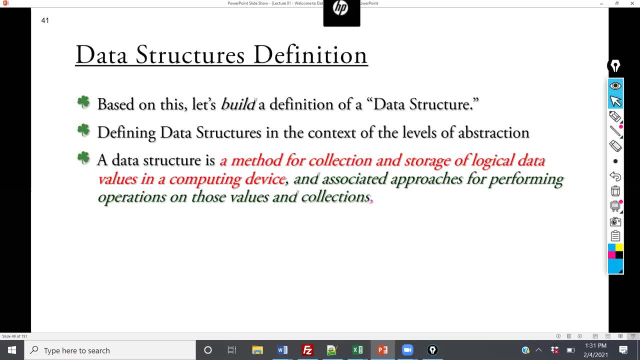 So, we have to bear all those things in mind. So, the second part of the definition, and associated approaches for performing operations on those values and collections. 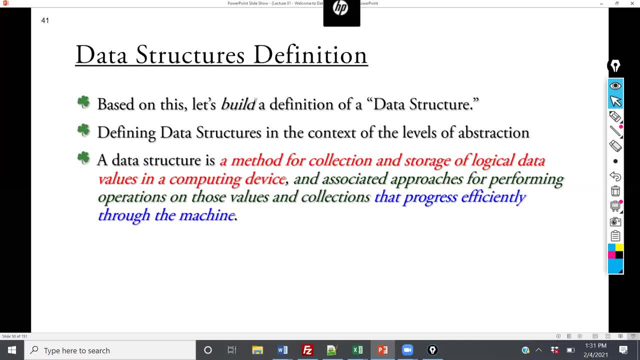 Okay, and now the last part, that progress efficiently through the machine. That's where we're going to start tying in this algorithms portion. 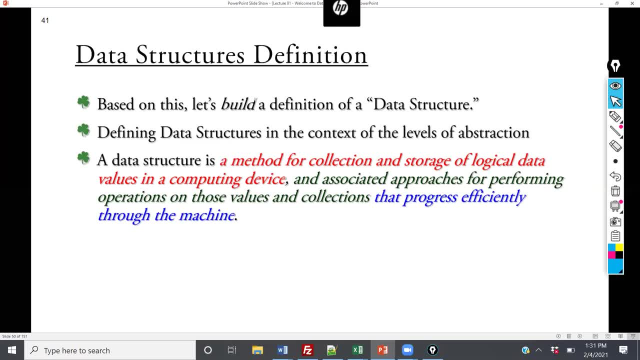 If I want to reduce memory consumption, but I still need to have some sort of relatively fast access time, a binary search tree is a good choice. Hash tables are accessed faster, but consume more memory. Trees consume less memory, but are not as fast access. 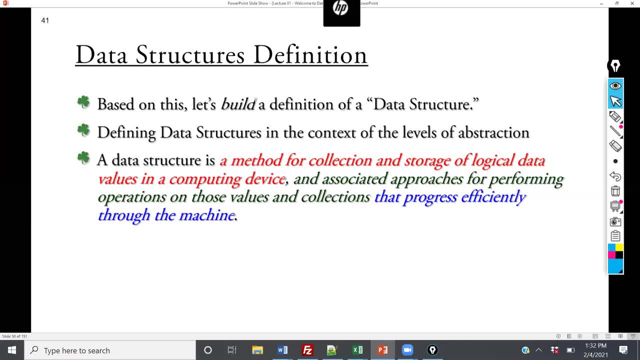 If your customers, like, for example, let's say perfect NASA, right? So, NASA, when you're putting an embedded system onto one of the Mars rovers, weight is a premium, which means you have to be as efficient with the computer as possible. You can't be, like, ask for a larger memory chip, because you have to be very efficient with it. Also, we don't want to have a segmentation fault on Mars, because we can't just send somebody out to just reboot the computer, right? We're literally millions of miles away. So, we have to be efficient and reliable. So, we have to think about good trade-offs and being able to run, you know, reliable. Reliability is very important. Low memory is very important. 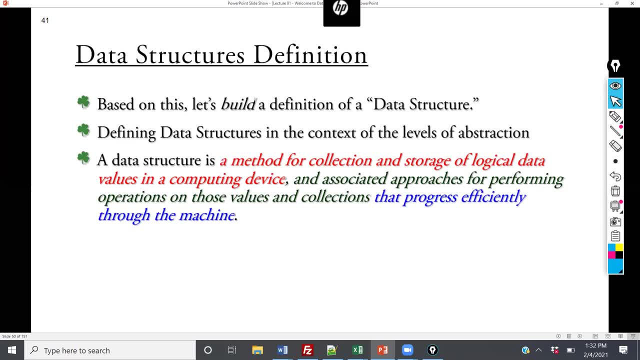 Speed is not as important, because even though it's going to do something, it's still going to send it back millions of miles away, and it's going to move the Mars, the Mars rover is going to move only a few feet at a time. So, speed is not as important as memory. 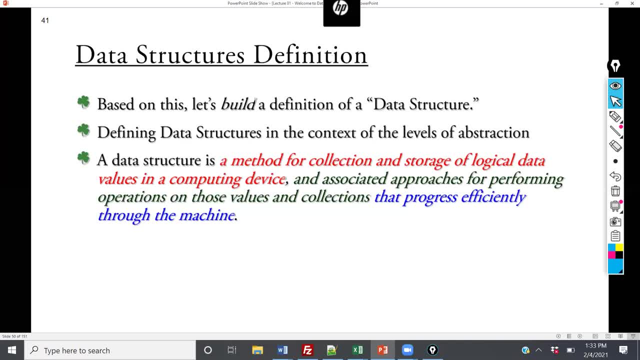 So, you're going to make those kind of choices based on what the customer wants, what is required for your specific environment. So, I'm going to read through the definition one last time, based on the levels of abstraction. 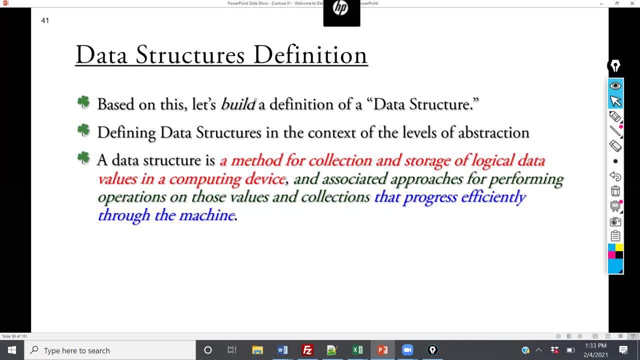 A data structure is a method for collection and storage of logical data values in a computer device. So, that's a logical level and the architectural level, and associated approaches for performing operations on those values and conditions. 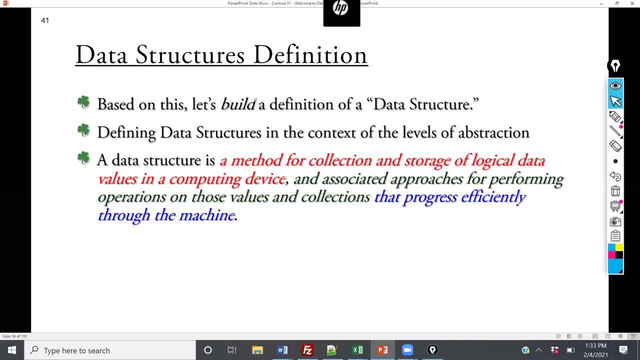 And now, we're talking about procedural and object-oriented level. And then, we have the last part of the definition that progresses efficiently through the machine. So, now, that's your algorithm. 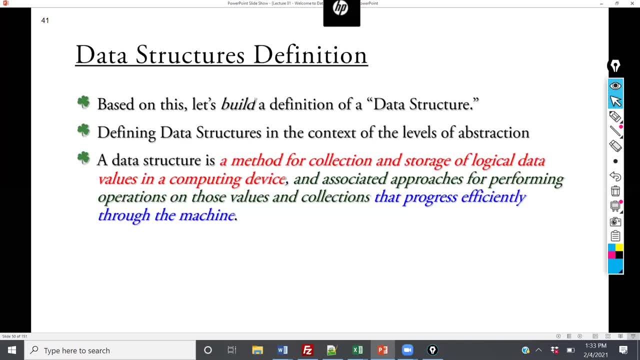 Does anybody have any questions about that? Not even Erin. That's impressive. She really knows her stuff. All right. 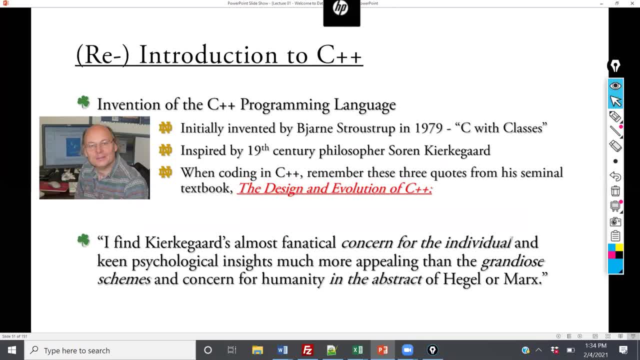 So, some of you may know C++. A few couple of you may not. 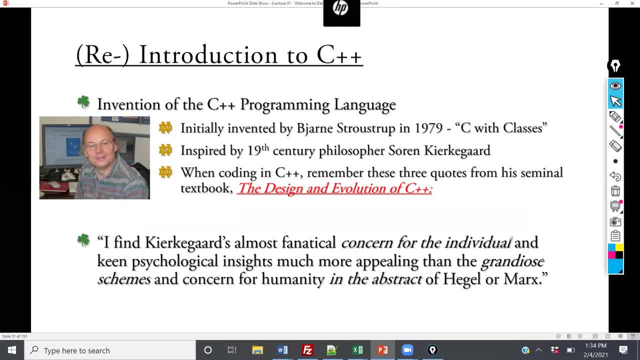 So, there's a reintroduction to C++. So, this picture here is of Bjarne Stroustrup. And he is the. . . . . . . . . . . . . . . . . . . . . . . . . . . . . . . . . . . . . . . . . . . . . . . . . . . . . . . . . . . . . . . . . . 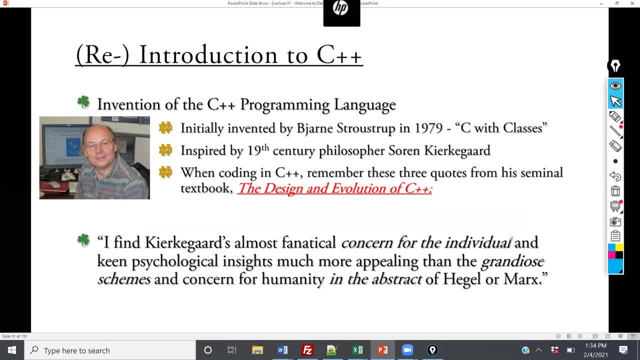 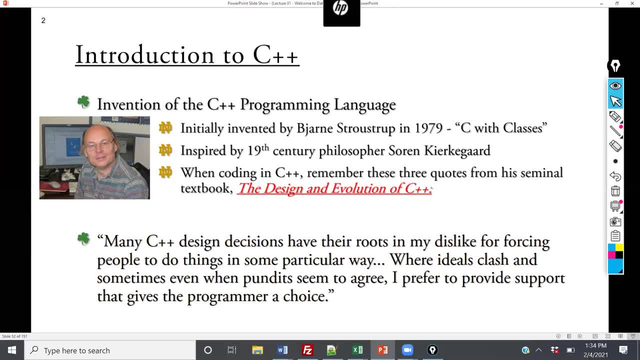 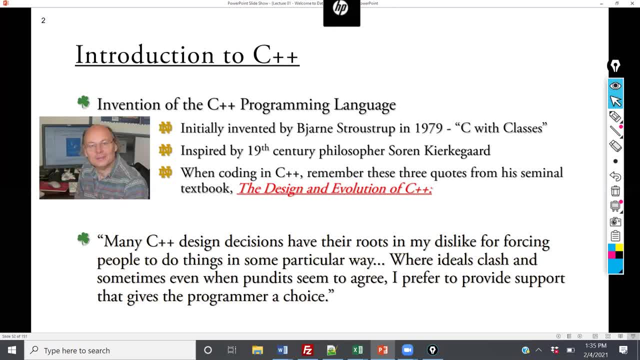 sometimes even when pundits seem to agree, I prefer to provide support that gives the programmer a choice. Generosity, being able to write a data structure that can store integers, characters, strings, a class that you create. 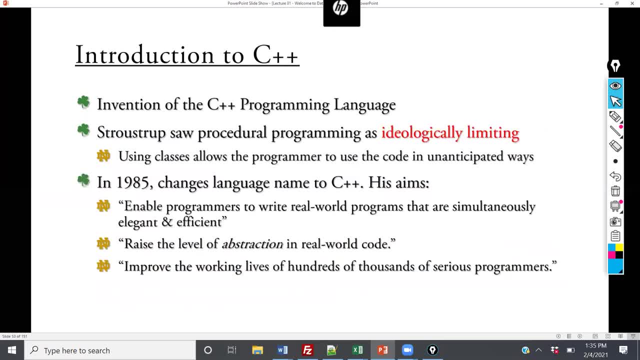 That's the goal with C++ and object-oriented programming. So he changes the name to C++, 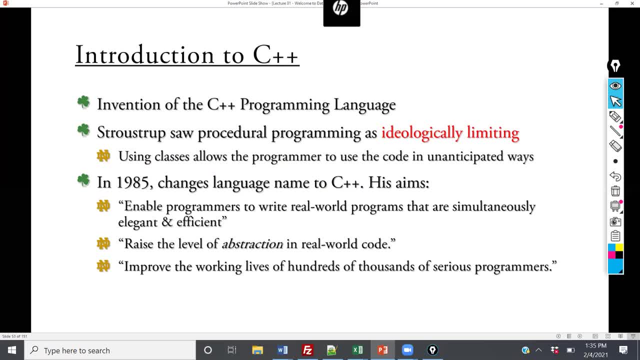 and the goal is to enable programmers to write real-world programs that are simultaneously elegant and efficient. 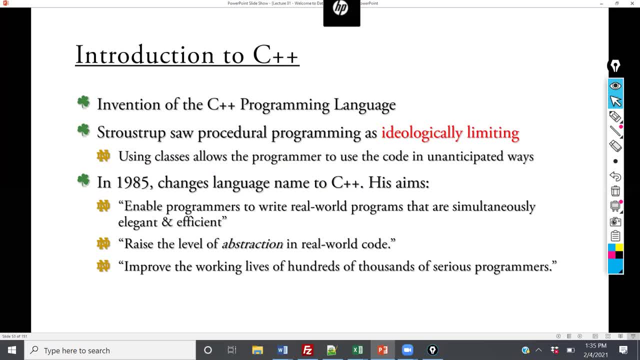 So if that's a philosophy I want you to take away in terms of what data structures is, elegant and efficient. 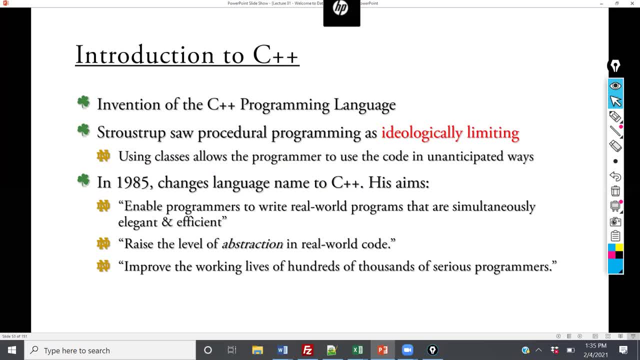 Is the code efficient? Can it be, is it easy to interpret? Is it easy for other people to use? So he wants to, his quote here is to raise the level of abstractions. 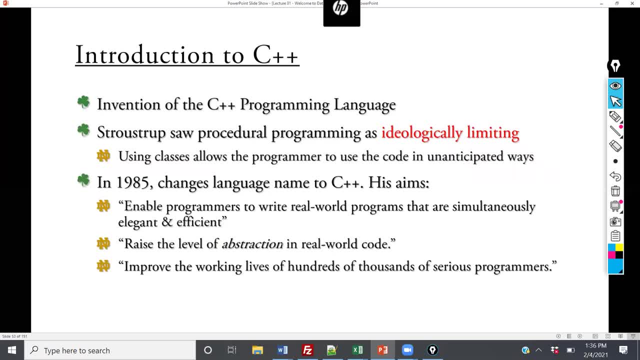 We've gone from procedural to object-oriented programming. And I had that quote in red there 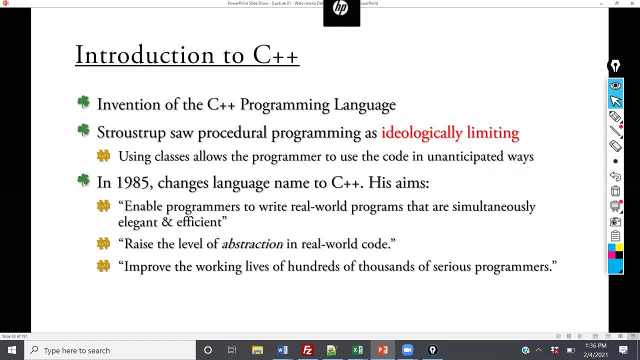 about ideologically limited. The reason I have that highlighted and I present it, 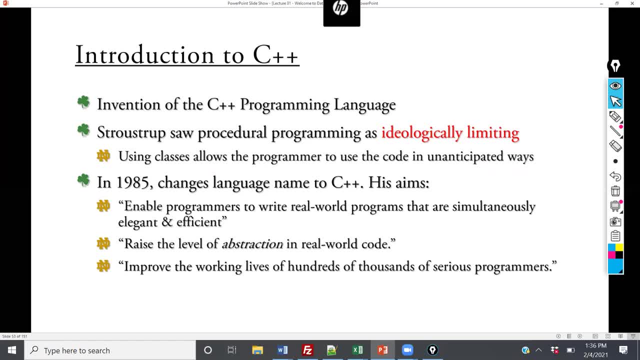 I'm gonna show you the data structures is that transition from C to C++. 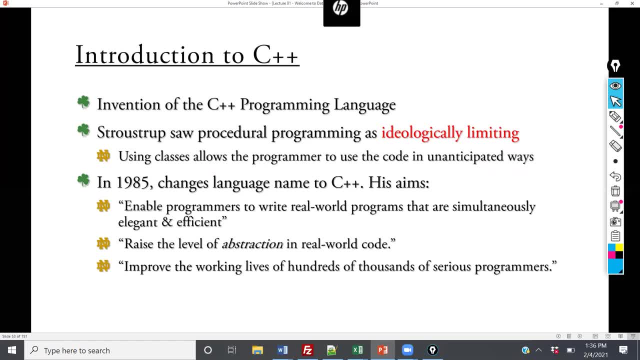 If you're kind of having an initial hard time kind of visualizing and understanding C++, that's perfectly okay. It's a different type of philosophy. 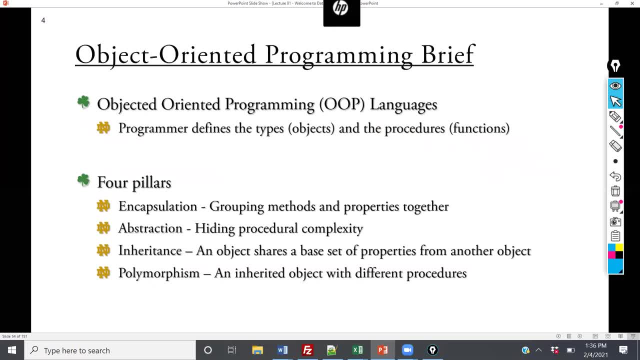 As, okay, so moving from C to C++, this idea of object-oriented programming, of being able to take objects and put them into code, has four main pillars. One is encapsulation. 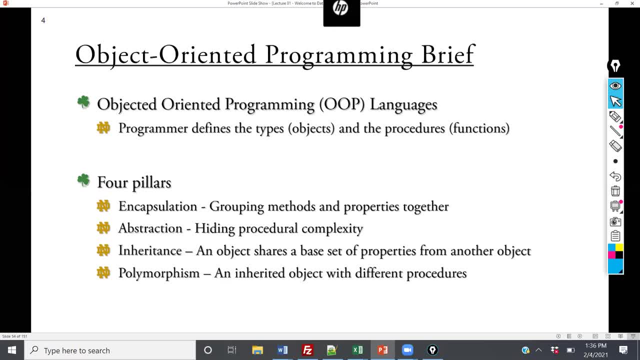 For those of you who take the code in C++, if you've, let me ask you a quick question. 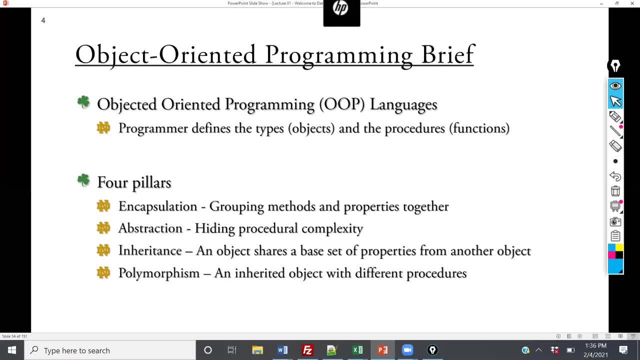 Those of you who take fundamentals with Dr. DeWallen, do you all cover classes at all? No, okay, so the idea of a class is I could say class person. I'll actually go into more detail about this in future slides. 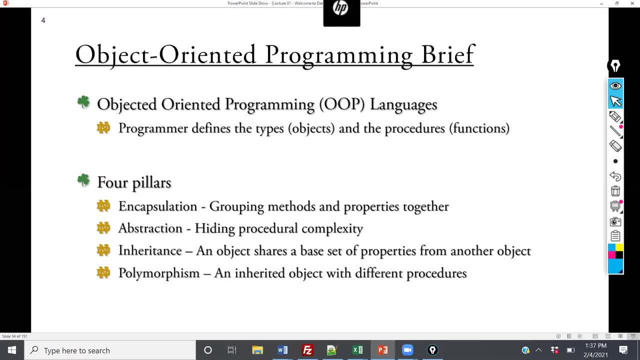 I can say a person has these specific characteristics and I can perform these specific operations. When I define a class, I can encapsulate that so every single time I define person, it has those specific characteristics. 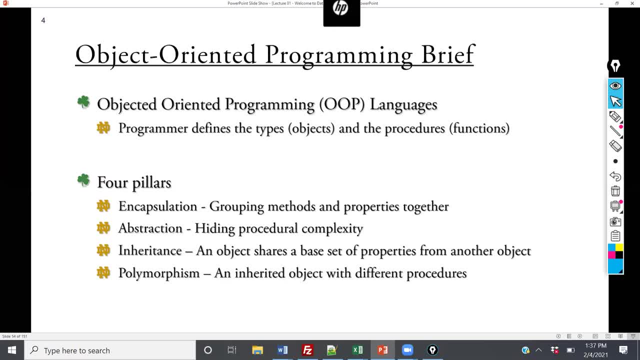 Second is abstraction, hiding procedural complexity. One of the goals, if you build a really good class and you build a really good data structure, it should be really easy to implement it. 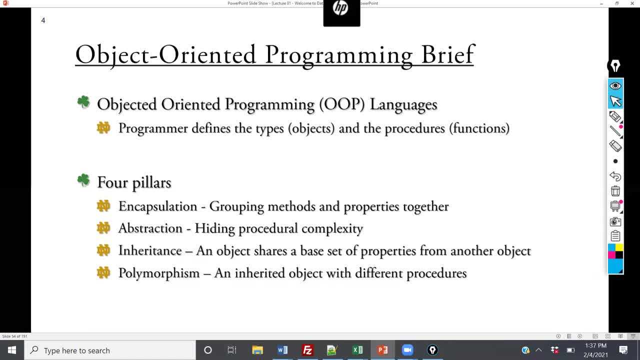 The more complicated the data structure, the simpler the algorithm. 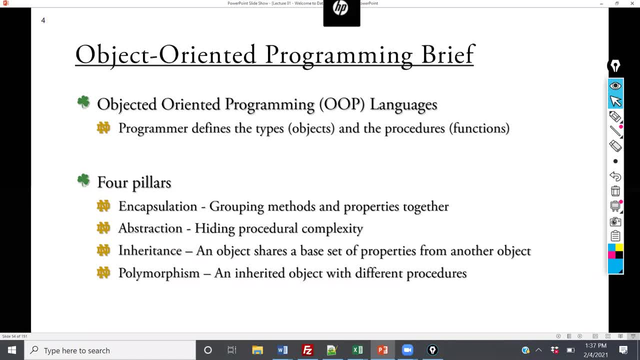 If it's easy for someone to use your code, it's well abstracted. They only have to write, call a function, call a class method that's the equivalent of a function in the class, and it does something that makes them happy. They don't have to deal with what's going on underneath the hood. That's good abstraction. 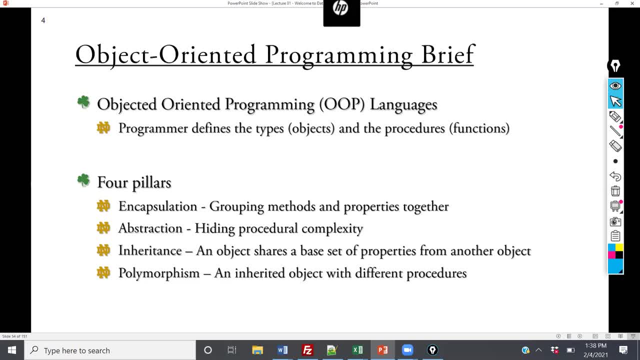 So inheritance is the next one. Inheritance means that certain classes have the same common principle. 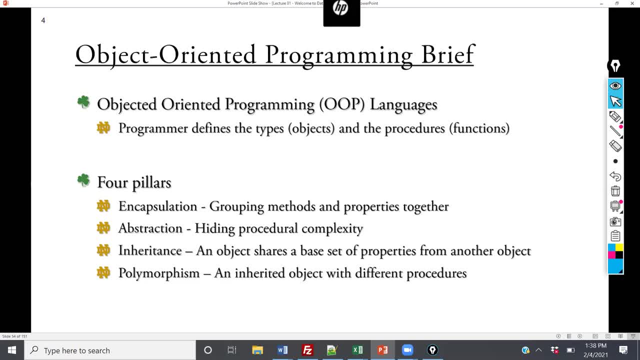 So everybody who's at Notre Dame, whether they're faculty, staff, or a student, they all come here, we all have IDs, we all have parking, there's certain things that every single Notre Dame person has. But then you get the students. Students have a dorm. 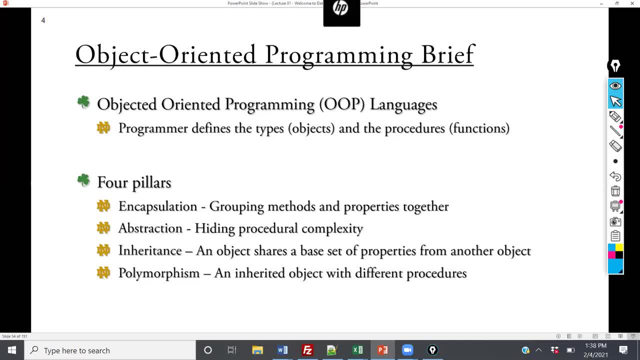 Faculty, like me, have no business over there. So I don't need anything involving a dorm. 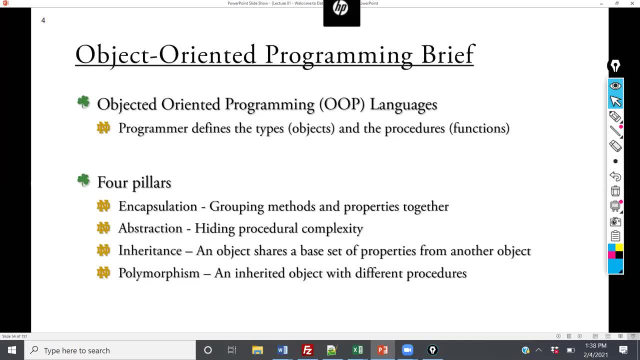 I need to have where my house is, right? And then I have information about what kind of salaries, things like that. 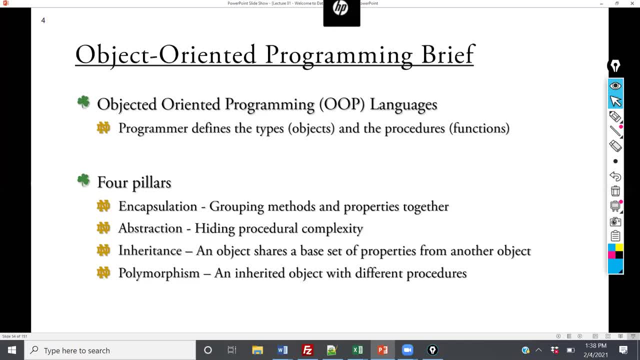 You have things like GPA. When you have different types of the same fundamental object, that's known as polymorphism. 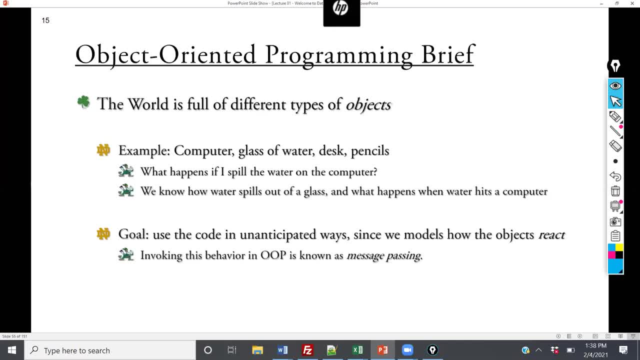 So let me go over an example of this idea of objects and encapsulations. 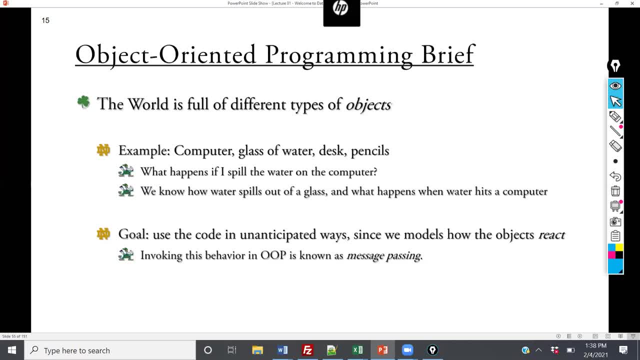 The world is full of objects. Let's say I had a glass of water, a computer here, and some desks and pens. 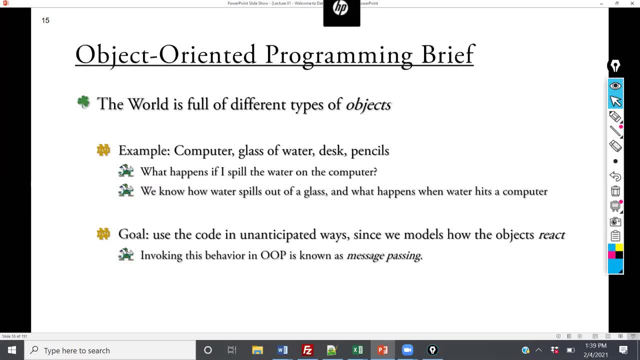 I know what will happen if I turn the glass of water over. And I also know what would happen if water hits glass. So the idea of object-oriented programming is I should be able to write code that outputs a method, spills water, and has it operate well with a computer hit with water, 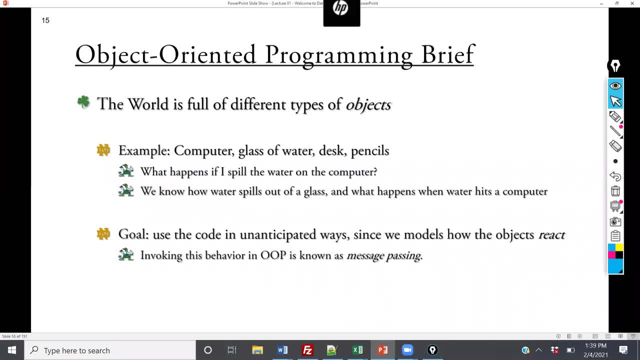 where I don't have to actually write another big, important, large code that has to somehow tell them how to interact. 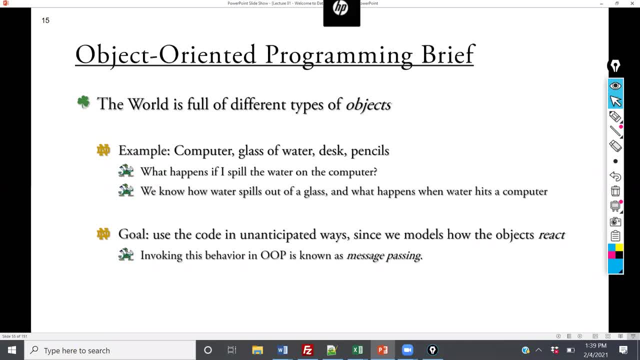 So that's one of the goals of object-oriented programming. to use the code in unanticipated ways and one of the reasons why we want to structure data in a specific way is to make those unanticipated ways work efficiently and reliably 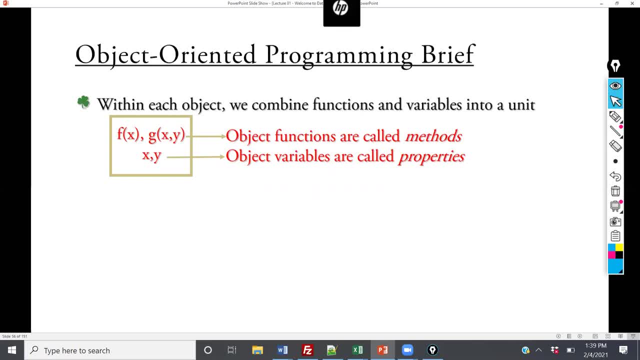 so here i have an encapsulation so object functions are known as methods and object value variables are known as properties i'm going to show you an example here in a moment 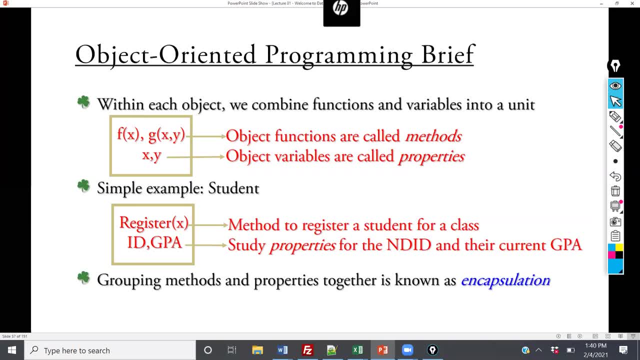 so as a student you have your notre dame id you have your name and you have a gpa these are all properties within a class and i want to have methods that operate on them 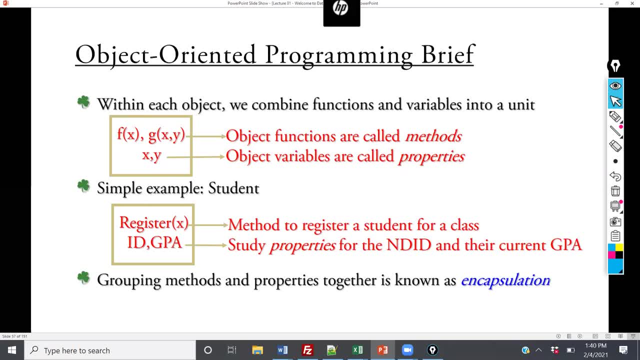 so for example register register i want to put in some sort of inputs and that checks to see whether or not you can register for a class so for example those of you who want to move to monday's 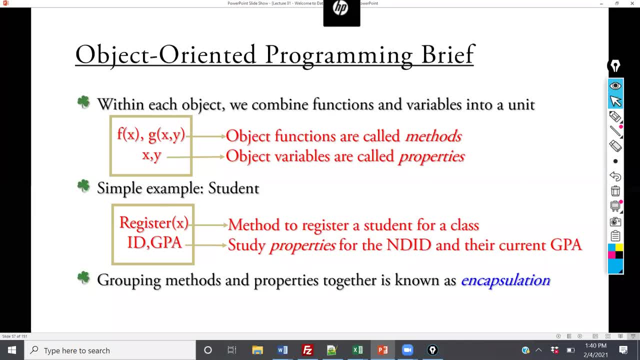 lab one of the things that you might want to do is check to make sure you're not registered for another class or we have to check to make sure that it's not full 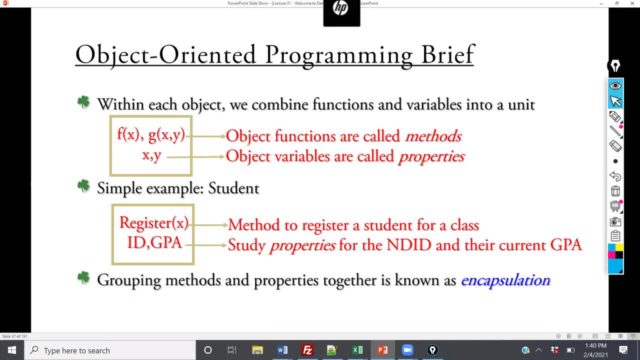 that's the type of method that can be operated upon a class student and then we have these private numbers or properties so that way when we access the class so for example let's say 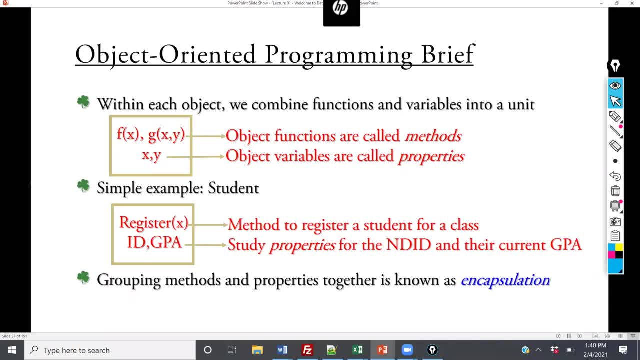 one of the properties is social security number you need to have that in there but only needs to be accessed at certain times not everybody who's accessing the program needs to have 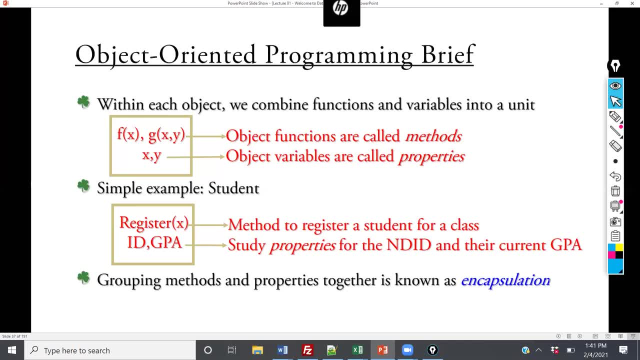 a public number on their social security number so the only reason everybody would have that is to know your social security number there's no good reason for me to know your social security number so therefore there should be no program that i can run or code that would allow me to 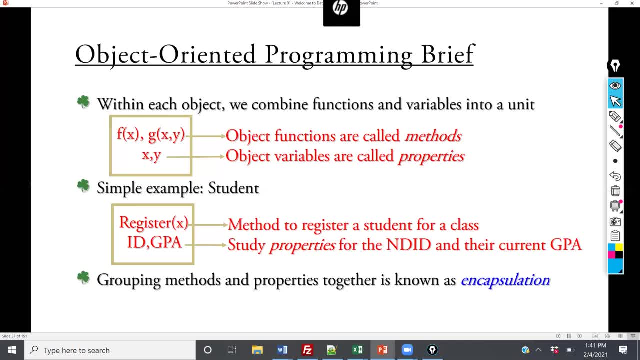 access it so that is this idea of encapsulation does anybody have any questions before i go on 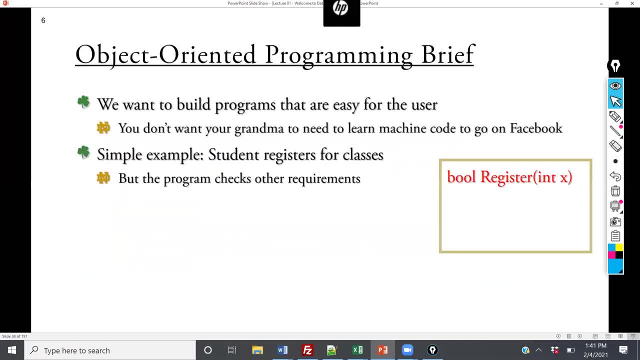 abstract abstract abstract okay so so 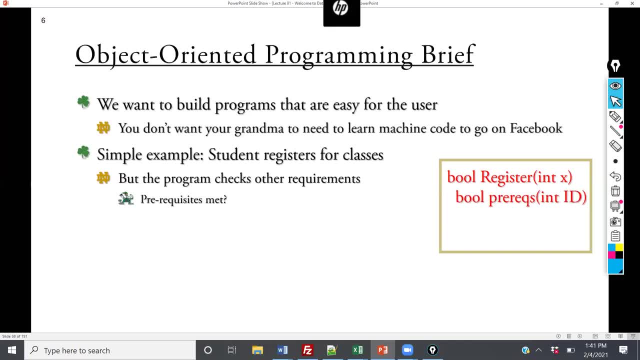 programs that are easy for the user, but we want to check other requirements. I think actually now we have other methods that we're going to say are private methods. So when I say this abstraction, you would put in a specific class that you want to register for. You want to register for this new section six for the lab. There's certain things that need to be checked and we don't, you know, we have to check to see if you meet the prerequisites for the course. Have you passed fundamentals of computing? The thing is, you don't, when you're using the code, you want 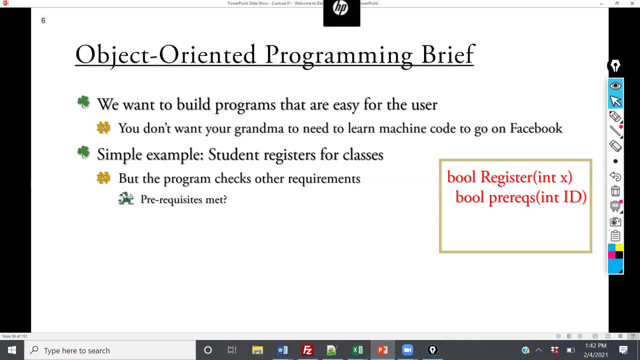 to have to click through everything. Okay, have you done this? Yes. Have you done this? Yes, right? 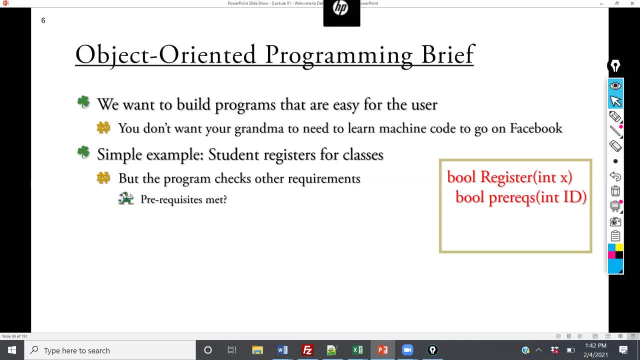 That's obnoxious. A well-written program abstracts unnecessary details away from the program. 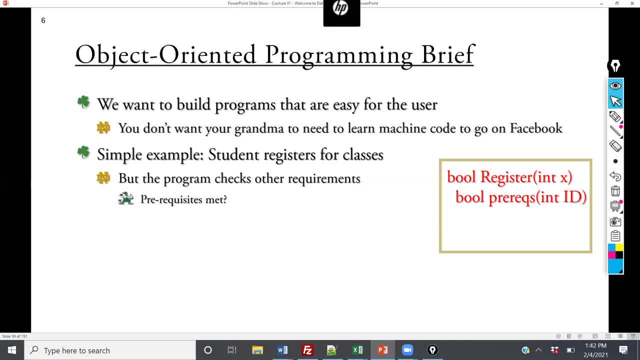 So when I say have I met the prerequisites, it can check the student properties to see if you've met the employees. And we're going to have a method there that's private. Number of seats. Are there seats available in that class? And credit overload. If there's a limit on the number of credits you can take in a semester, are you exceeding it? So for example, let's say you unintentionally exceed it if you're in section five and you're somehow registered for both. You'll say, wait a minute, you can't do that because you're now at 21 credits or whatever it is. So that would remind you to get out of one section before going back into another. 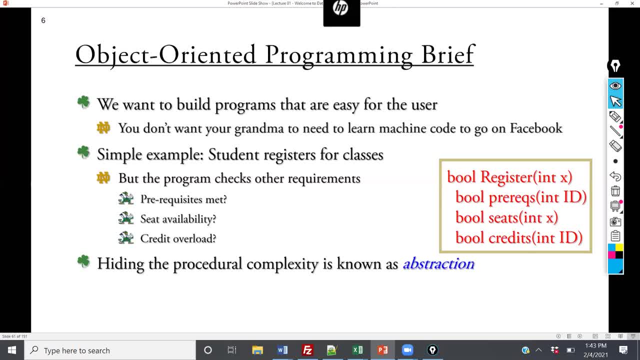 And hiding this procedural complexity, away from the program, is known as abstraction. This is a very important aspect of data structure. 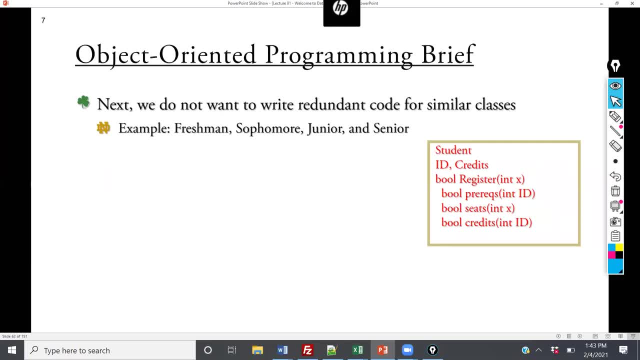 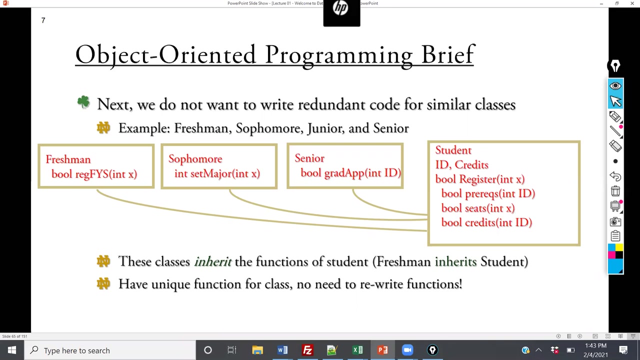 So for registration, there's different types of registration for different classes, for freshmen, sophomore, juniors, and seniors. You could actually have a class sophomore that inherits fundamental properties from students, but makes different methods for a specific sophomore. So for example, freshmen, you have to register for the first year of studies. Sophomores, you have to register for the first year of studies. Seniors, you set your major. And then senior, you can apply to graduate. So these are different things, but build off of the same fundamental class student. So you inherit 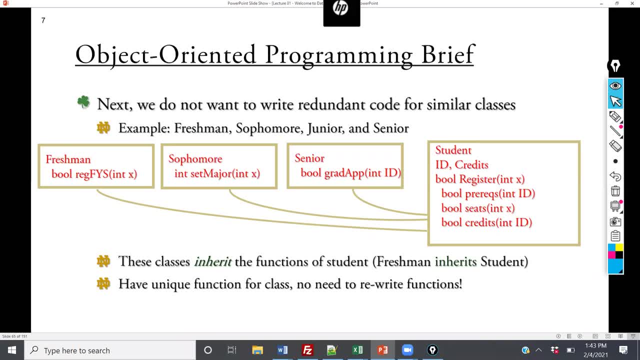 those fundamental properties, but then you can build upon those. And that is known as inheritance. 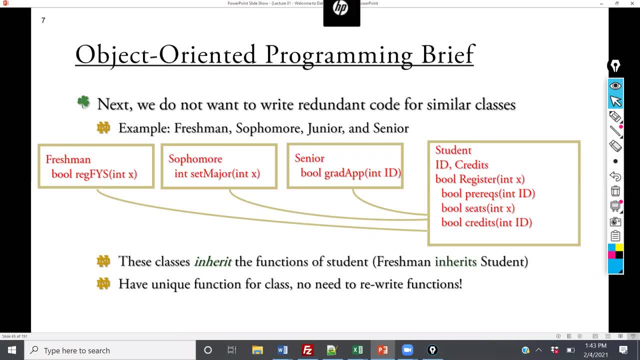 And we're going to see several examples of a data structure that actually inherits from a different data structure. We're going to learn about different types of hash tables. We're going to learn about AVL, trees. We're going to learn about splay trees. And the objective there is to say, well, I've already written all that previous code. If I can, in everything that I need there, I need this for this other program. Instead of just rewriting or copying all this code tediously, I can say that this class inherits that class, and then I'll make modifications based on it. So the objective that you should take from that is how to avoid doing redundant, unnecessary work. 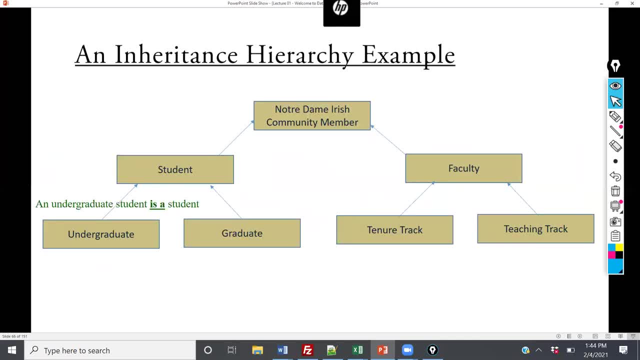 And so here's a, I've kind of alluded to this, but here's an animation to show you. So an undergraduate student is a student. And a student is a member of the Notre Dame community. 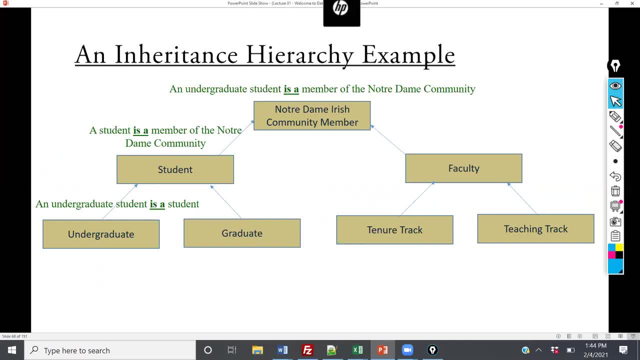 And an under, so therefore, an undergraduate student is a member of the Notre Dame community. And when we go over inheritance, I'm going to talk about, there's a reason I have is a highlighted, because you're going to go into a lot of detail about is a. 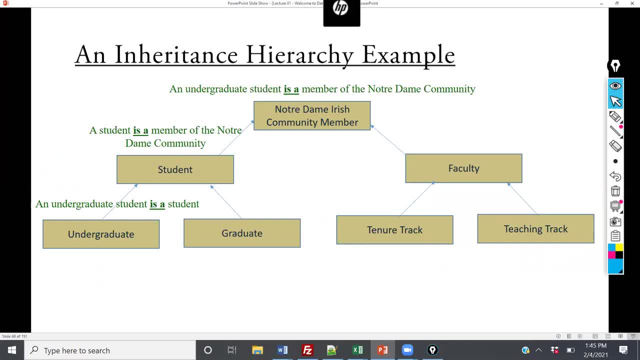 Professor is a member of the Notre Dame community. A student is a member of the Notre Dame community. A student is not living in Dillon Hall. 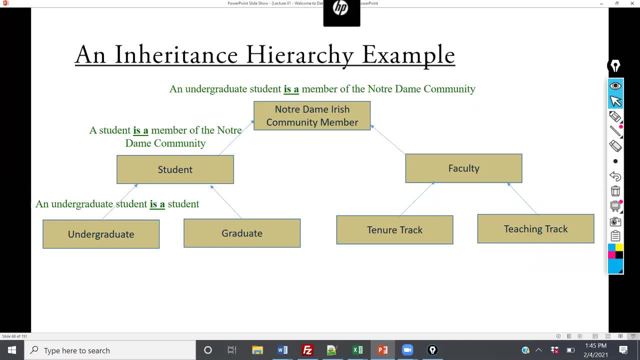 These are how you can separate what should be and should not be done in inheritance. 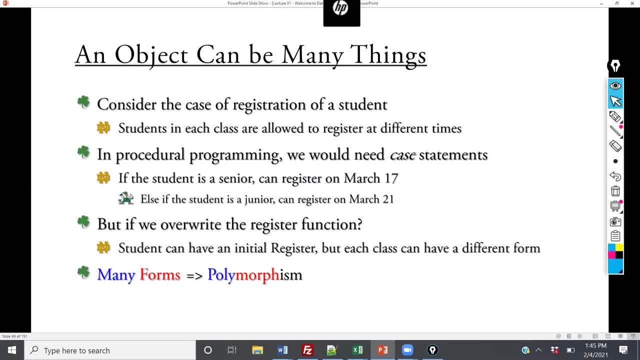 I want to check to see if anybody has any questions before I quickly review polymorphism. 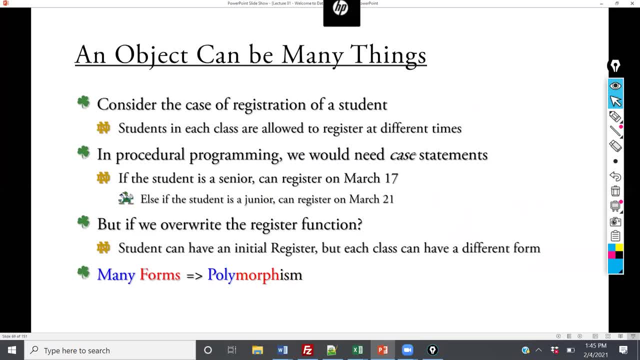 All right, so polymorphism, you can say, you can have a different version of the same method. So for example, let's say that I have, I say I have four classes, freshmen, sophomore, juniors, and seniors, and all of them have a method register. 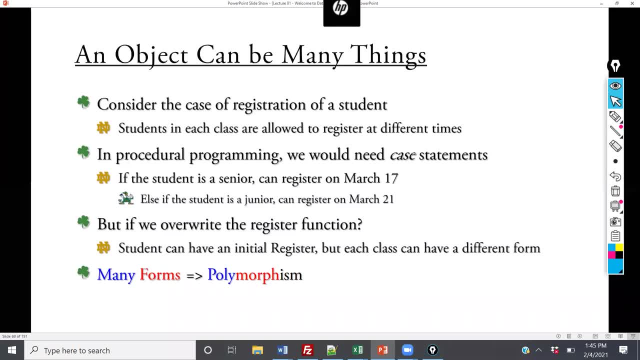 You want to register for classes. But we want to have them, have the student be able to register at different times. 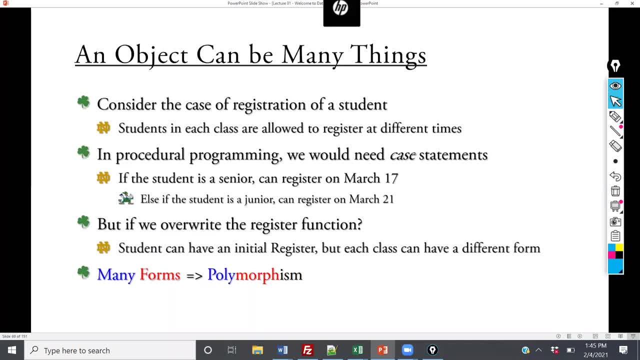 So freshmen, sophomores, juniors, and seniors can register on different days. We don't want a freshman to be able to register at a senior time. So what we can do is we can write a different version of register, in the senior class, the sophomore class, the junior class, and the freshman class. So that way we want them to do exactly what we want, and make sure that the students can register at the appropriate time. 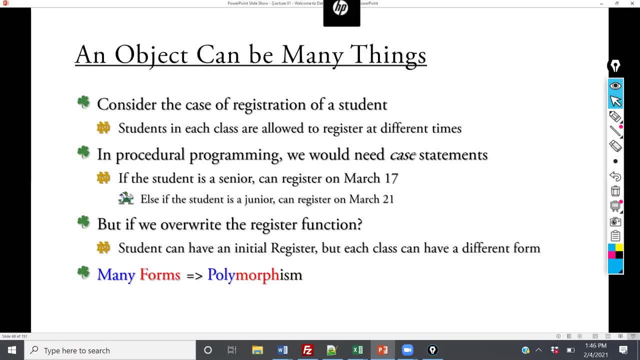 So we have the same method, but it has different forms in different inherited classes. 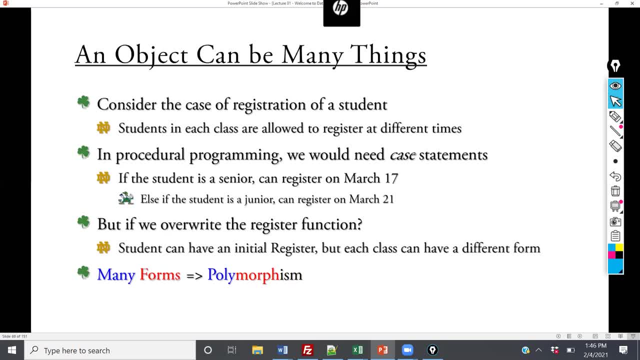 So that polymorphism, that's Greek, in English, that stands for many forms. 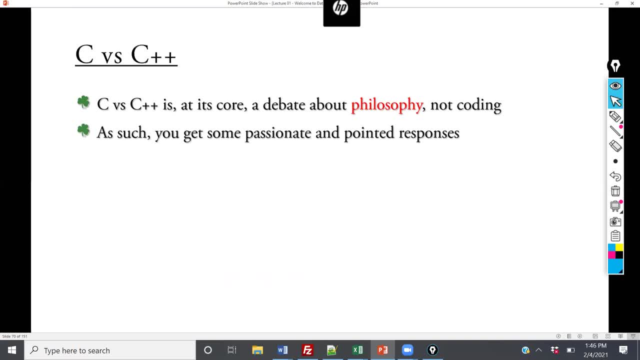 A quick note about C and C++. So it's C++ or C, depending on which one you think is better. It's more of a debate of philosophy, not coding. 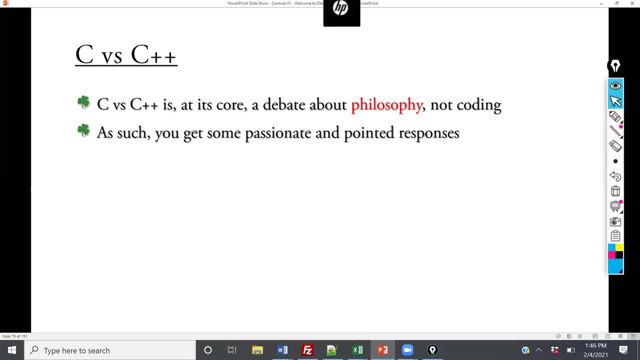 As such, you get some passionate and quoted responses about which one is better. So I've included some quotes from some of the main contributors. 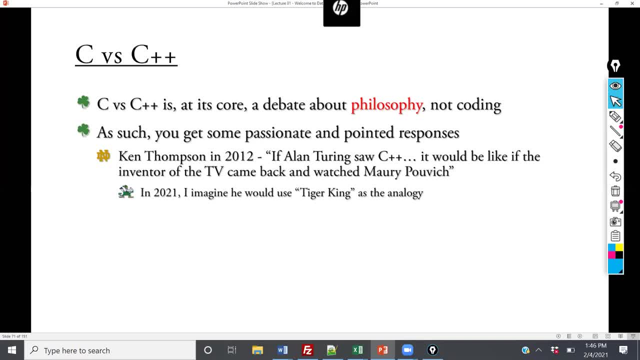 So Ken Thompson was a fundamental contributor to C and the Unix operating language, and he didn't like C++ very much. he said, 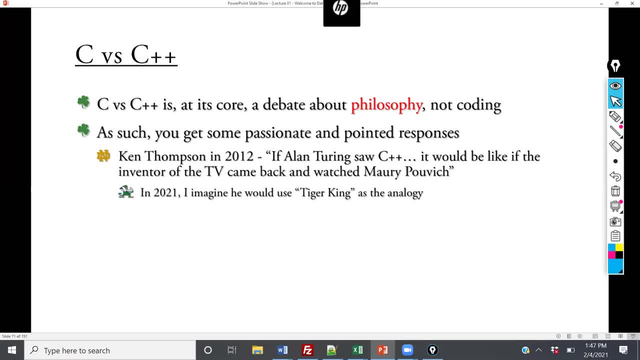 If Alan Turing, who was the inventor of the modern gaming device, He said, 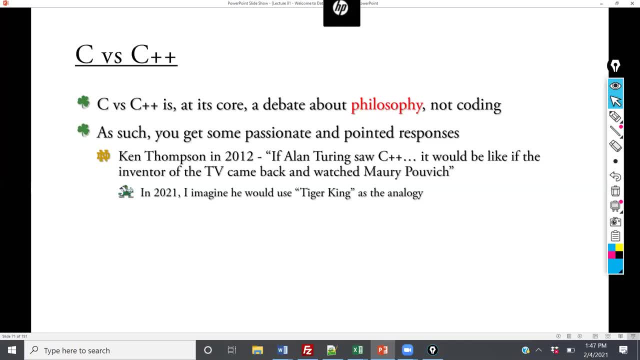 If Alan Turing saw C++, it would be like if the inventor of the TV came back and watched Maury Kovach. 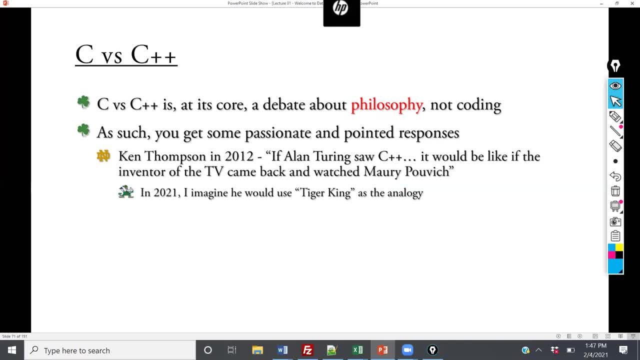 He's a you-are-not-the-father guy. So the modern analogy in 2021 would be if the inventor of the TV came back alive 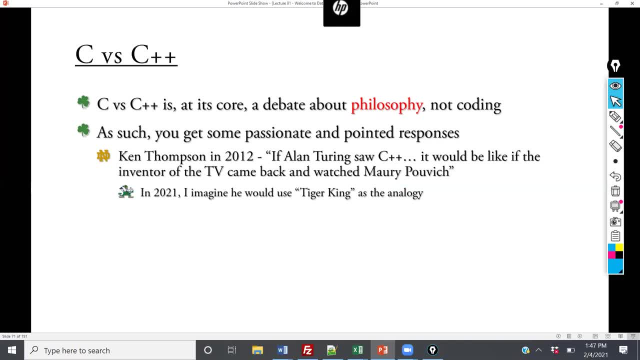 and saw Tiger King and saw Carole Baskin acting the cool one on television, right? I like that. 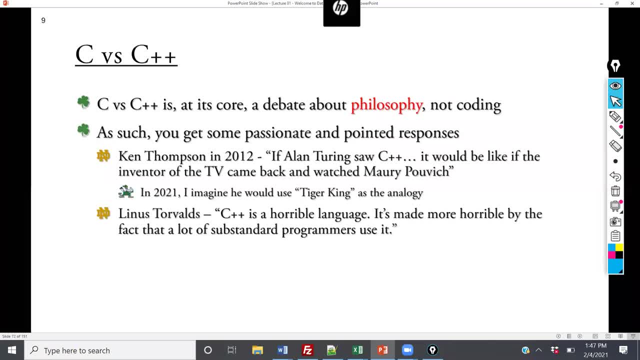 Furthermore, if Linus Torvalds, who invented Linux, he just straight up says C++ is a horrible language. 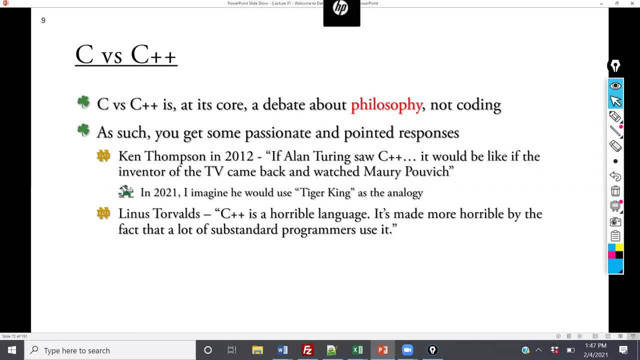 It's made more horrible by the fact that a lot of substandard programmers use it. So then, Bjarne Strauss-Strupp comes back. 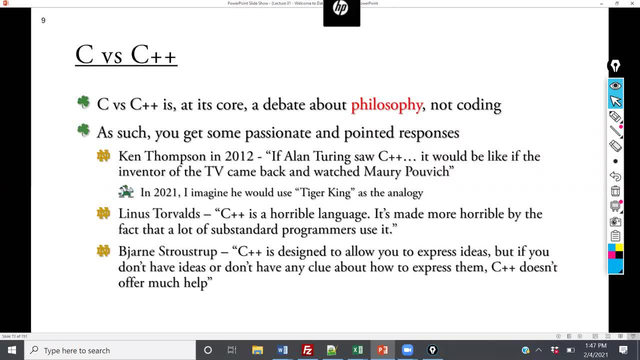 He claps back, so to speak, and he says, C++ is designed to allow you to express ideas. But if you don't have ideas or don't have a clue about how to express them, C++ doesn't offer much help. 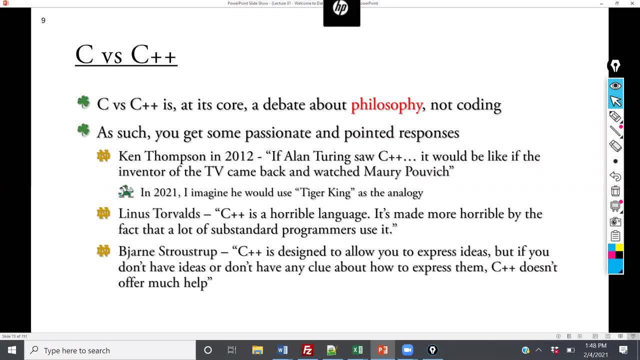 So in that debate, there's a lot of shade going on between them, right? 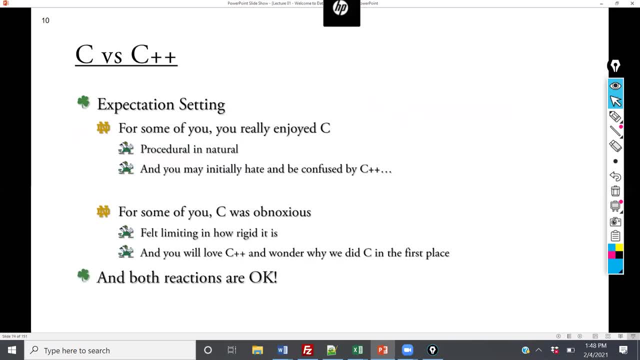 So why do I mention C++? You know, we're teaching this class in C++. 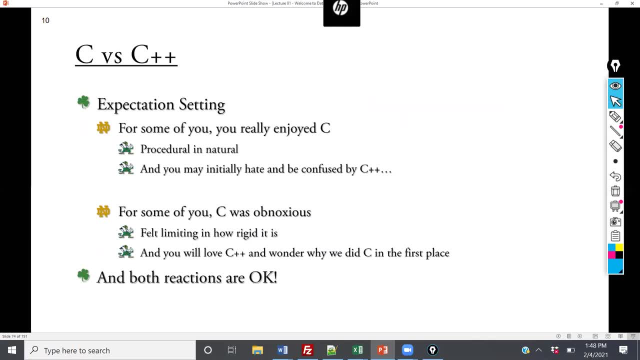 And why would I come up with C++? It's a substandard programming language. A lot of substandard programmers use it. 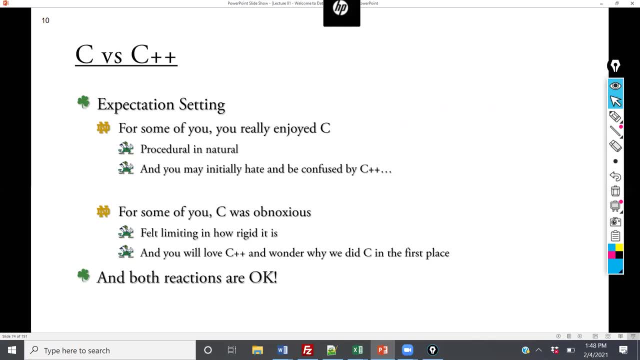 It's involved in my class, right? We don't want to do things like that. We want to set some good expectations. 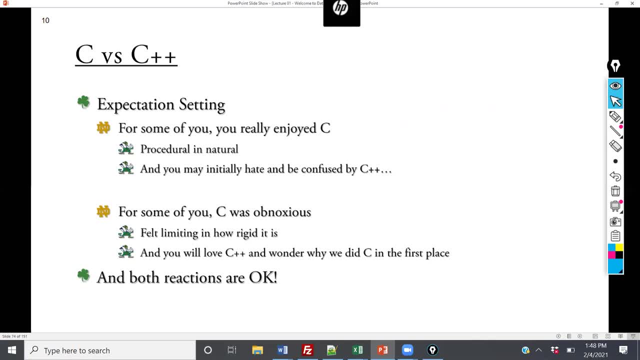 Some of you will have really enjoyed C because procedural is natural to you. For some of you, that was ideologically limited. But at C++, it's the other way around. C++ is like, oh, why can't this just do it in a way that I'm not going to do it? It's something I'm thinking. 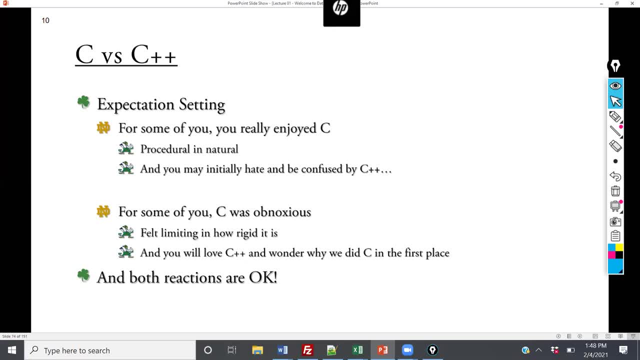 And then you start coding and C++ will make a lot more sense, too. And both of those reactions are okay. 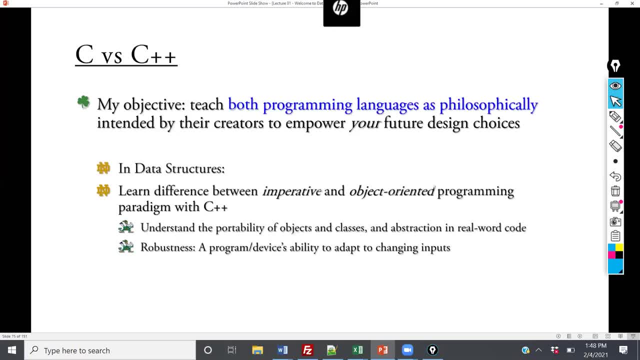 You can still be an outstanding programmer. There's no reason for us to bicker like Linus Torvalds or Bjarne Stroustrup. 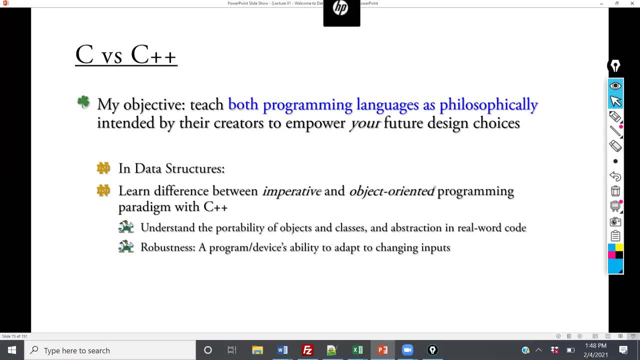 The big thing about programming language is an understanding the procedural versus object-oriented programming language. Because if you understand what's going on underneath a hook, if you understand how the data is structured, if you understand how to construct it, 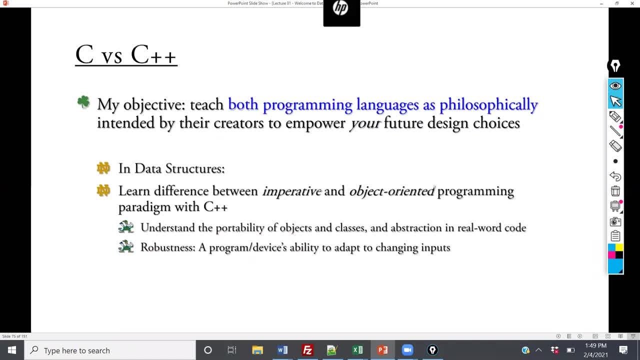 it efficiently and reliably in a way that progresses efficiently through the machine then you will be able to be outstanding at implementing the object oriented programming 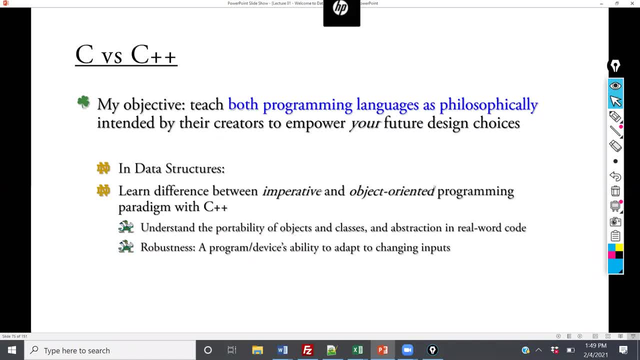 so the part about linus torvald saying substandard programmers i i don't know about you but i don't expect any substandard programmers from notre dame right my father went here so i know that you know like well dr morrison you didn't that's right i didn't but um but the crucial thing is if you understand both you'll be able to uh do really well so understanding the portability of objects 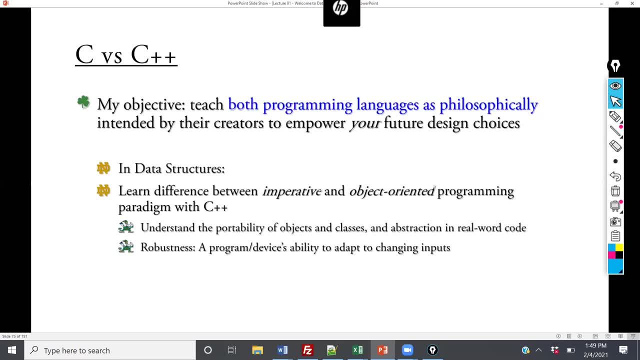 and classes and abstraction in real world code and robustness of programs devices ability to adapt to 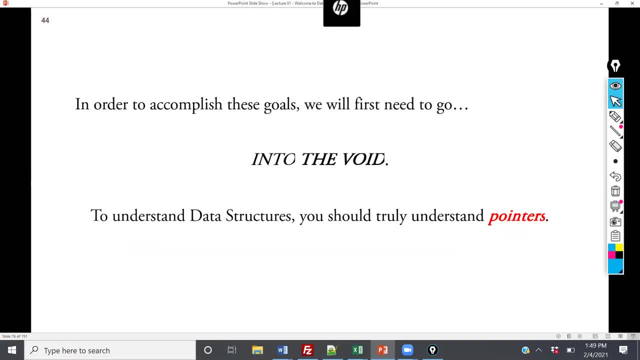 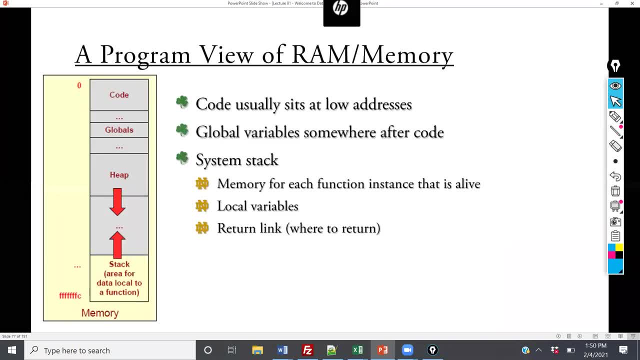 bit in number so let me quickly go over ram memory so in ram you have the code itself you have global variables which you've learned about and then you have functions and as you call more functions especially when you do things like recursion you'll see that um as it goes on it takes more memory so the we're we store what's known as dynamic memory when you build a dynamic array or for those of you who coded in c calic and mallet you can allocate the memory after the program has become running you will implement that on the data heap and the system stack is where you start storing these functions and eventually you have return when you type in return zero what that also does is it has it go back to the previous location where you made the function 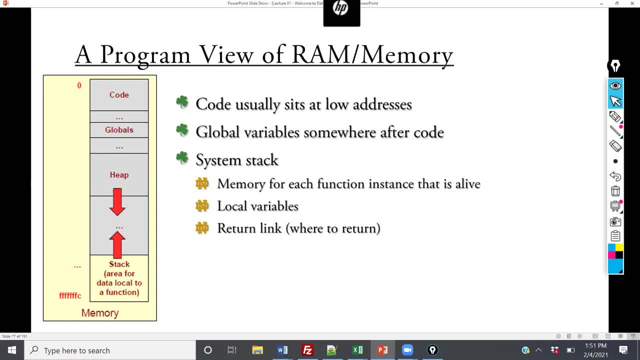 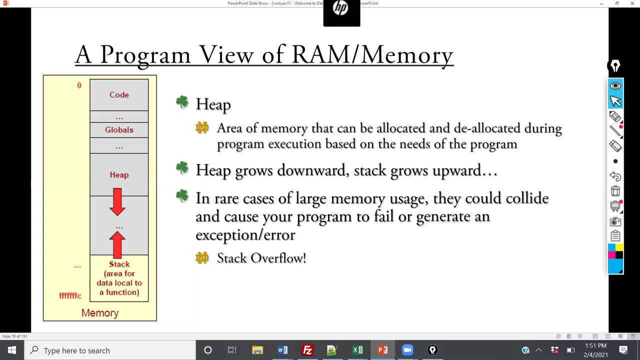 and so this is a general idea of ram and what i want to show you next is how this is broken down so heap is the area of memory as i've alluded to that can be allocated 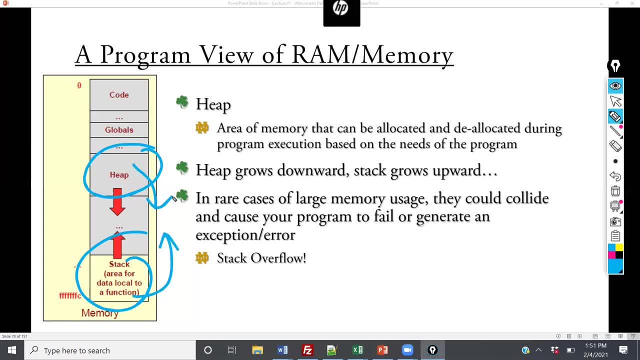 and then the stack with the function calls so you have dynamic memory they grow closer to each other and if you overflow you have too much of it that's what a stack overflow actually is so that's why we want to be 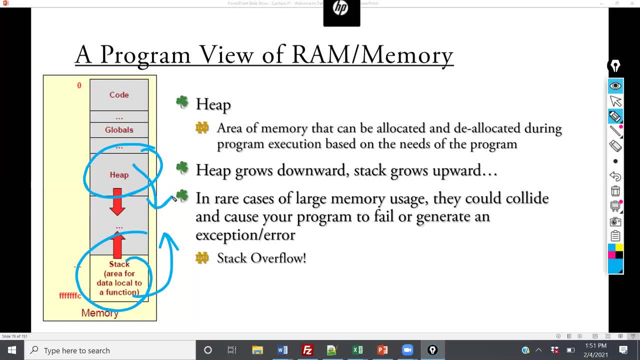 efficient and reliable with memory and data structures so we don't have any stack overlords 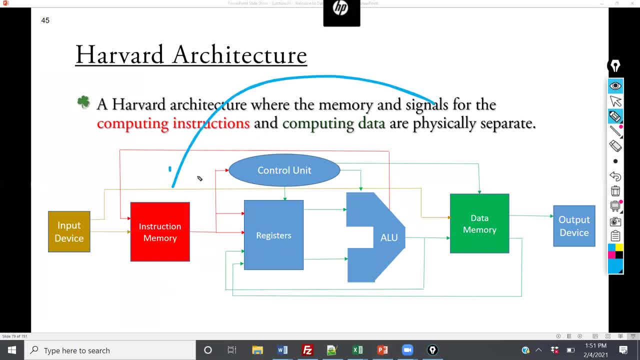 so one thing that you'll notice in the harvard architecture is that we've split up the instruction memory and the data memory and the objective there is to separate the stack and the heap and try to have certain amount of memory allocated 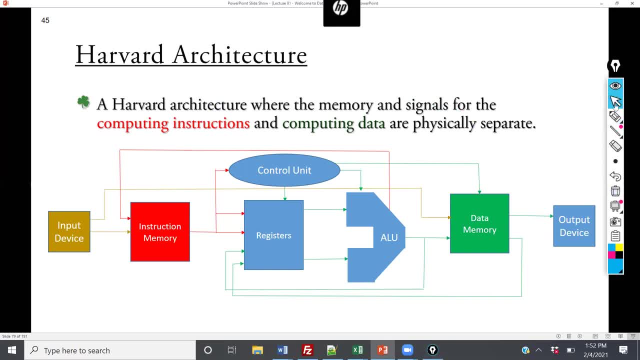 for each of them to try to offset some of these stack reflections so i say computing instructions and computing data are separate you know that a lot 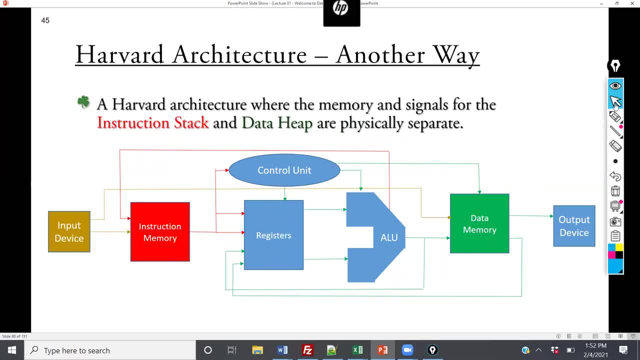 more detail about the architecture but i can say the same thing by saying the instruction stack and the data is more physically secure aaron thank you girl all right so then the 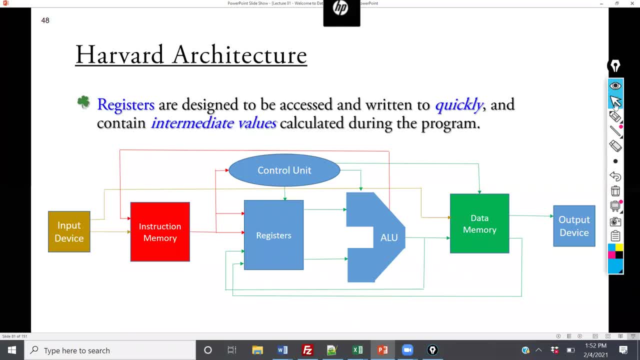 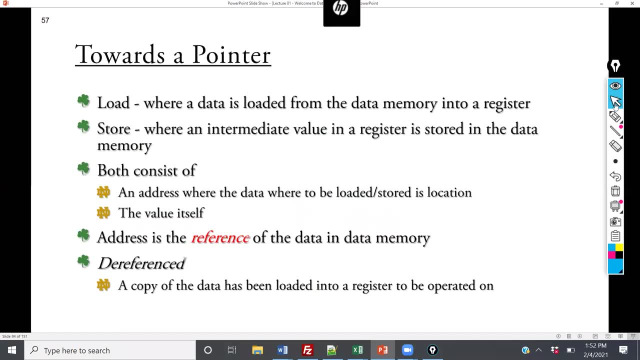 registers are fast they're kind of alluded to this already um let me skip past that i've told you all that already mode and store is how we get stuff from the instruction stack 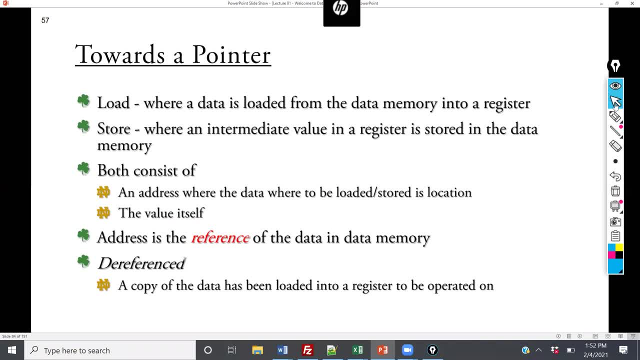 and the data key taking advantage of the register. And the register contains the address of a location on the data key. 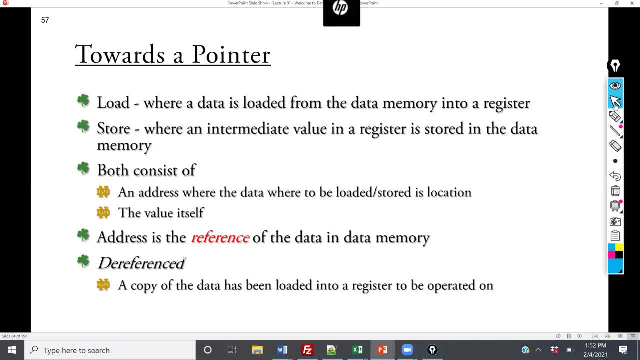 So that's what a pointer actually is. It tells me where something actually is. 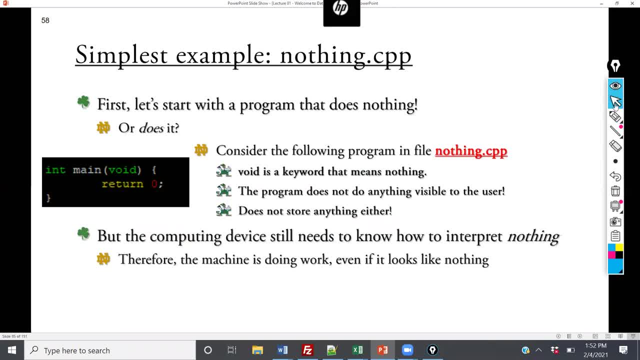 And so what's going on here, let's take a look at a very simple piece of code, nothing.cpp. It has int main and just returns zero. 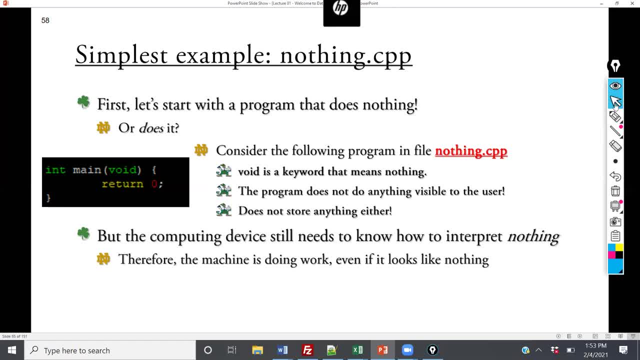 And void means that I'm taking in nothing from the input device. 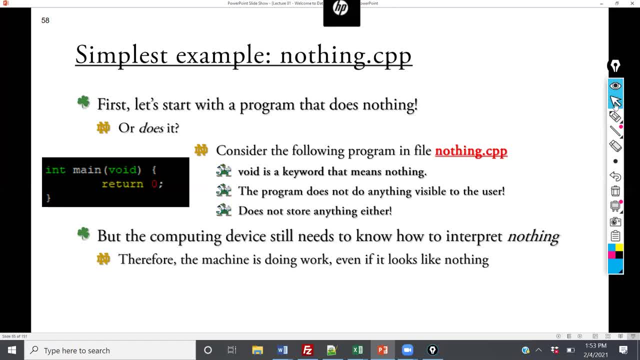 But it's important to note that there's actually more going on underneath the hood when we talk about these different levels of abstraction. So let me walk through this real quick. 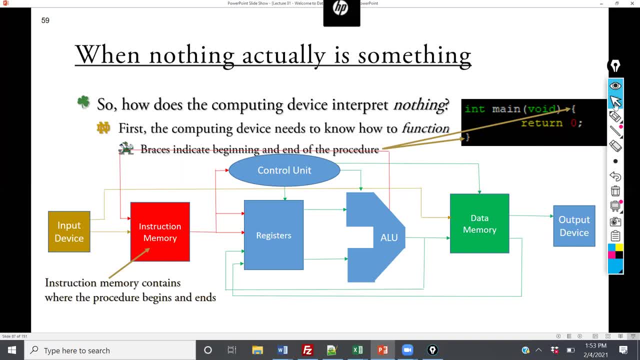 The braces in C and C++ indicate the beginning of a procedural operation. It's actually a location in the instruction memory that says, all right, this is gonna, the program starts here, we do certain tasks, and then it ends here. 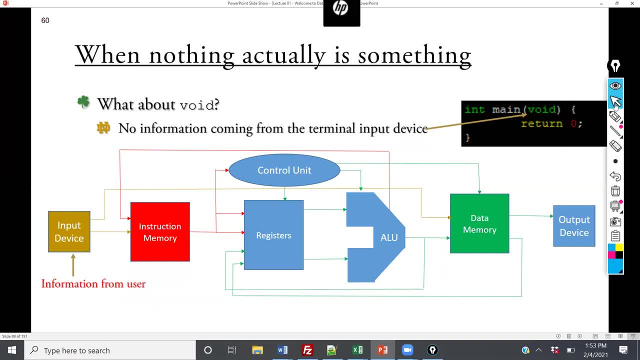 Next, void means we're not taking anything in from any input device. 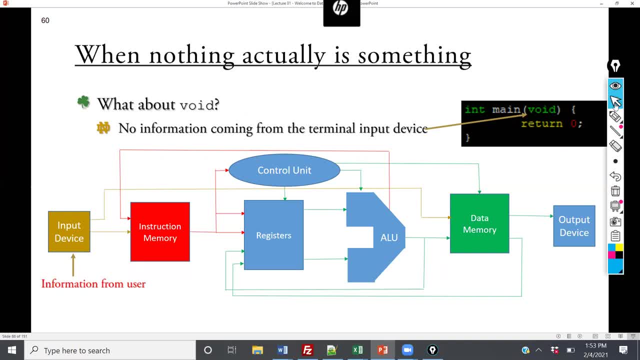 We're not needing anything from the terminal. It's not going to be available anywhere on the computer. 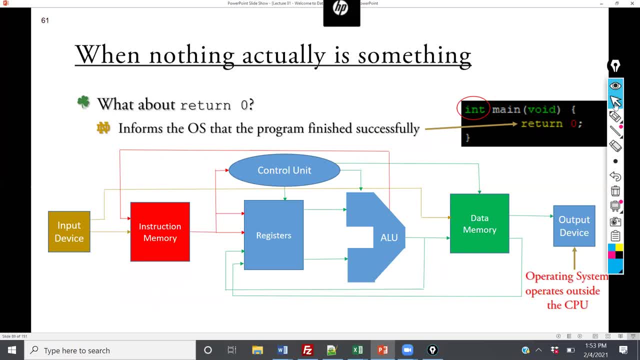 Then return zero tells us that we send an integer value to the operating system to indicate that we have successfully completed the program. 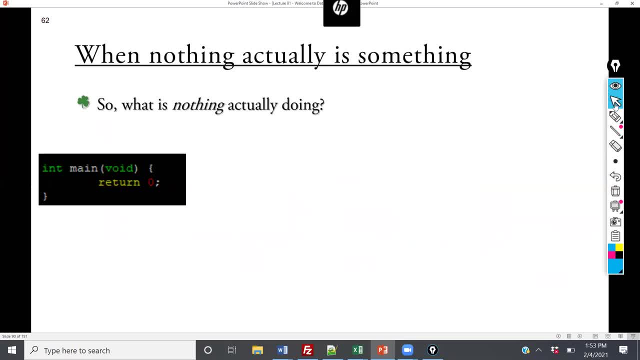 So walking through this, what is nothing actually doing? It's actually doing something. 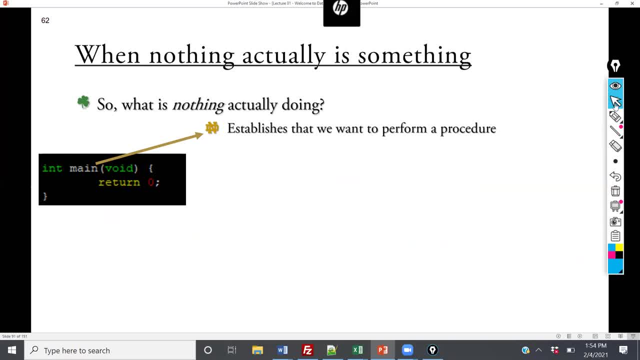 We indicate that we want to perform a procedure, and we're gonna put that on the instruction stack. Then we're not gonna get anything from the input device. 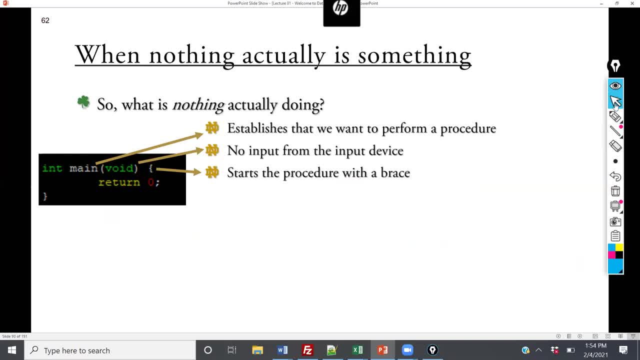 Then we're gonna start the program with this first brace. Then we inform the operating system that we're done successfully. 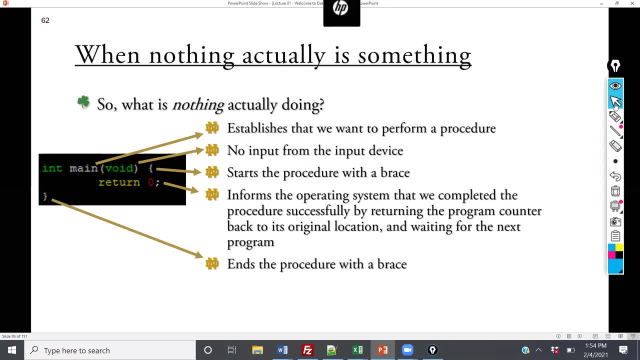 And then the last part, the final brace, is in the instruction, and it's in the, in case that we have completed the program. 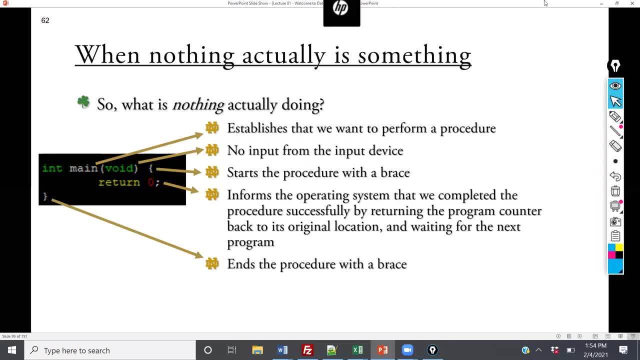 I'll quickly check the chat as well and see. Okay. 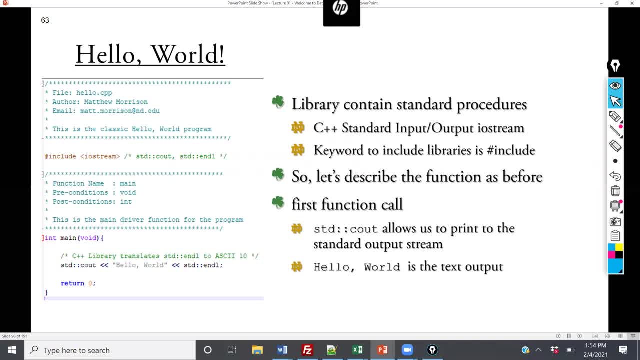 So now let's go into a little more detail. We're gonna do hello world. So it's the same program that I've been showing you before. I've described that what it's doing is allocating memory on the data so you can access it. So let's walk through with the same kind of thought process that I just did with nothing.cpp and see what's actually going on underneath the hood. 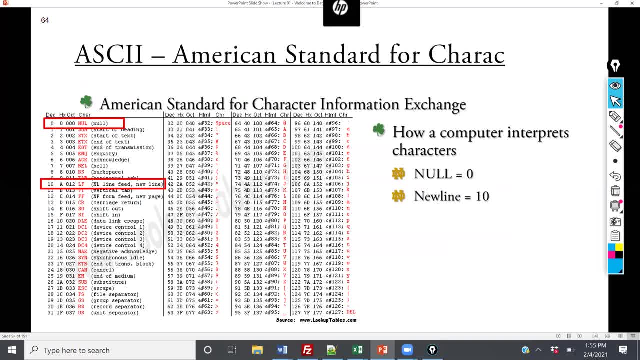 So each character, is what's known as an ASCII value. 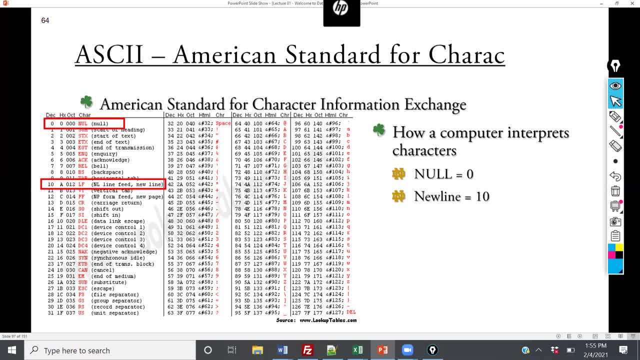 ASCII is an 8-bit representation of a character. And these are all the values, if you go to ASCIItable.com, it actually has all of these. 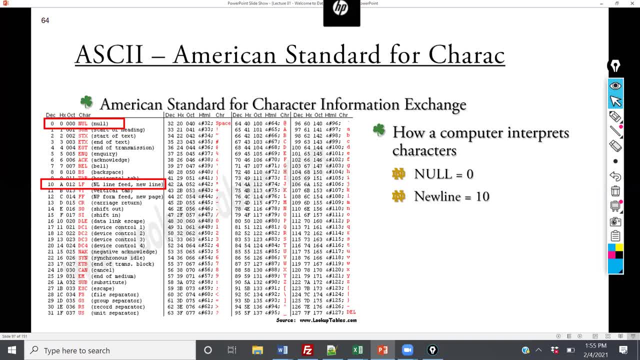 But zero means null. 10 is a new line character. So you did slash n, you're actually sending an 8-bit value with the number 10 in it, so 1010. 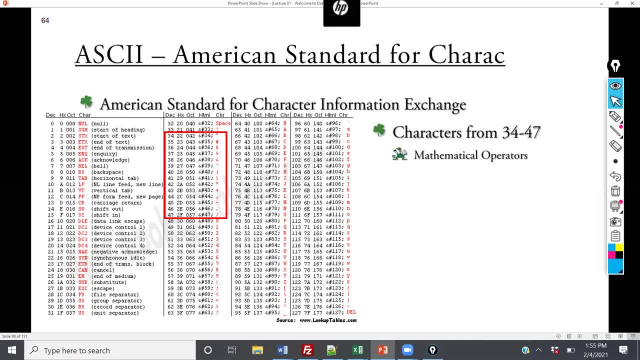 34 through 47 represents several mathematical options. 34 through 47 represents several mathematical options. 34 through 47 represents several mathematical options. 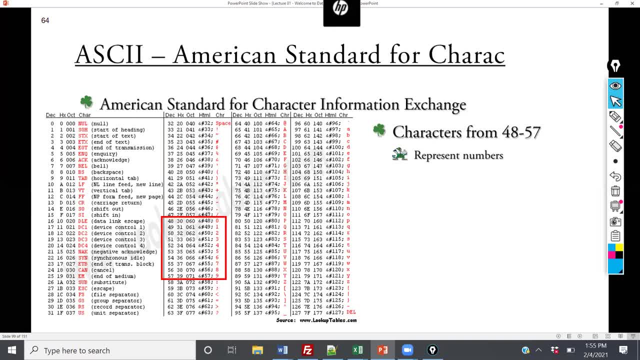 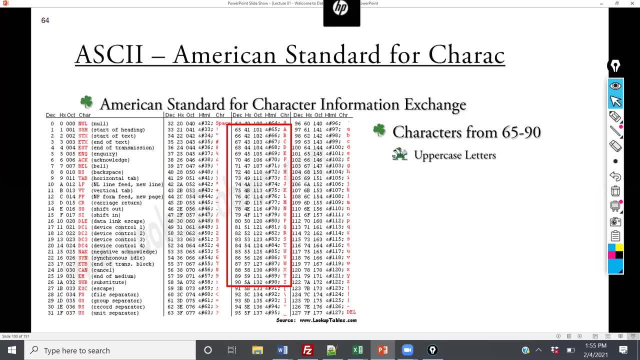 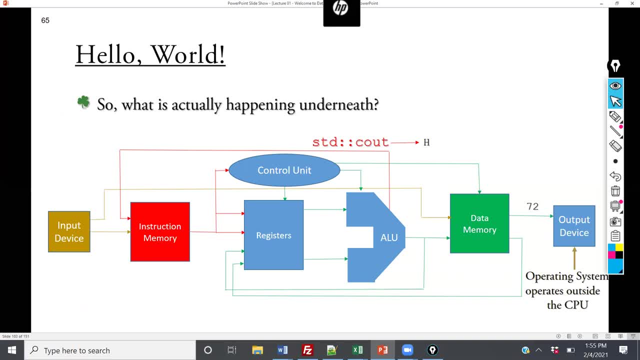 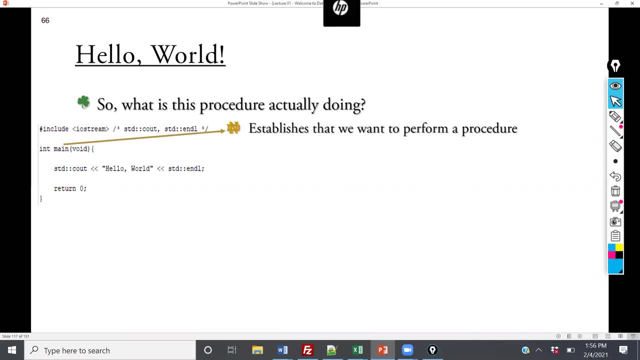 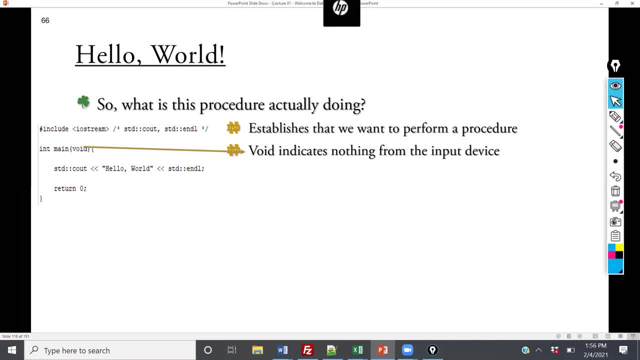 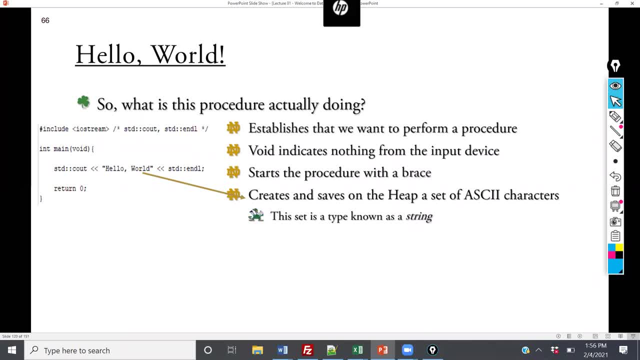 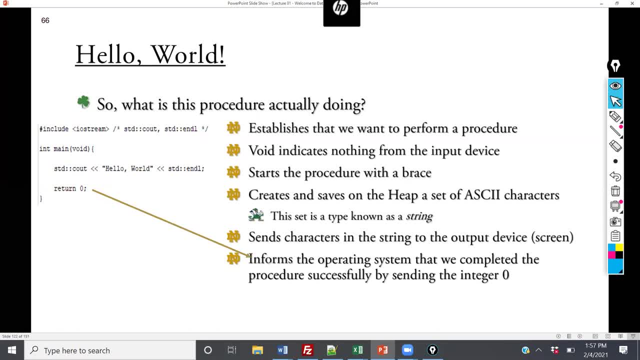 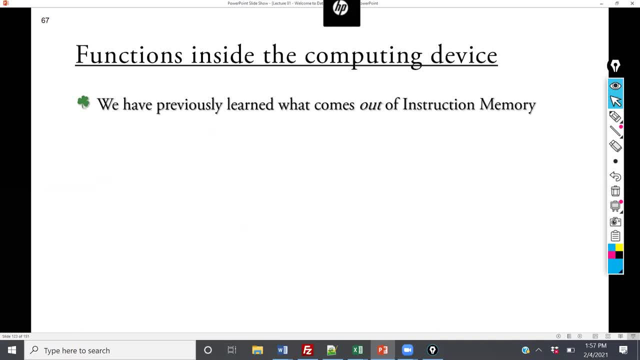 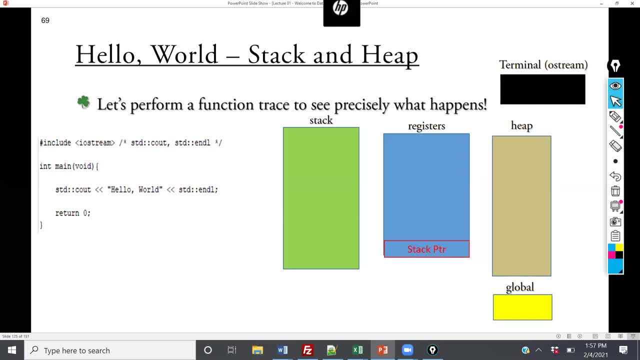 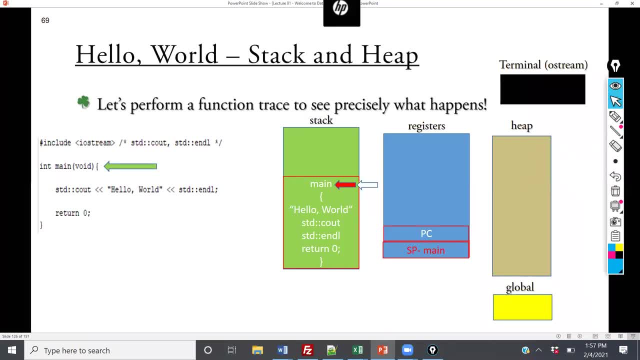 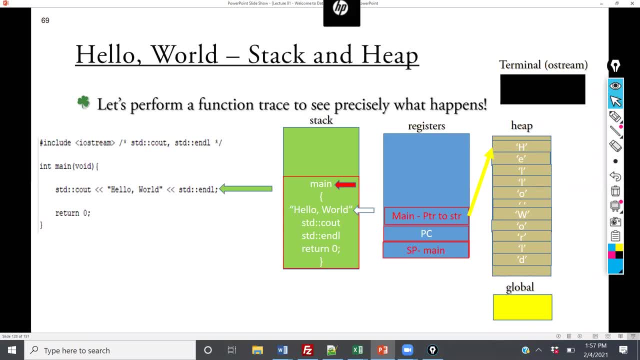